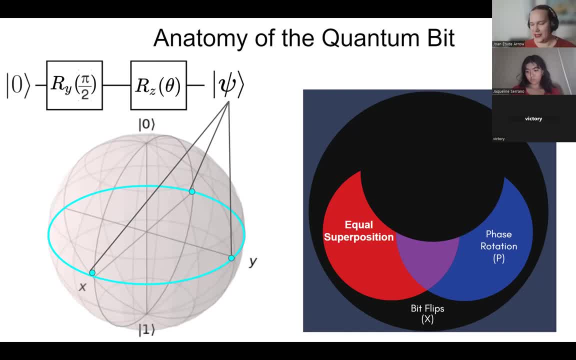 feature of quantum computers- And the hand wavy argument that you've been talking about is that you might hear- is that quantum computers use these phases. think of waves when they're in or out of phase, like a noise canceling headphones job. a wave comes in and it generates a wave in the 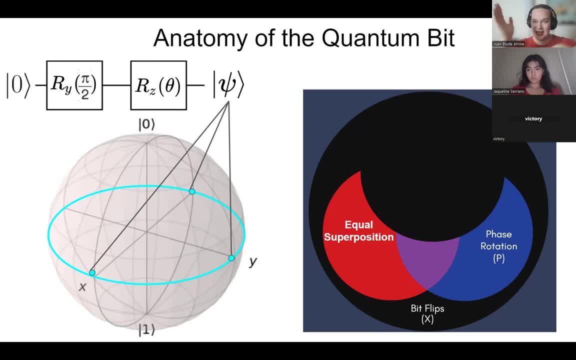 opposite phase. So that would be 180 degrees rotation to cancel the incoming wave, So you don't hear any sound. A quantum computer in a similar way choreographs that interference between quantum states of different phase to try and produce a solution that has probability of. 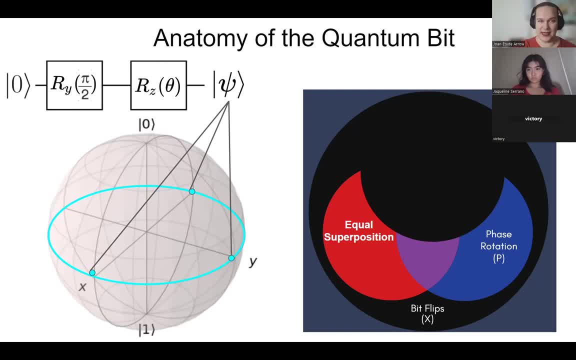 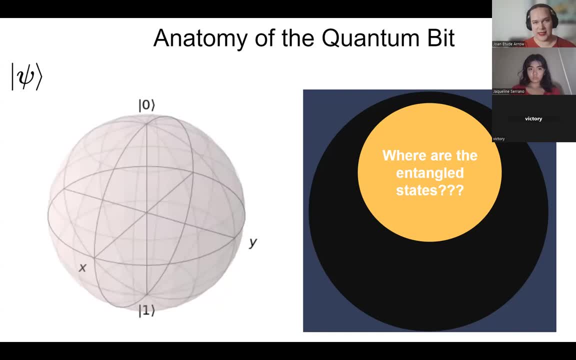 being measured and spitting out the quote unquote solution to the problem. That's a hand wavy answer. It's not really the whole picture, But that's just one way you can think of it going forward. And we left with this kind of thought experiment of how do you make entanglement And we talked 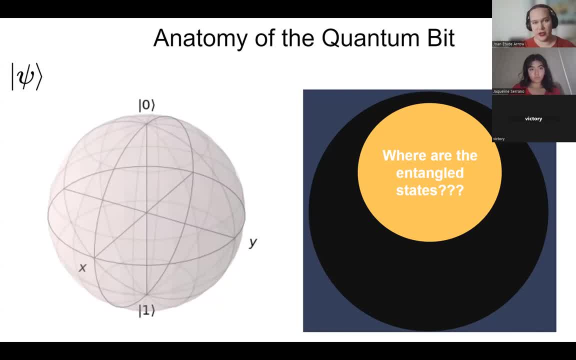 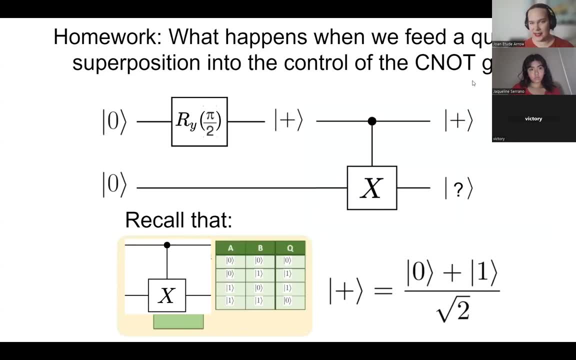 about how you can't actually make entanglement unless you have more than one qubit, And so we returned to this experiment that we had done, where we were previously running these bits and sending them through an XOR gate or or control, not where we remember. if the top qubit is a zero, you apply the bit flip gate to the 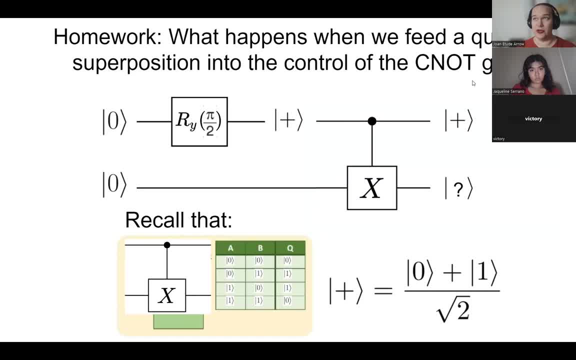 bottom register. Or, excuse me, if the top bit is zero, you do not apply it, If it's one, you do. And so the question is: well, that's all fine and dandy if you've got classical bits in the top. 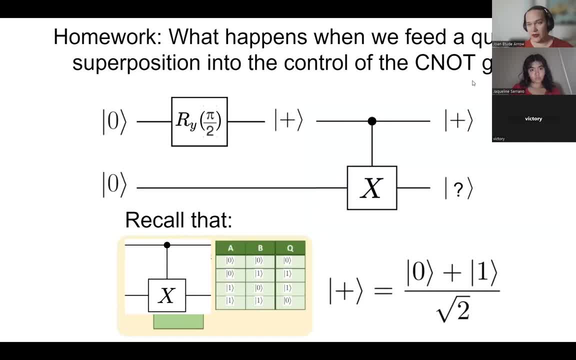 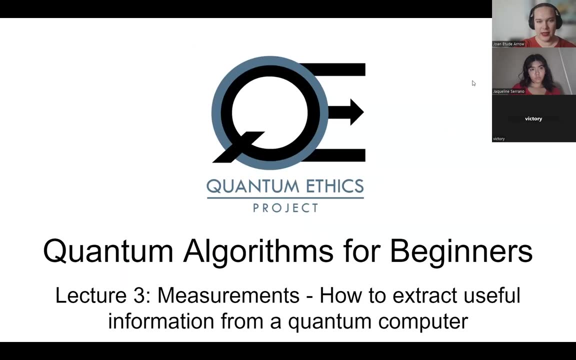 qubit. But what if that's a superposition? What if you set, if you, what if you apply a gate based on whatever state Schrodinger's cat happens To be in? what? what happens then? And so this is how we kind of want to motivate the, the value of. 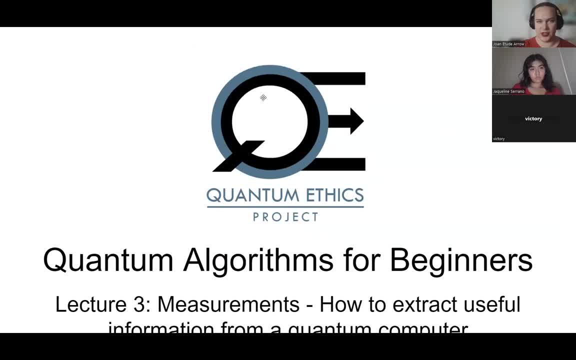 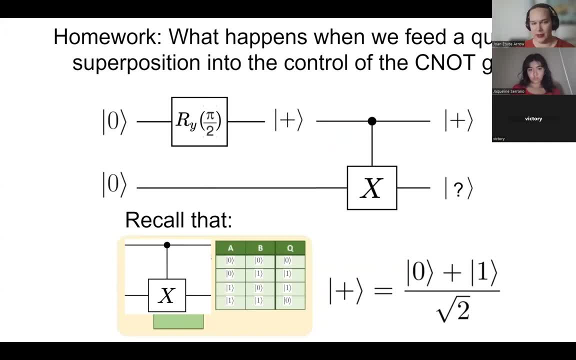 performing measurements, because we need the language of measurements in order to talk about. you know what happens with this setup. the setup generates the famous bell pair. these are the canonical example of an entangled pair of qubits. So what ends up happening at the end of this is: 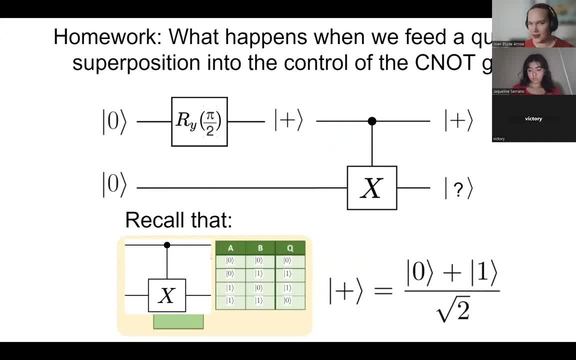 that you want to think of. well, so you're in this quant posit, you're in the state of quantum uncertainty. the top qubit was uncertain as to whether it was a one or a zero, And because of that it kind of 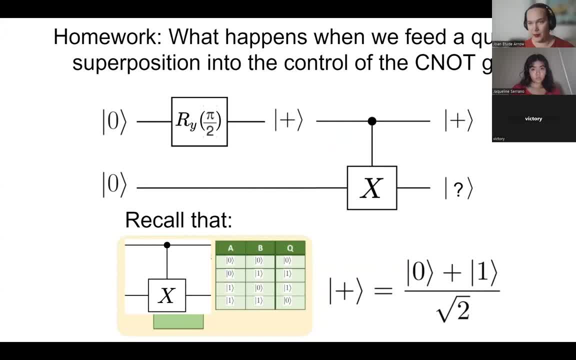 spread its uncertainty to the bottom register. So now that bottom qubit- well, I don't know what state it's in. it might be zero or it might be one. And because of the quantum nature of these things we actually can think of, we can now think of these two states as being connected. 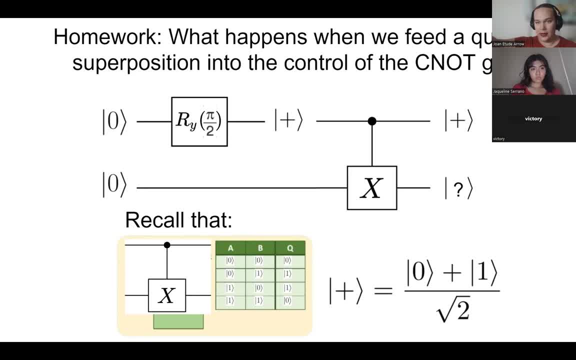 If I look at the bottom qubit and I'm not sure what state it's in. I'm not sure what state it's in. if I look at the top qubit and I see a zero, then the bottom qubit will be a zero. But if I look at 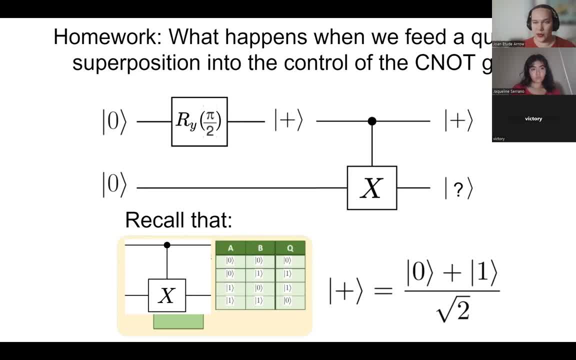 the top qubit and I see a one, then the bottom qubit will be one. The rough way to think about it that I like to use is: quantum doesn't break the laws of logic. Like you're not going to see, 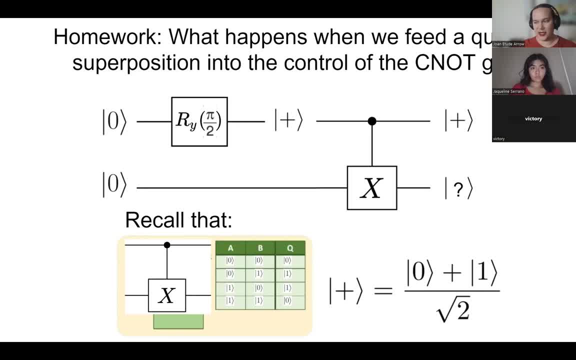 a quantum state measured in one place that disagrees with what would have happened in another place. Like the agreement has to be in one place and it has to be in another place, It has to be there even if there's still uncertainty after the circuit has been run. 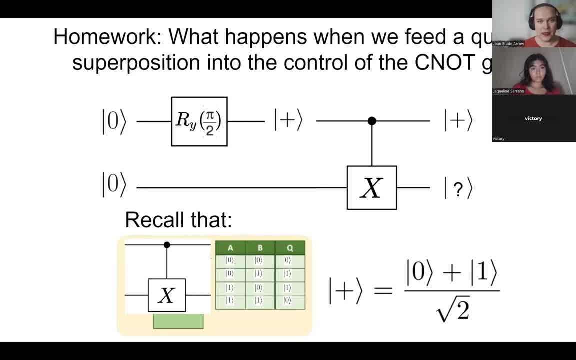 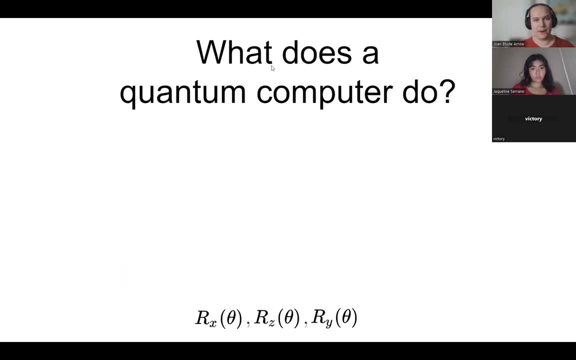 which is maybe a little convoluted, But the bottom line is we need measurements to talk about. you know what this bell pair looks like, And so that's where how I'm trying to motivate this third lecture here. So we started with this last time We talked about you know. 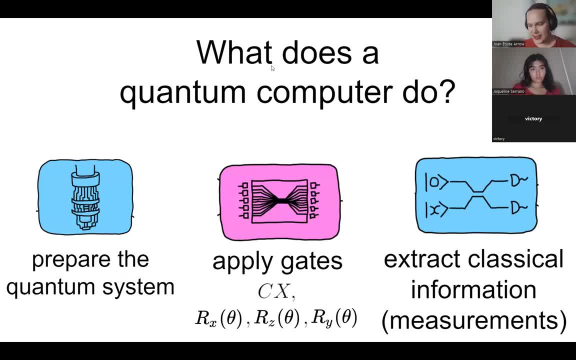 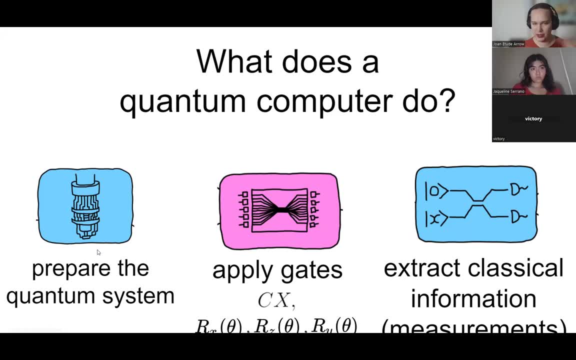 what does a quantum computer do? You know if you're sending a job to a physical quantum device that would be on the left-hand side? It would start off. it would prepare a quantum system, an array of quantum bits. It would start them off in some starting state. 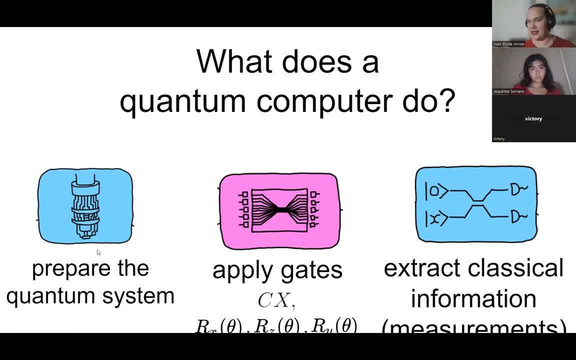 Usually quantum algorithm. people assume the starting state is everything is in the zero state. But that doesn't have to be the case. Then the algorithm side is you apply a bunch of gates. We've talked about the rotation gates, the X, Y and Z rotations, about various angles. 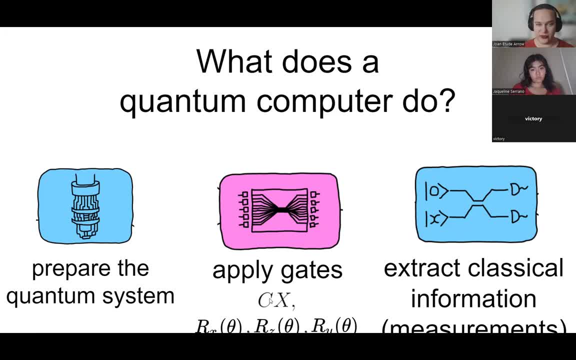 And we've talked about the control-not gate- that is helpful, as we've just seen, for generating entanglements Today we're going to focus on. so we've talked a little bit about those gates and I haven't told you too much about like useful circuits. 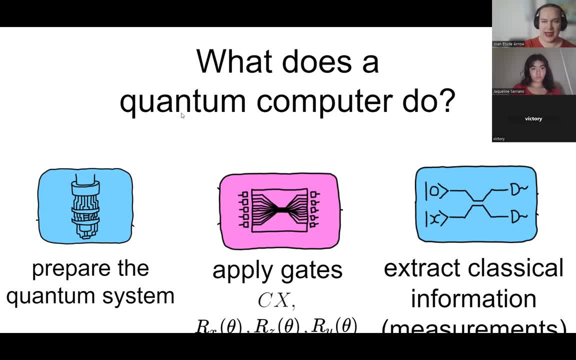 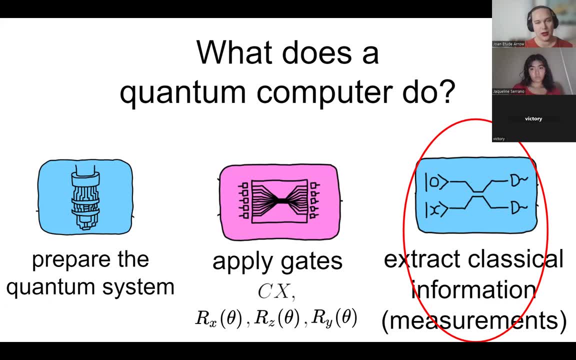 you can run with them yet. But today we're going to focus on how, at the end of the process, you can extract classical information from that whole system, Because the quantum computer can exist in states that we classically can't see, Like you can't physically see a. 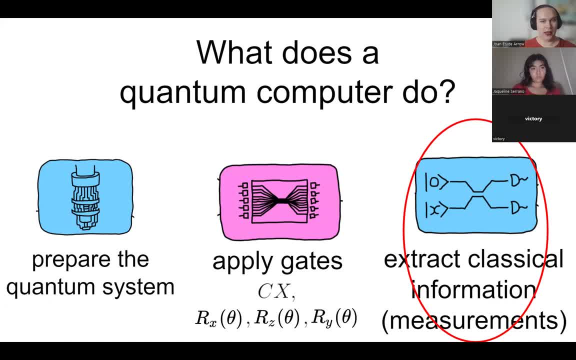 Schrodinger's Cat, both alive and dead at the same time. You can only see it as one or the other. So you can think of a quantum computer as being able to store information in this special quantum state, But you can only extract from that classical information. You can never actually. 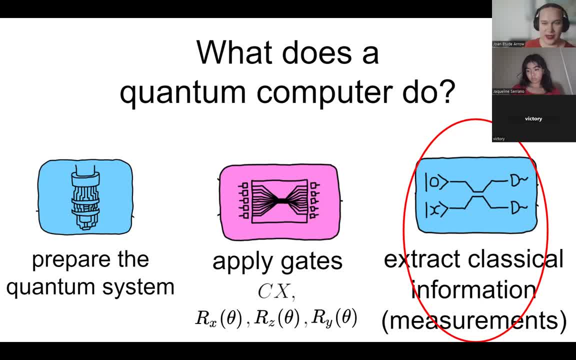 physically see the quantumness. The quantumness ends up realizing itself in the classical information that you read out of the device. So that's what I mean by a measurement. You measure those qubits, you measure those Schrodinger's cats and you see some configuration of ones, or 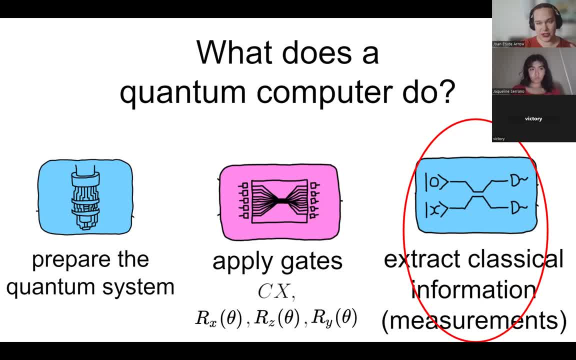 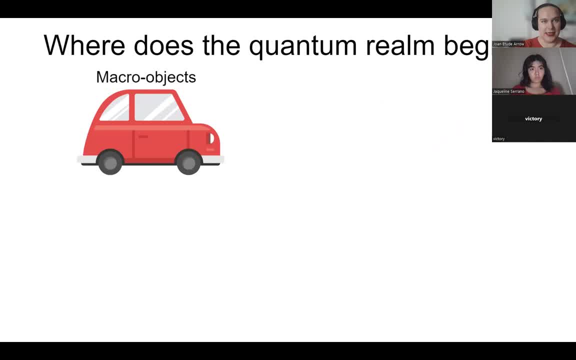 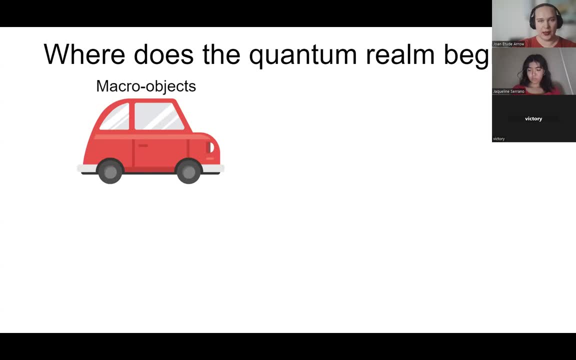 zeros And we want, at the end of the day, the computer to store the answer to a useful question into the value of those measurements And we want to talk about how that happens today. So we've talked a little bit about like there's something special that goes on in the quantum. 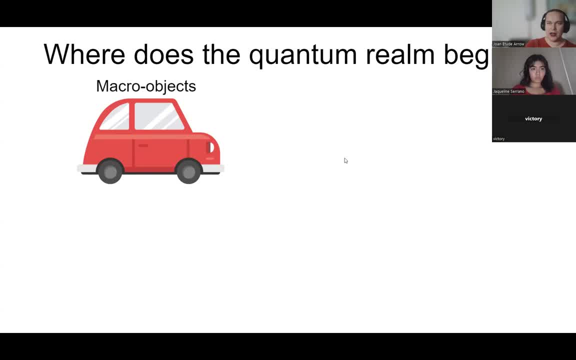 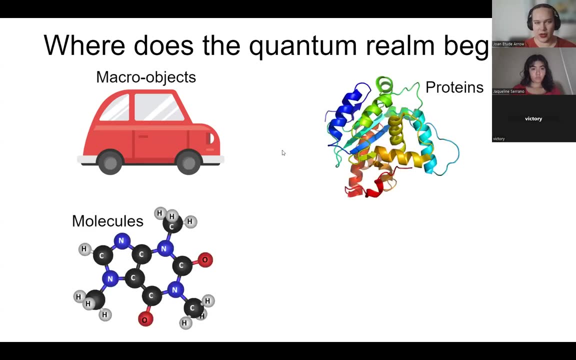 realm, You know, and the question is like where? where do things start acting like quantum projects? You know, you've got cars which I think nobody is going to assume your car can behave quantum mechanically. But the question might start to get blurry, You know. do you see quantum? 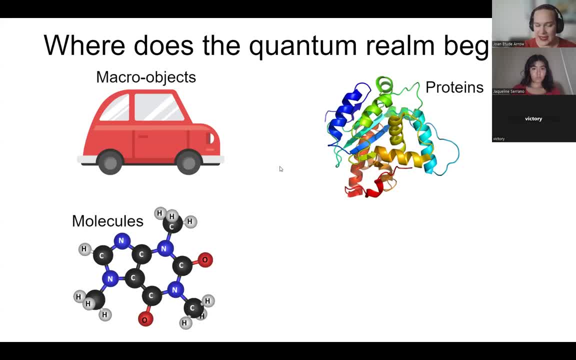 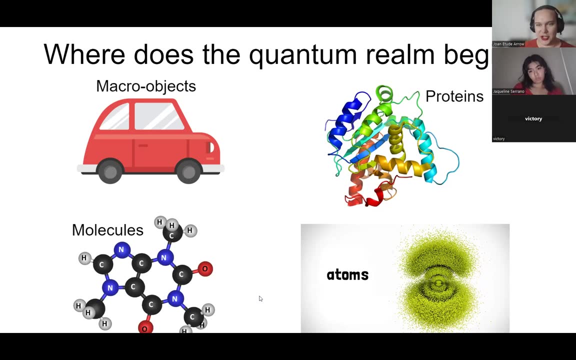 behavior at the level of proteins. Maybe more likely you see it at the level of molecules. I think probably. certainly we see it at the level of atoms And, by the way, on the bottom right that picture is is supposed to be a nice, more realistic representation of an atom than like. 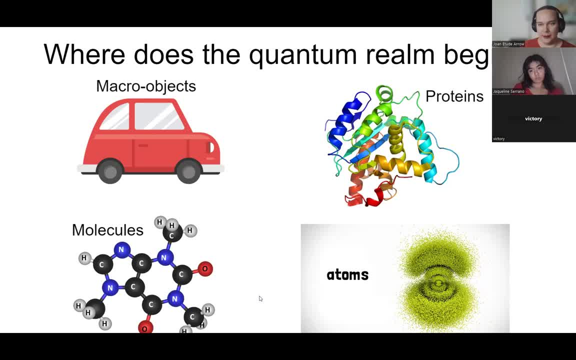 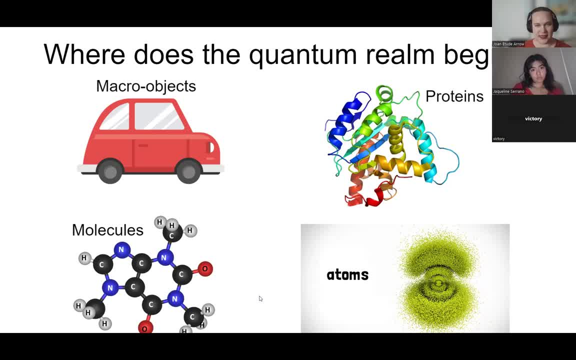 do you think we might need to pay attention to quantum effects? do we pay attention at the level of one of these four, like how big can you get in silty quantum? I think probably as big as macro objects. and explain why? just because quantum can be so like I'm trying to find a way to say it. 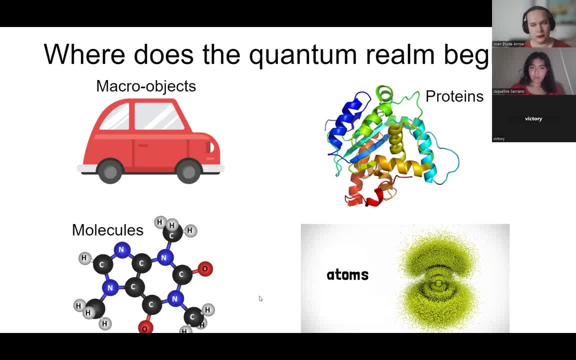 um, well, there's so much that goes into like quantum that I feel like it could be in objects as big as like cars. we can probably see like some quantum algorithms or behaviors and things like that. yeah, so I mean, I think and I I have, I've been. 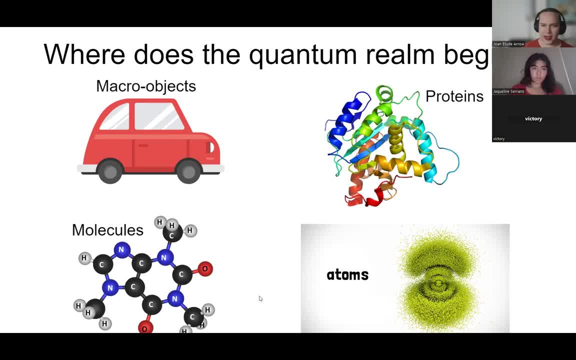 making, working on a lecture to talk about this. but um, have you ever been in an MRI machine? no, do you know what they are? they're like these big donut shaped things. they they can image soft tissue. those use quantum properties to visualize macroscopic tissues in in the human body. um, 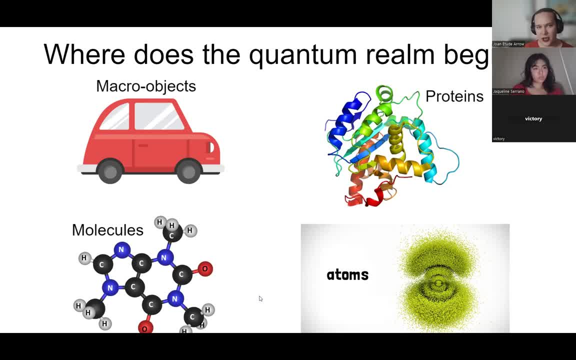 typically people, um, don't think of large-scale objects like cars as behaving quantumly, um, but you're right that these objects are made of quantum pieces. So, you know, in the case of humans, where we've got all these molecules inside of us, like in the bottom left corner, all these atoms, and those atoms are made of, you know, even smaller particles. 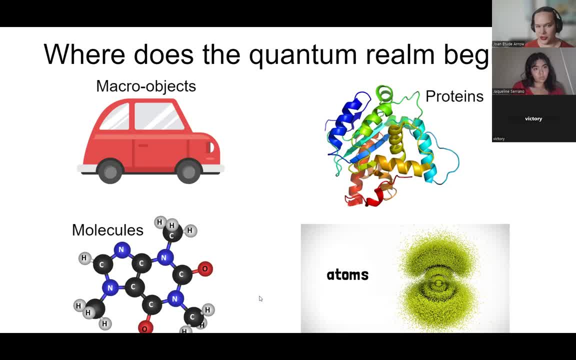 The MRI machine can register the magnetic field generated by, say, the nucleus of an atom inside of your body and that will be affected by the other atoms in the molecule that it's part of. And that's how MRI machines identify the different types of tissue. But for our purposes, I think you know, in the space of 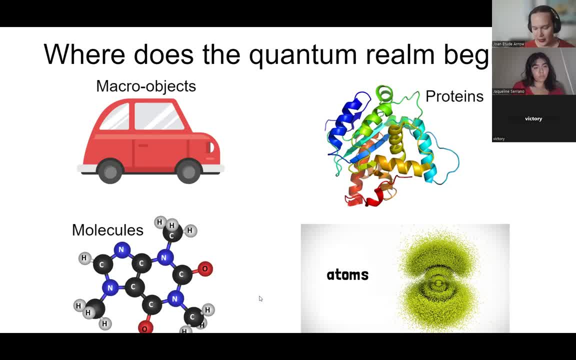 quantum chemistry, I think the largest we can go where quantum effects may be realized is on the scale of proteins, at least for this exercise. But you know, it's a philosophical question that actually is currently an open field of discussion where physicists, I think, don't have 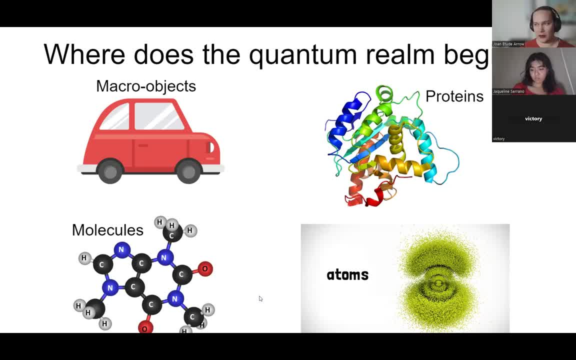 a haven't come to a full consensus on, you know, where the precise boundary between the quantum and classical world falls and why it might fall there rather than somewhere else. That's that's kind of a philosophy of quantum question. But for now we can think of atoms are certainly quantum. 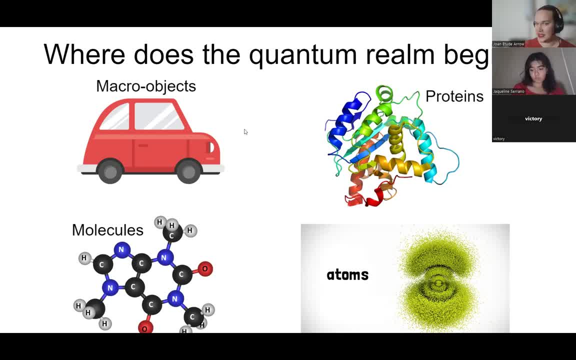 molecules, Absolutely. Proteins still, Yes, But starting to get large by the time you get to the size of a cell. it's controversial. You know, some people are trying to do research about whether cells interact via quantum effects. I know someone who's doing that at UCLA. but that's kind of getting a little bit further towards the. 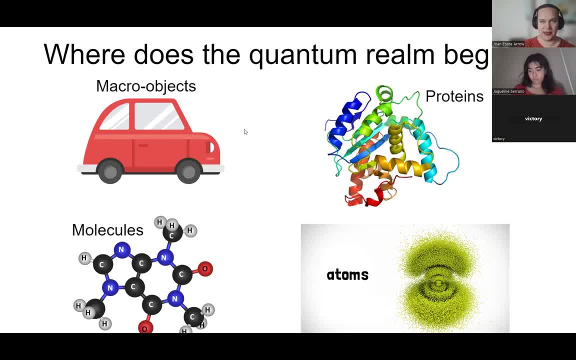 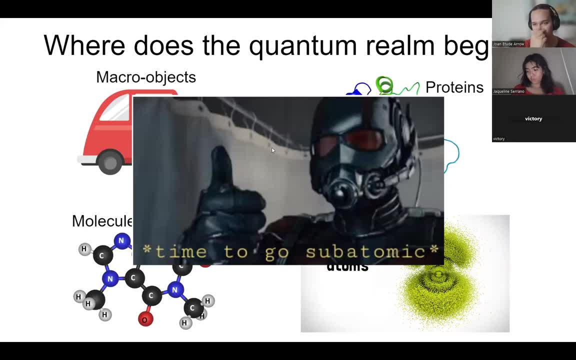 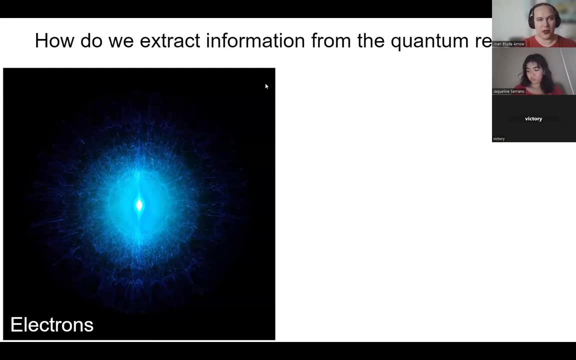 fringe. So certainly proteins, molecules and atoms. we can talk about quantum effects. So for now let's just focus on things that are smaller than atoms, So the electrons, protons and neutrons that make up An atom, And we're talking today about measurements. So the question is: I've got this. 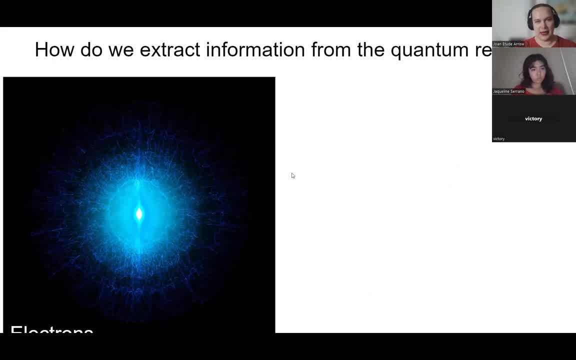 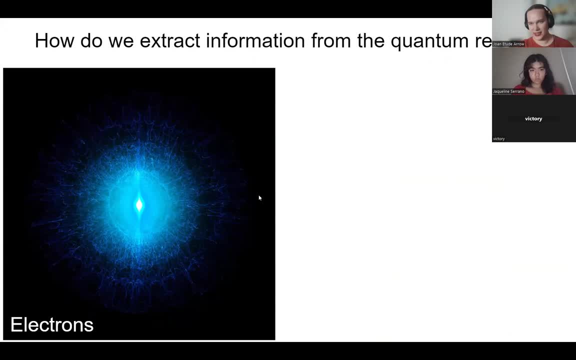 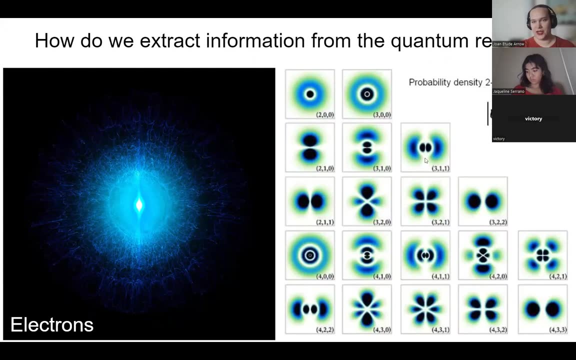 depiction of an electron on the left And real quick just want to clarify that when we imagine particles as little balls like this, this artistic representation is showing that's really not what these things are. If you have an electron bound to an atom, these are more accurate depictions of 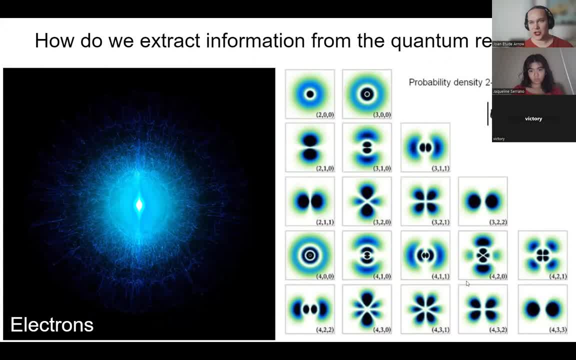 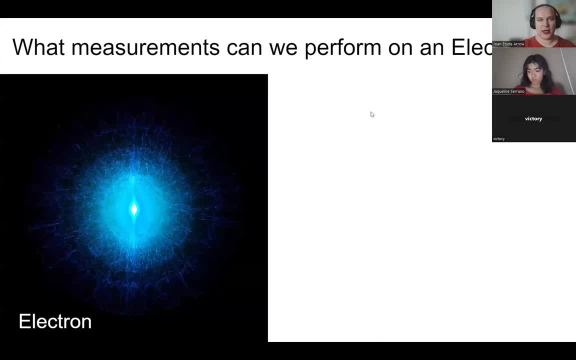 what that electrons Wave function might look like. So just just keep in mind, as we're going through this, that the left-hand picture it might be useful, but it isn't accurate. So we want to talk about: how do you extract? you know? what sorts of measurements can you? 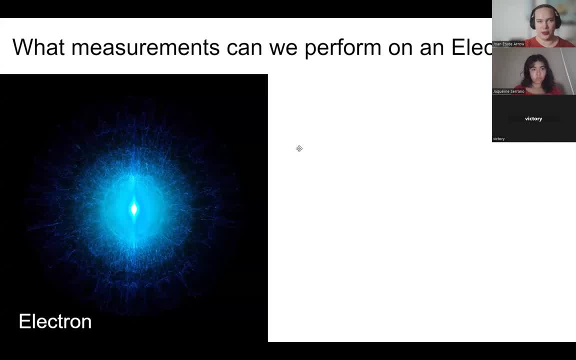 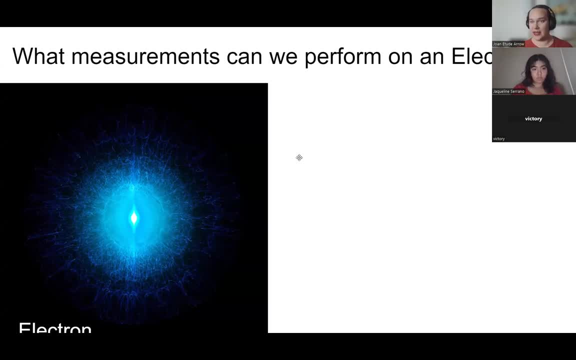 perform on an electron. What kinds of information can you pull from that? And we're imagining now our quantum computer. We want to build it out of electrons. Electrons are now the qubits that we're going to be using, And so the question is: what properties of the electron give? 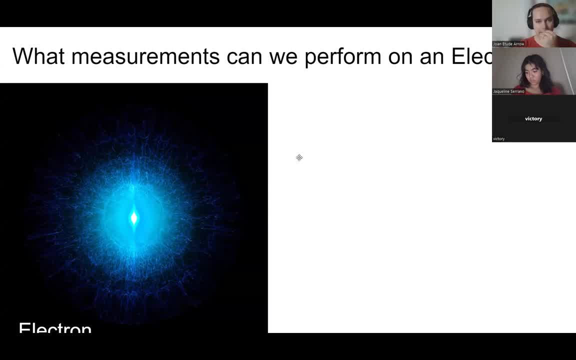 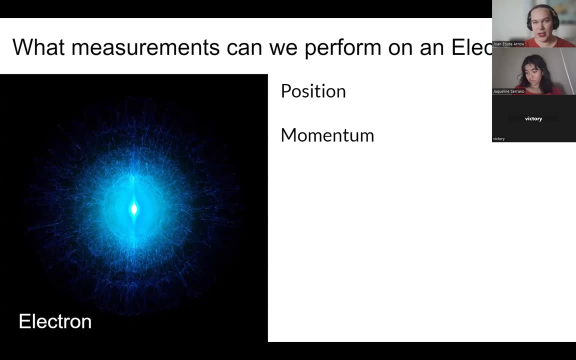 us the sort of two zero and one, you know kind of poles of that of that block sphere that an electron uses. So there's various properties we could measure about an electron. We could ask where is the electron, We could measure its position, We could ask how fast and in what. 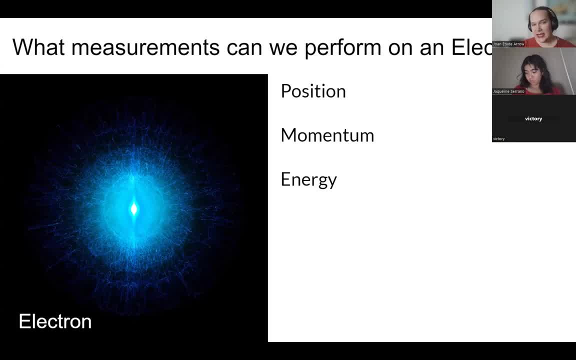 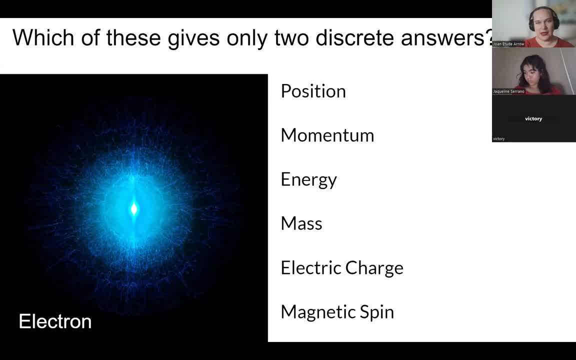 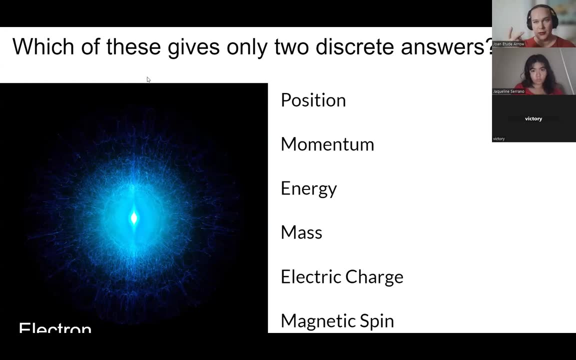 electric charge. What's the magnetic spin, And can you tell me you know which of these? these are all the you know various properties. We want to pick the one that gives. that can only give us two discrete answers. We might not know which one, but it can only give us two. 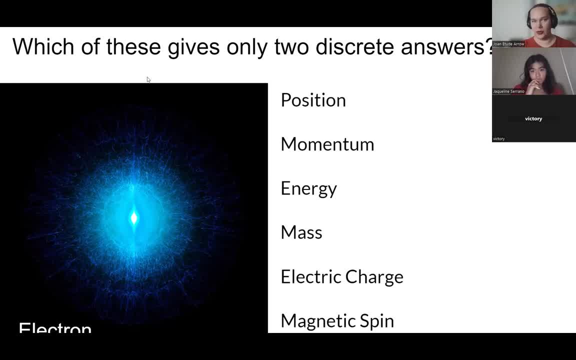 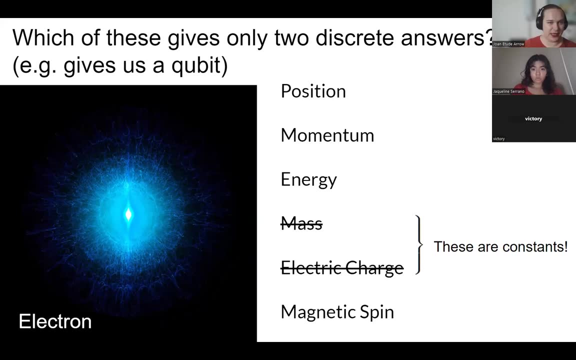 numerical answers, because that'll give us our qubits that we're looking for. Um. so first I'll ask: mass and electric charge. Does that give us two discrete answers? Uh no, Electrons have the same mass. They all have the same electric charge. This is actually a feature. 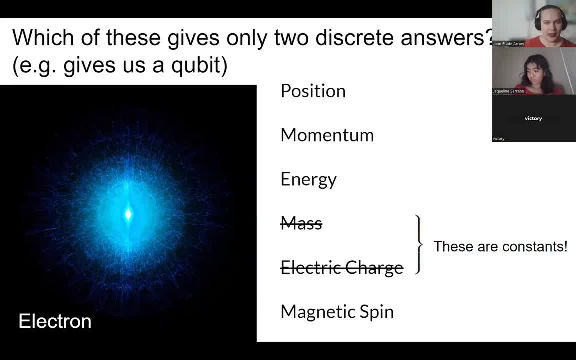 that you use to identify. oh, that thing's an electron because it has those, that mass and electric charge. So because of those things are constant. if you measure them, you're not going to get probabilistic. you know ones or zeros. You're not going to get a distribution of answers. 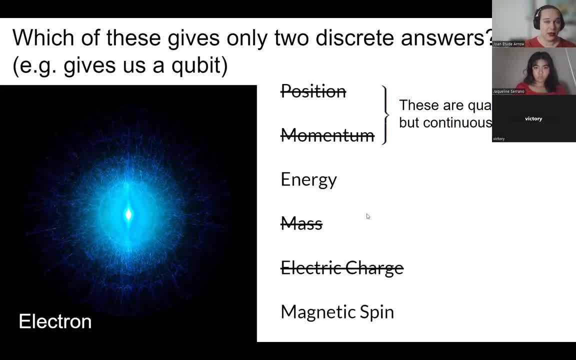 So maybe we want to look at position or momentum. Those things are quantum. Um, you, you, you can describe them using a quantum state. Um, let's say you have a, an electron, trapped in a box That's one meter wide. It'll be somewhere in there, from zero to one meters, So that is a. that is a quantum. 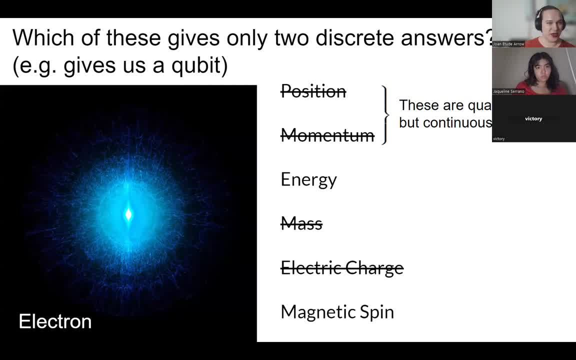 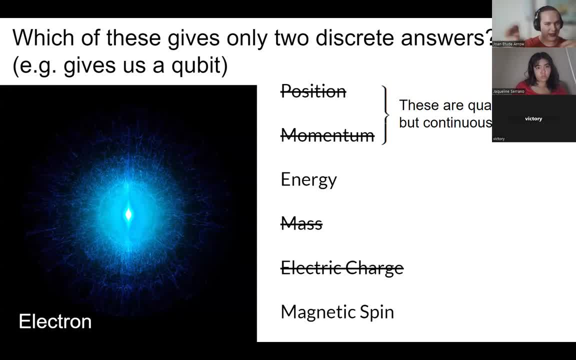 0.53 or 0.01234567,. right, It could be at any point inside of this box we've created for the electron Um and, yeah, you know, continuous, uh, quantum variables, is is a whole, you know. 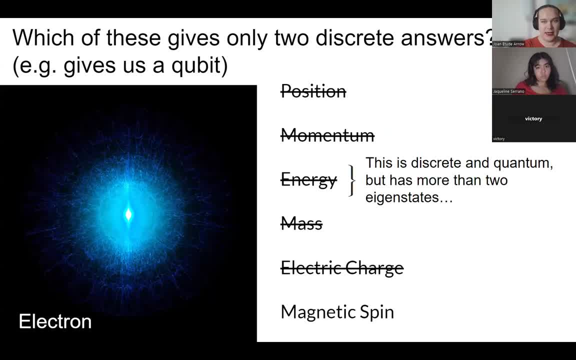 field unto itself, but for our purposes, it's not what we want to be using. You could measure the energy of an electron, And again I'm imagining this: uh, electron might be bound to an atom. Um, so you will have a discrete energy, It will be quantum. 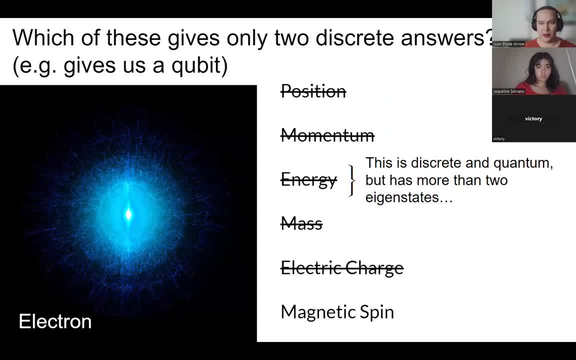 So in the sense that you'll not be able to tell a priori what it'll be beforehand, uh, but it can be more than one value. So an atom can have um, an electron, bound to it, And that electron might sit at the first energy level, the ground state, the lowest energy. It could be one. 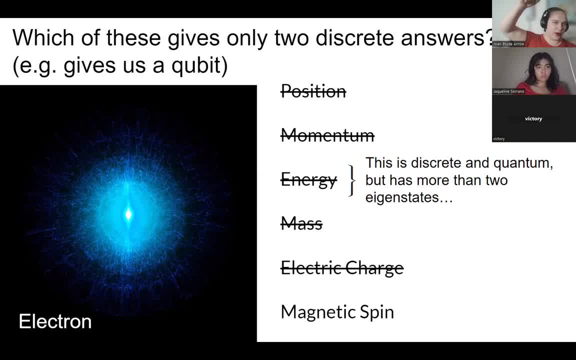 level higher, or one level higher, or it could be, you know, a number of energy levels higher up. So, um, if we only want to, you know, some people rig up their experiments to try and restrict the electron from going higher than one energy level, And if you do that then you only have two. 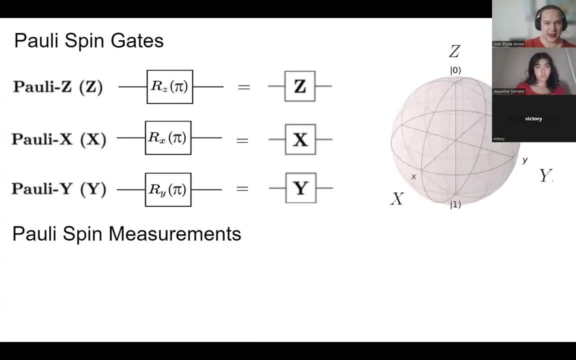 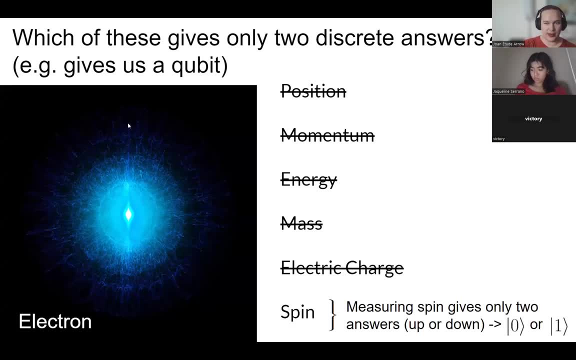 there's a qubit, But for our purposes I like to think of um, the spin, the magnetic spin of an electron, And so what you know, you know my ask: what? what is this property and why do we call it? 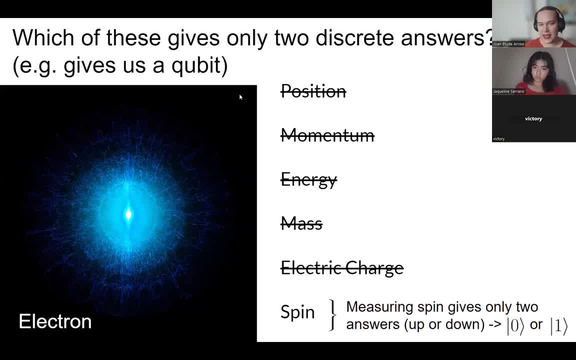 spin. It's kind of mysterious, but for the purposes of time, today you can just think an electron- We already talked about the fact that it has an electric charge, It gives off an electric field. And similarly, an electron has a property called magnetic spin, which means that it gives off a. 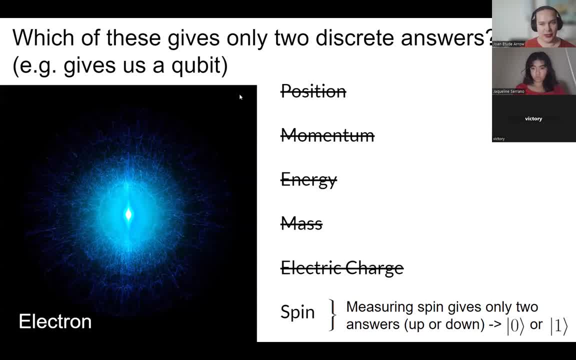 magnetic field. It interacts with magnetic fields, And so when you measure the spin of an electron, you're measuring which direction that spin is, And so you could measure it as up- That would be your zero- the top of the block sphere, or down- Uh, that could be the one, the bottom of the 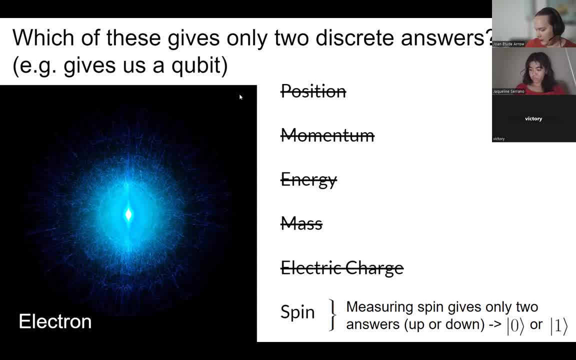 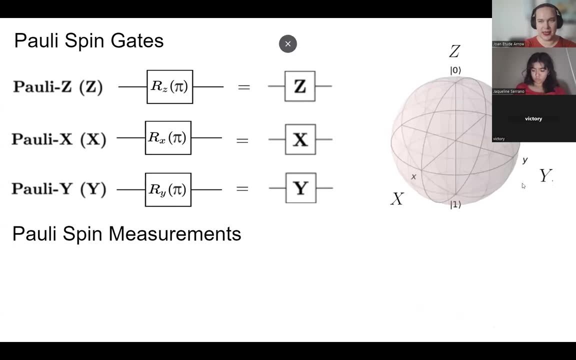 block sphere And I picked electron spin. People build quantum computers using qubits, of all the different you know uh ways. you know electrons might be one way, Um, but I like this way because it feels more directly analogous to the visualization we've been using of of the 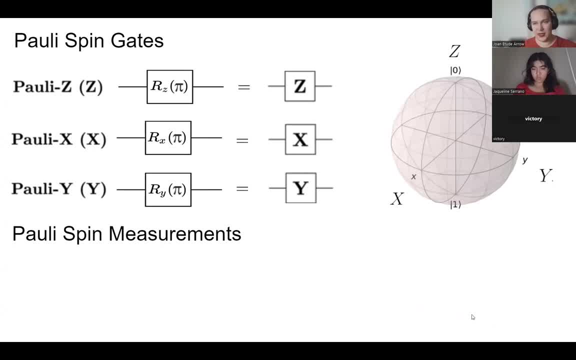 block sphere. So you can imagine this block sphere as the representation of the magnet, the, the different directions that you could measure. the magnetic field You could measure in the Z direction, which is that vertical axis on the block sphere, And then you could measure the. 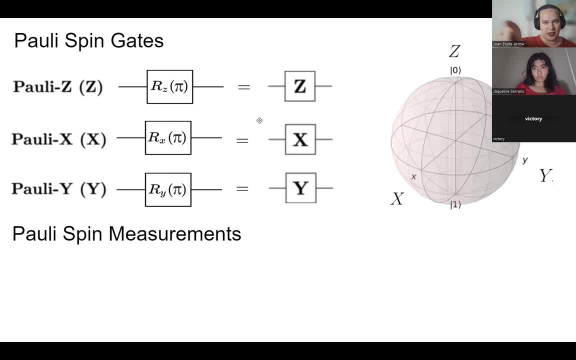 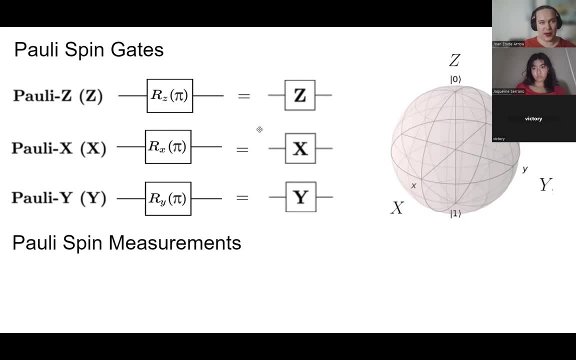 block sphere that you can see there on the screen on the right. You could measure it in the X direction or the Y direction, And so those measurements of magnetic field can be represented using what we call the Pauli operators. And these are just special cases of these rotations. we 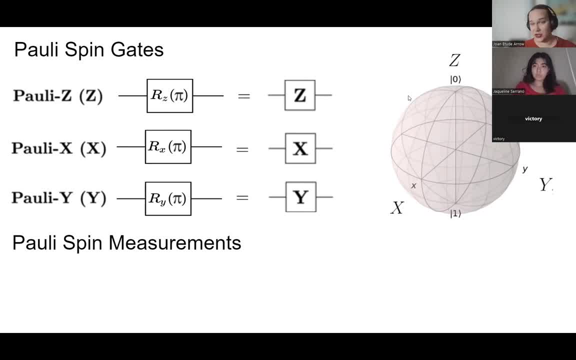 already introduced. Um, so because they're so special, they get their own name. So instead of writing R sub Z of pi, which is 180 degree rotation about the Z axis, I'm just going to uh denote that as the Pauli Z. And so again the the we're talking about measurements in. 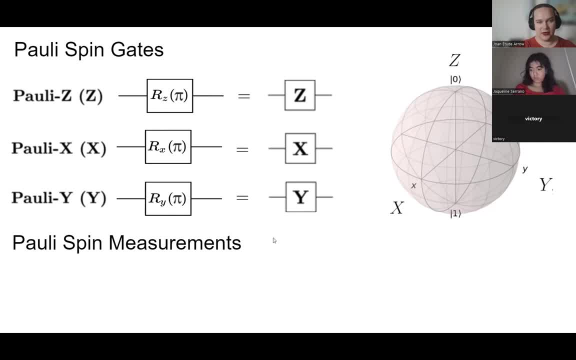 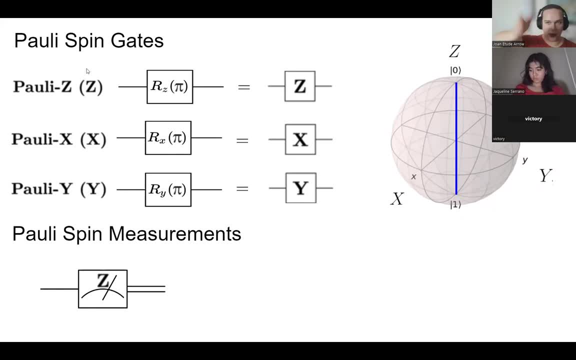 this, uh, in this section these you can think of as measurements of magnetic spin, of an electron Um, so that that blue vertical line is a measurement of the Z axis. And on the bottom left corner you can see how you would represent that in a quantum algorithm or in a quantum. 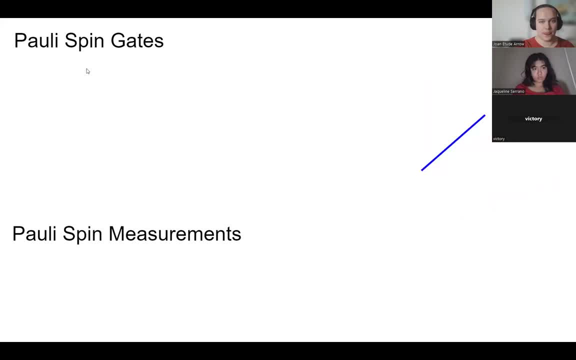 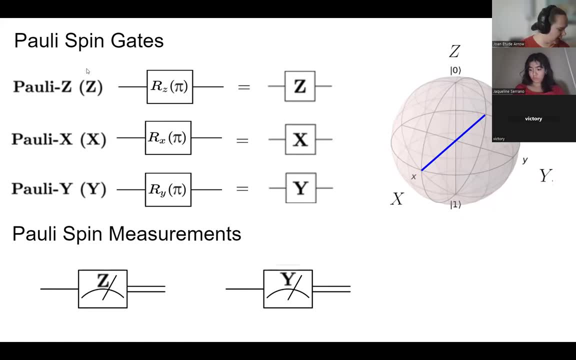 circuit. Um, okay, I'm going to move a little bit farther forward and we can happy to answer questions, but I just want to make sure I leave enough time for victories. uh, uh, his, his section. Um, so for now you can think of just there's these three different measurements that we can. 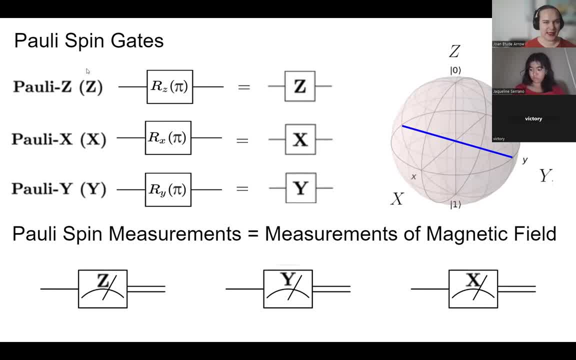 perform, which are related to these Pauli uh gates, these Pauli operators, and we can represent them, as with these little the the, the box with the little swoop and the cross. it's meant to look like the dial on an instrument, like it's a uh volt meter or something like that. That's where 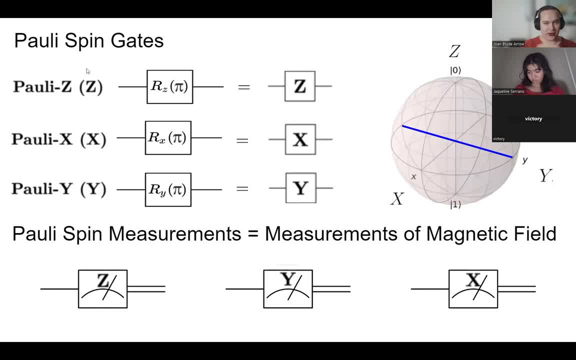 that notation comes from. So it's, it's basically just re diagrammatically representing: oh, I'm measuring the magnetism in this in the Z direction or measuring it in the Y or the X. And just a little note on notation, because the Z, uh magnetic. 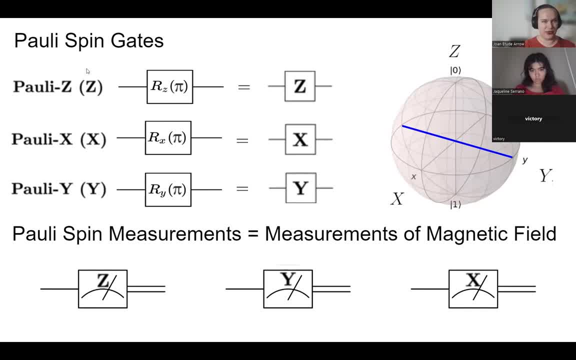 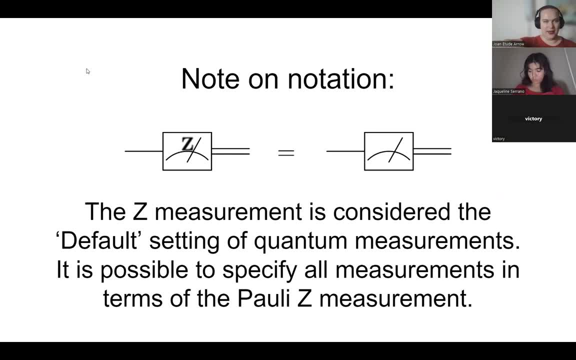 measurement aligns with the zero and the ones, those standard basis elements. We typically just don't leave the Z off. So if you see a box with a dial in it that doesn't have an X, Y or a Z, it's assumed that it's a Z. uh, because that's the most common measurement, that people uh. 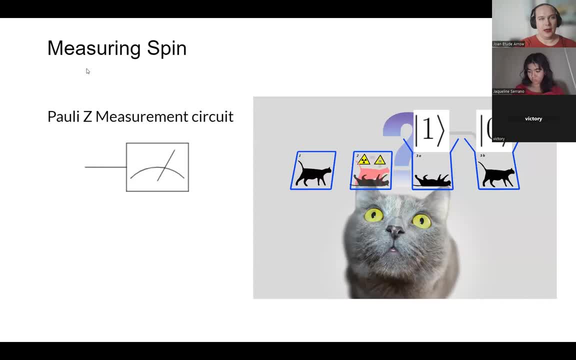 use as the kind of the standard one. Okay, So again. uh, we talked about like these measurements. they physically mean you know how we're extracting information from the circuit, how we get it A zero or a one that could be the shortening is cat finding it alive or dead? Um, and. 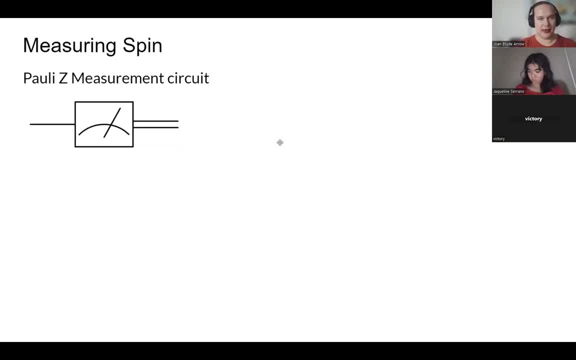 and those measurement outcomes are what? what comes out of the circuit? Um, so let's see So the, the measurement can be thought of as a question. you're asking that, you're asking the electron is your spin up or down? Uh, and it could be quantum, It could be. 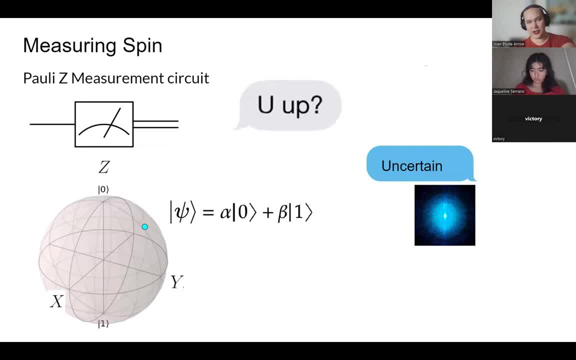 uncertain. And then, um, you know you could, that uncertainty could be this: you know a blue dot that isn't exactly on that vertical Z axis, And so, if you describe it as a sum, um, what this sum does is it basically just tells you the likelihood of each zero or one. Remember how? 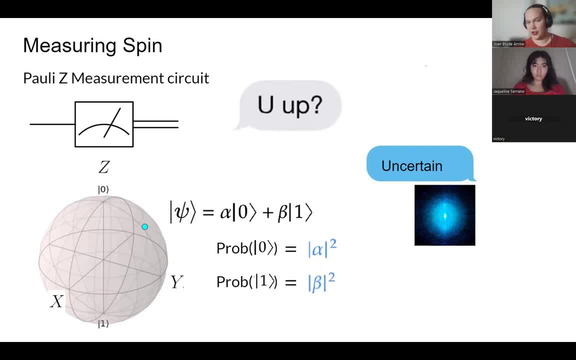 we said, if it's closer to zero, it'll be more likely to be measured as zero, And so this is just our way of now quantifying what is the probability of measuring zero. Well, it's the coefficient in front of it, squared Uh. so if there was a square root of one, then it would be. 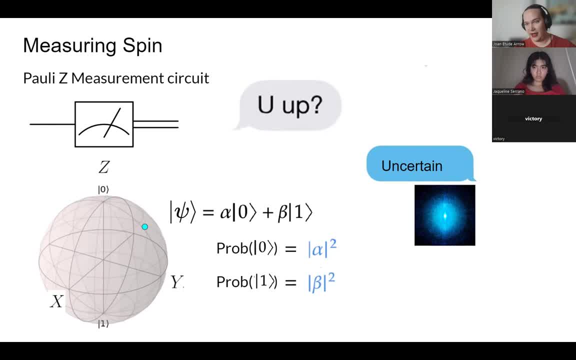 one over two. in front of that I square it, Then the probability is a half. that would be on the equator. I'm going a little fast, Um, so we can. uh, I'm happy to answer uh questions on this. 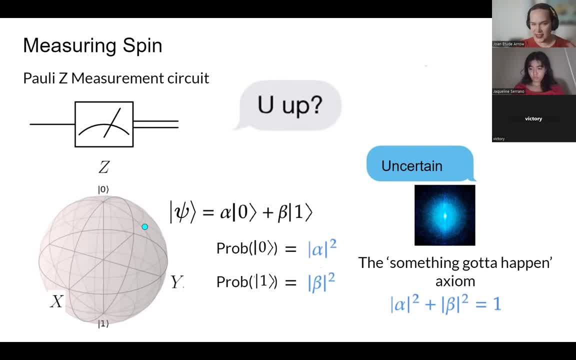 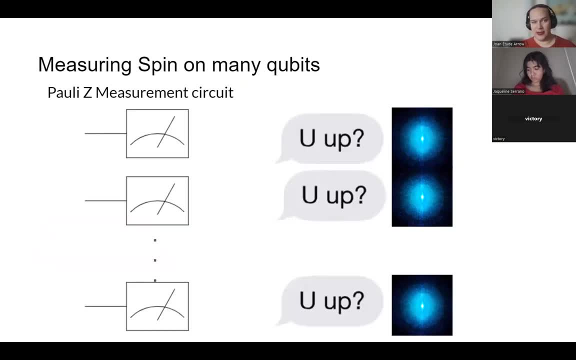 but the bottom line is you can measure, uh, this thing, And if it's in a quantum state, it'll give you a probability of zero or a probability of one, And you can do that with many, many qubits. Um, you know, you build a quantum computer to have multiple components. 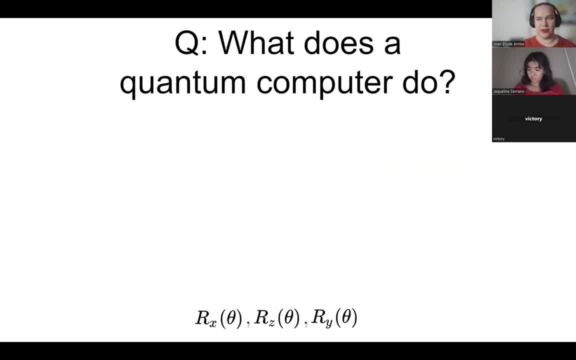 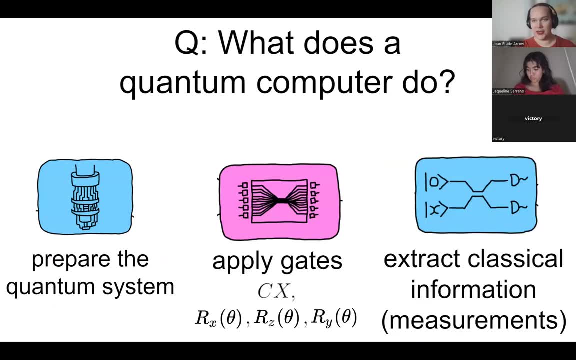 not just one. So that's happening. uh, you know, for for each of those. this is the point that I wanted to get to at the end here. So we talked about how the you know what, what a quantum computer does. we can focus here on. 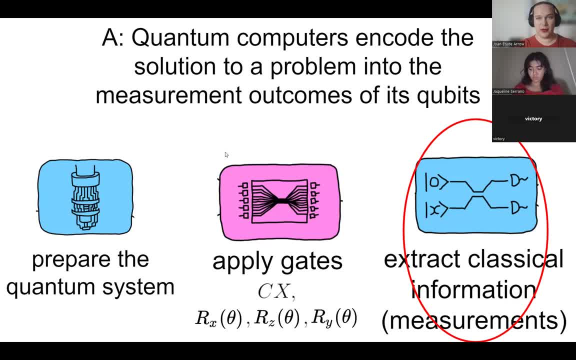 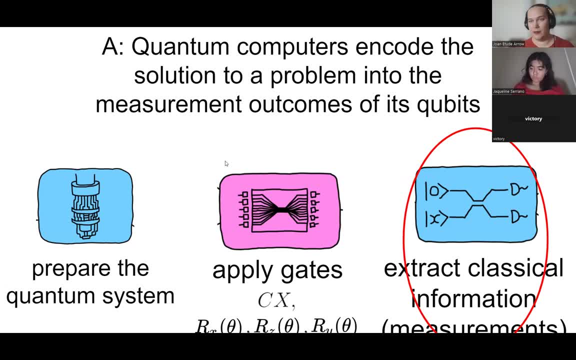 um, you know, uh, a quantum computer can be thought of as a device that encodes the solution of a problem into the measurement outcome of its qubits. So you can just think of the measurement as as the, the finale, the, the, the end result, the end result. 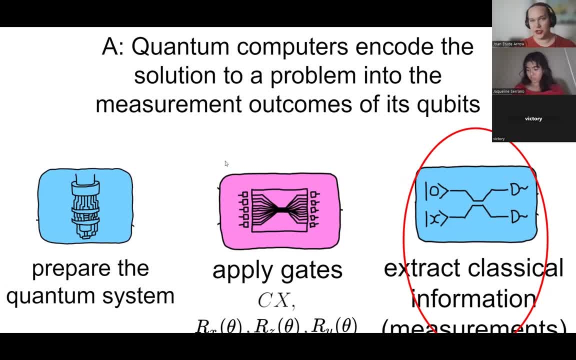 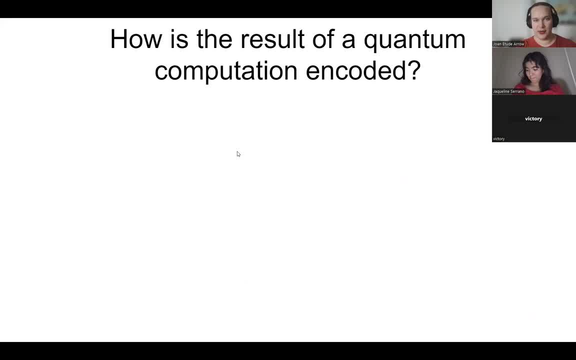 the end result. that actually tells you what you wanted to know about the solution to your problem. And so the question is: you know, how does a quantum computer encode the results of a computation? It might do it in a couple of different ways, Uh, but the first one. 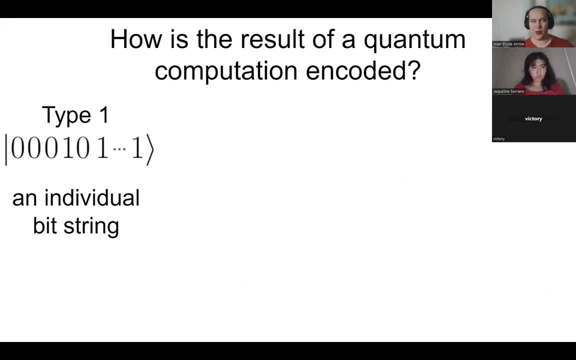 like, let's say, a silly problem. you're asking the quantum computer to tell you where to eat for dinner And you've encoded a bunch of different answers. The quantum computer computes all these crazy things you know, figures out the absolute best restaurant for you to eat at. 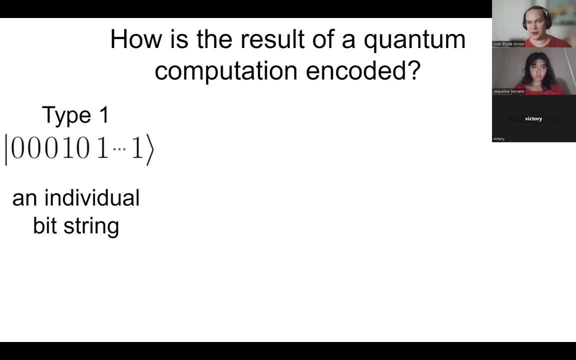 And it spits out just a single bit string, and that bit string corresponds to a specific restaurant that you've encoded. So that could be one way a quantum computer tells you the answer. It just tells you one bit string with 100% probability, and all the other probabilities of the other bit strings are zero. 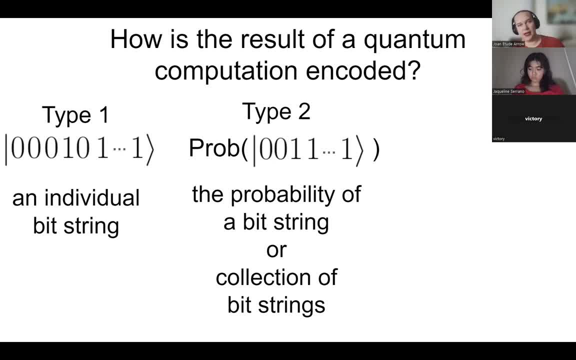 More commonly I see a type two uh- uh answer where instead let's say you want the quantum computer to calculate uh five plus three, That's eight. The quantum computer could encode that answer with uh by giving a specific uh bit string: 0.8 probability of being. 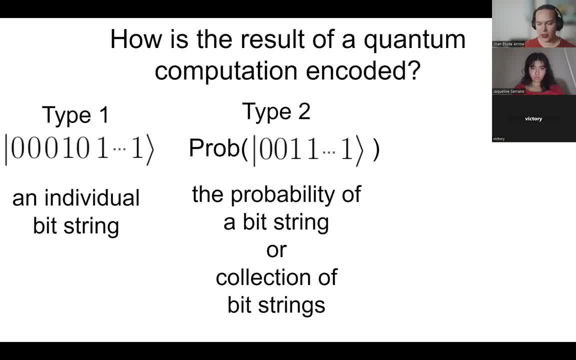 measured So you can think of the. the quantum computer can encode a numerical answer, uh, of the result of a calculation into the probability of a specific bit string. So that would mean you would have to measure, like you would have to look at the Schrodinger's cat multiple times. 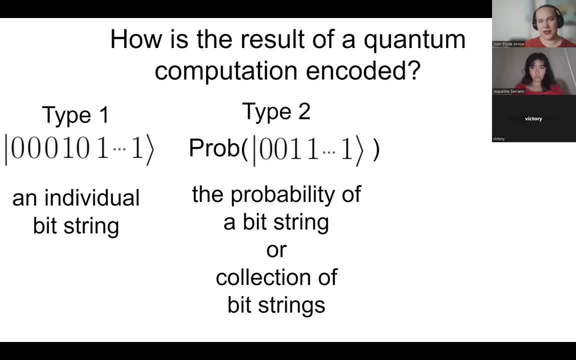 with multiple cats And calculate what is the probability of seeing the cat alive or dead. Maybe it's 50, 50,, maybe it's 70, 30. And if you know that the answer is the probability that Schrodinger's cat was alive. 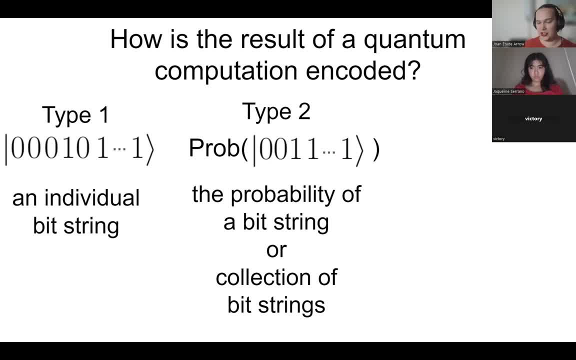 each time, and you see, the probability that he was alive each time is 0.536 or something. then that 0.536 is the numerical answer to your problem. Um, so cause again. quantum computers can only speak in the language of probabilities. 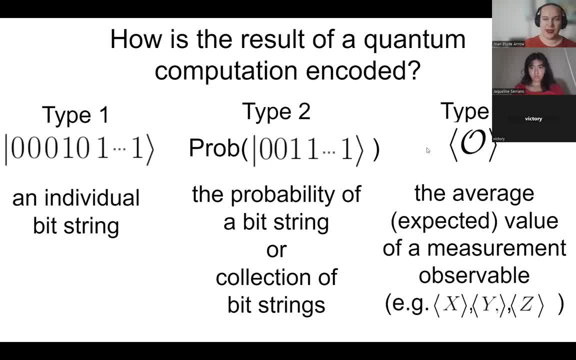 Um. and then finally- and this will be useful for the uh V, Q E challenge, uh, that we can talk about later- Um, you could measure the average value of a specific magnetic field, like the average value of the magnetic field in the Z direction, And the answer could be encoded in. 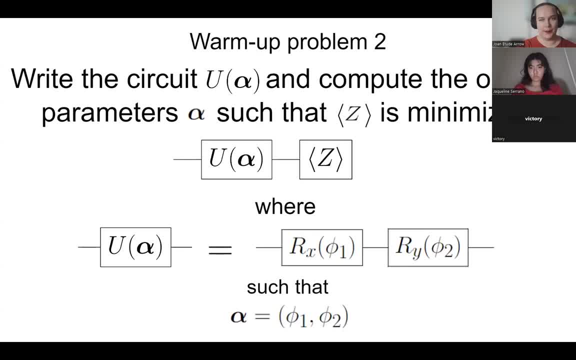 that average value of an operator. Um, so I'm going to skip over this. Um, I want to make sure we save enough time here. This is the end, Um, but this uh last slide is literally my warmup challenge too, where it's. 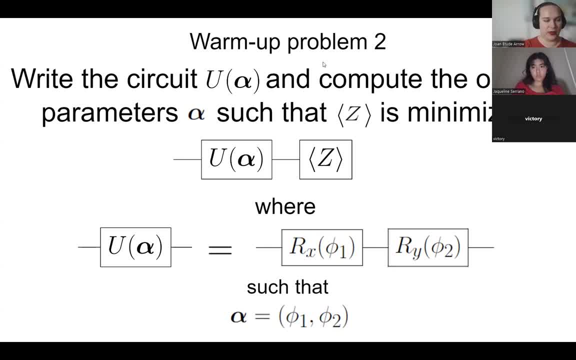 designed to give you some of those skills that we talked about that you'll need for the uh NVIDIA challenge on variational quantum. I can solve her. So, uh, Jackie, appreciate you taking that uh fire hose there. Um, uh, happy to answer questions, We can. let's let victory go, come and. 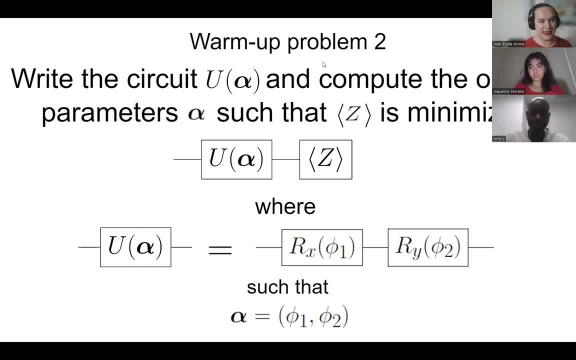 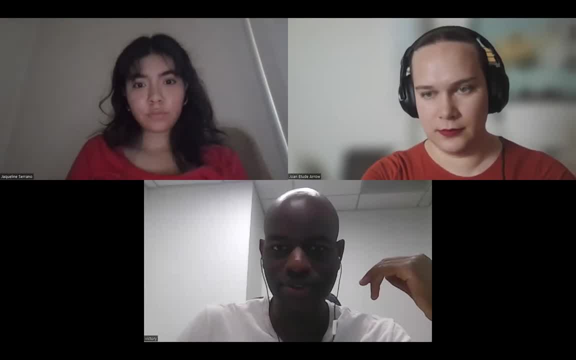 and give his materials. Uh, and then I can stay a little late, Jackie, if you've got some more questions. Yeah, So unfortunately the fire hose is not gonna, it's gonna just ramp up after this. Um, so uh. 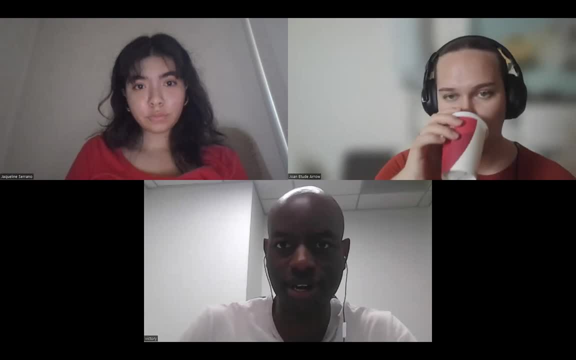 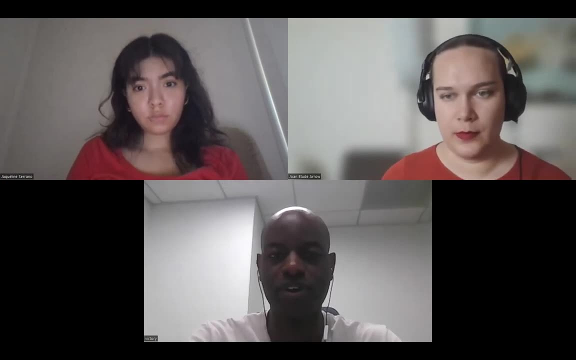 yeah, let me, um, yeah, so I'll give a brief, uh just, summary of what the- uh- supermark challenges are supposed to be. So the supermark challenges are supposed to address the problem- error correction- And the reason why I brought this up is because I've been a participant in hackathons. 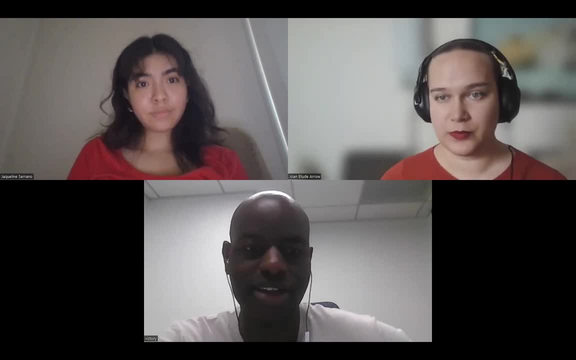 for like a day For a decade now. Um, I used to, you know, just do like classical computer hackathons back in college and you know quantum, you know find them most like a thing like then, like five. 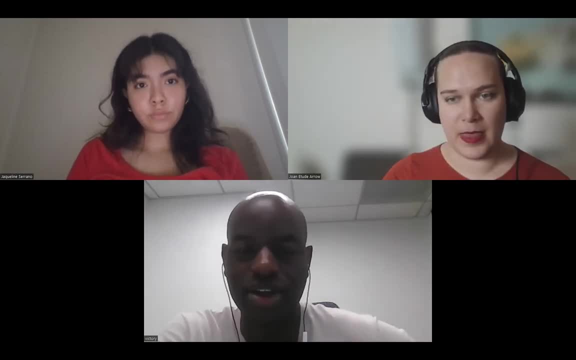 10 years ago, but that was becoming insanely popular. since I was an undergrad and you know, the concept of quantum hackathons has come around and um. now it's like you know these hackathons in Abu Dhabi and you know IQ hack and all these um, um online hackathons and stuff. The one thing 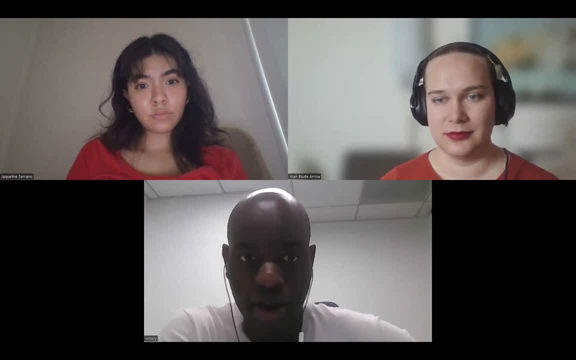 been missing in hackathons are these types of like quantum error correction specific projects. and just to give um a definition of quantum correction, um, when you existing quantum computers are very noisy, um and uh, the way you need to run quantum, these, these protocols on these noisy devices to make them less susceptible to noise, which makes your computation more reliable. 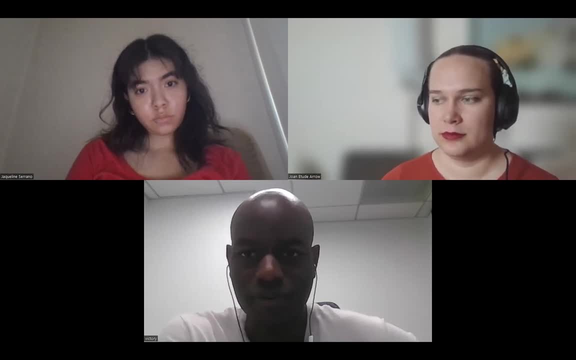 so the reason why this hasn't been been a focus on you know, hackathons and also the quantum industry in general, is because people believed, used to believe, that you know, you will get, like you know, practical applications without error correction. but over the past year or so the tide has changed. 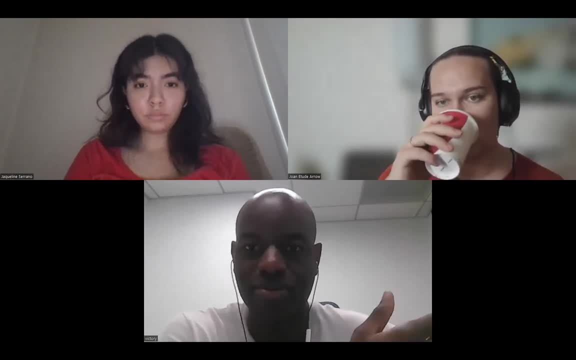 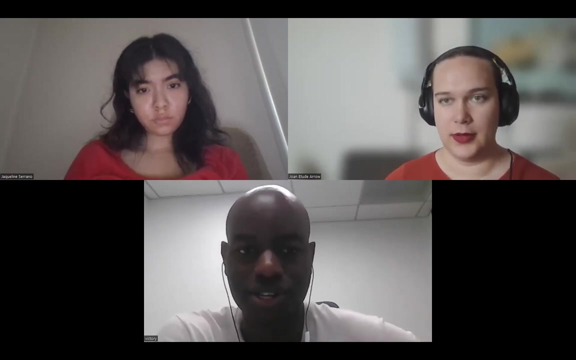 where, like most, the mainstream belief now is that we're not going to get um commercial, um applications of quantum computers without error correction. so a lot of, a lot of interest has has been um coming, uh, you know, being a part of the field recently, because because of this, this new um. 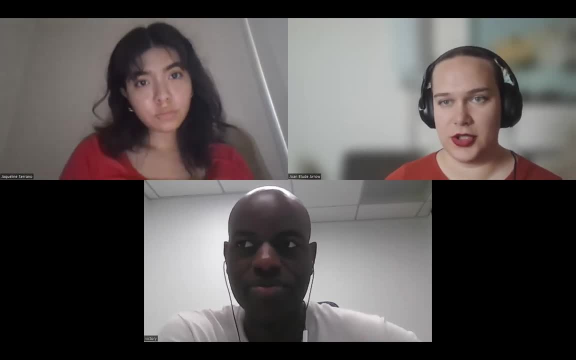 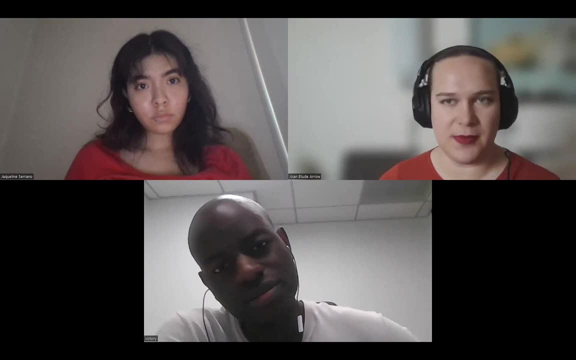 change in opinions in the field. so just to chime in real quick, because i haven't talked to jackie about noise before. noises can be pretty intuitive, uh process. just imagine you're trying to build a computer with like electrons or individual atoms and the only way to get those things to behave 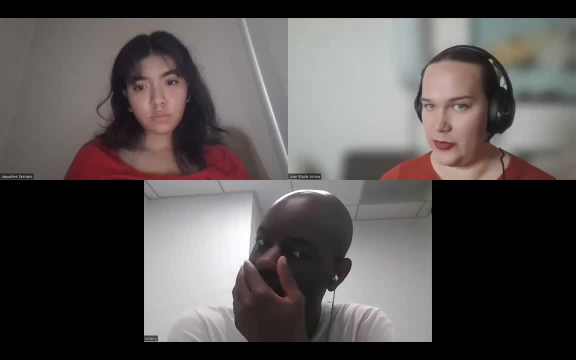 is if you make them very cold and keep them very still, you don't let them interact with anything, so that they can exist in their special quantum states. the challenge is that you also need them to be able to interact with you as the computer operator, and with the neighboring qubits, and so 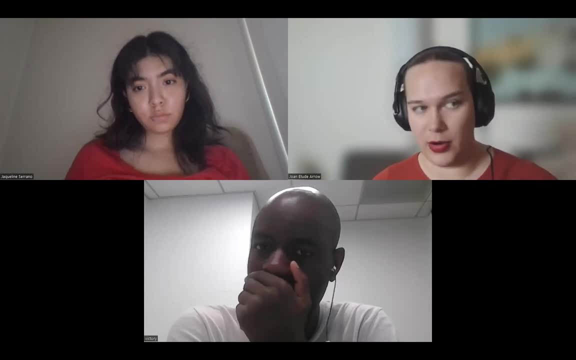 you have this trade-off where you could take a single atom and make it perfectly isolated and it would be great. it would have no noise, but then it wouldn't be able to talk to anything. and so as soon as you give these quantum uh states or these 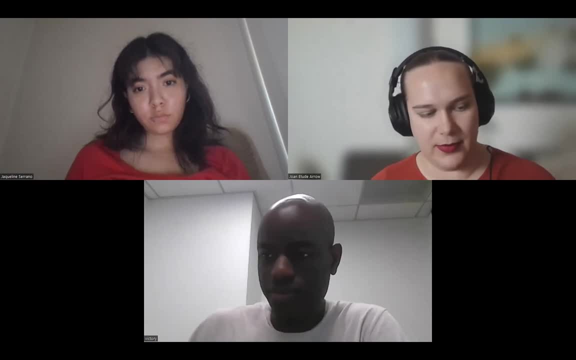 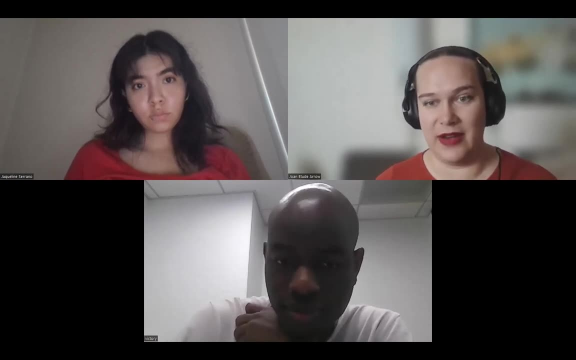 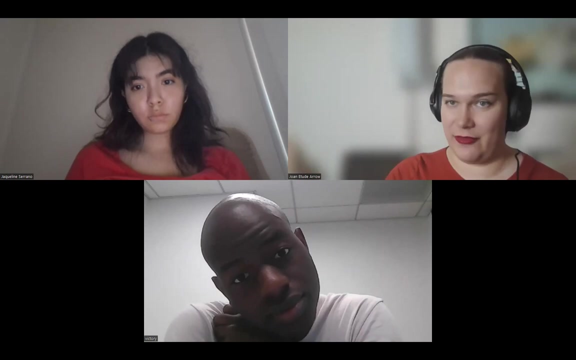 atoms, electrons, whatever you're building your computer out of, as soon as you have them interacting, any kind of environment, you could have them interact in a way you didn't expect and that manifests itself as a computational step. you didn't mean to happen. uh, and then imagine those building. 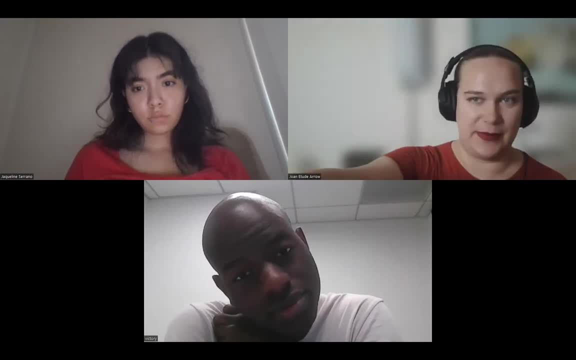 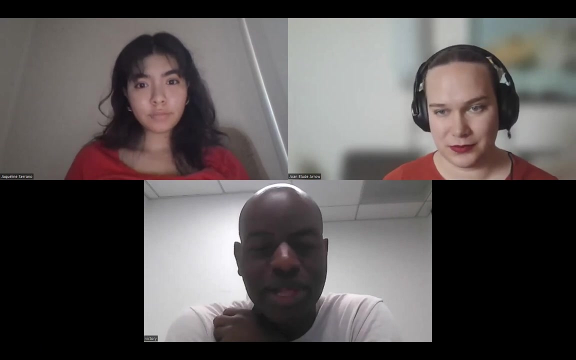 ever through every single component of the system, many, many steps along the line and then you worry that your, your program is just going to turn to mush because the the noise runs rampant and ruins your calculation. uh, yeah, thanks, thanks for um, giving uh more context and please, like you know, i, i, i'm, uh, i'm, i haven't really explained this stuff to like your first. 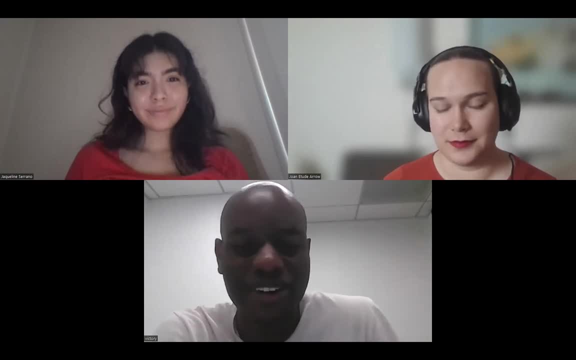 second year, so please, uh, interrupt me when i say a definition that hasn't been defined. yeah, no, you're doing great victory and and teaching uh like jackie is a trooper. jackie and the rest of her team are are quite courageous in my view. like i didn't start seeing this stuff. 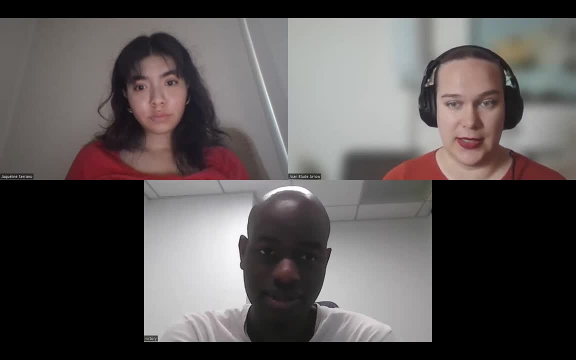 uh, that they're gonna be trying in the in the hackathon challenge until grad school, um, and it, what, what? you know, it's part of my role to make this stuff as accessible as possible and i think it prevents, you know, a really novel challenge. you know how can we take these um, these core? 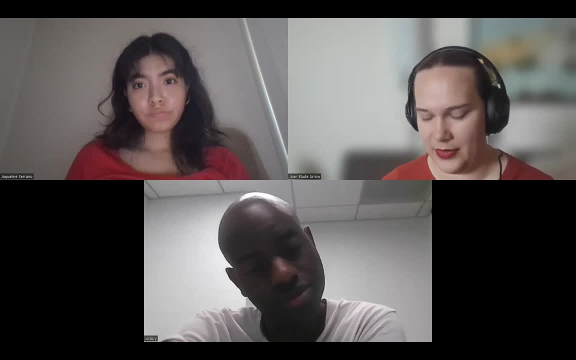 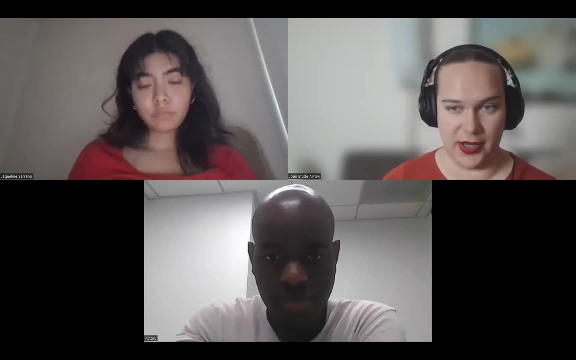 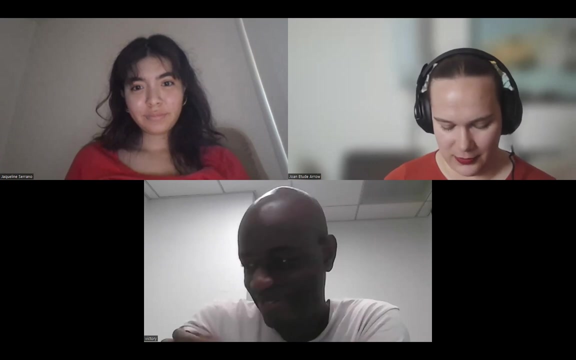 concepts like error correction and um, the, the nvidia challenges on quantum machine learning, and make them doable for students who have just started learning python or just starting taking calculus. i believe it's possible, but uh, the, the pedagogical and the educational approaches um need to be developed and refined. so, yeah, okay, yeah, so, yeah, exactly, so, yeah, so you. 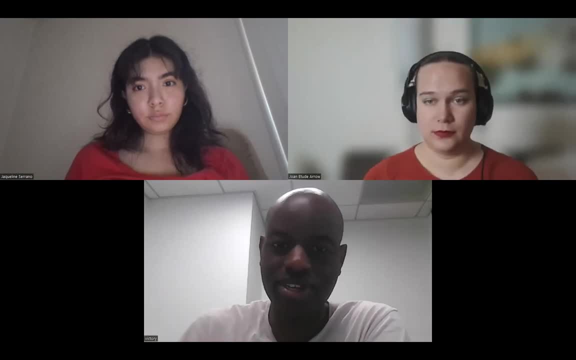 you want to build a computer and it has noise. and the reason why this is not a problem for your phone or this laptop or, you know, just classical computers, is because the laws of quantum mechanics, behavior friendly, which has been uh- were explained by you know, certain measurements um change the 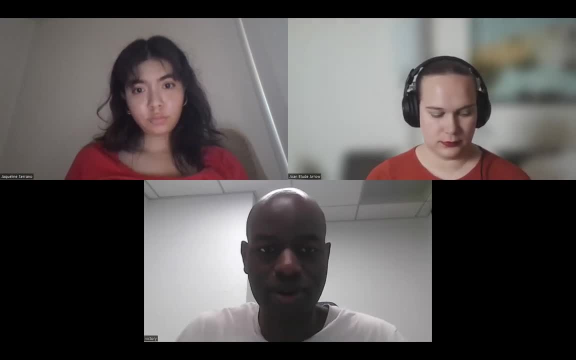 state and also the no cloning theory. have we? have we talked about the no cloning theorem yet? or we've, we have not. okay, so the no cloning theorem just says that if i give you a state and you don't know what it is, um, you can't make a perfect copy of it. so there's no copy paste on a quantum computer. 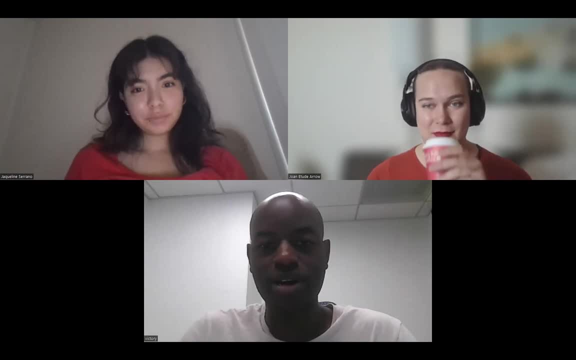 yeah, so the way, the way that your phone, your laptop, uh, your ps5- deals with errors, is it just copy. it just takes your bit and it just copies it multiple times. so if there's an error on one, it does a majority vote. it just checks for the most popular. 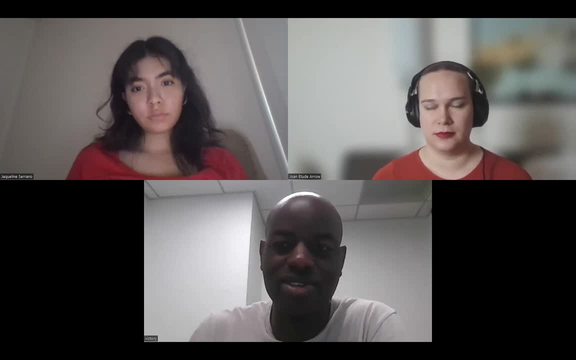 uh bit, and then it's so, uh, one, one actual. they're called error correcting code. so one error correcting code would be, um, a bit flip code, where you take three bits and then you use that to encode one logical bit. so those three bits, so there's a concept of physical bits which are your actual. 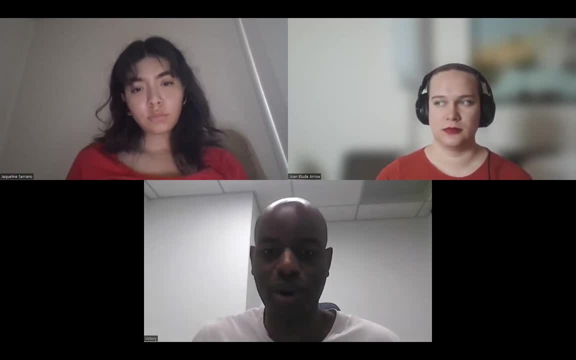 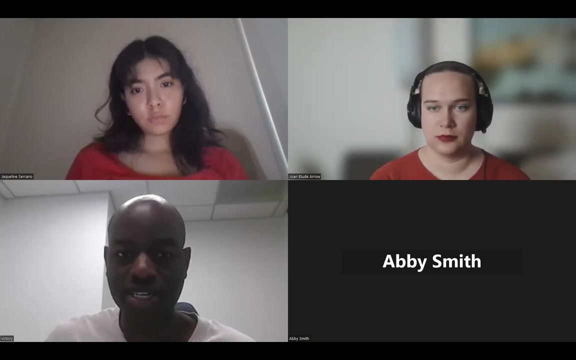 bits and then there's a logical bit which is: those three bits represent their logical bit. so if there's, if it, if i can say like: oh, if it's all zeros, uh one, uh, three zeros, that's one logical bit, that's just a logical zero. so if there's an error on one of those bits and then i check those bits, i can see that. um. 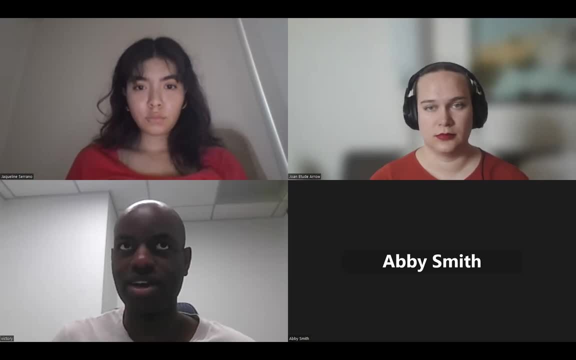 you know, i i can have like zero, one zero, so then i can say, oh, um, two is more than one. i know that i it's. it has to still be a zero. so an arrow might have happened. so then i can correct for that error, so i can apply: um, i i. 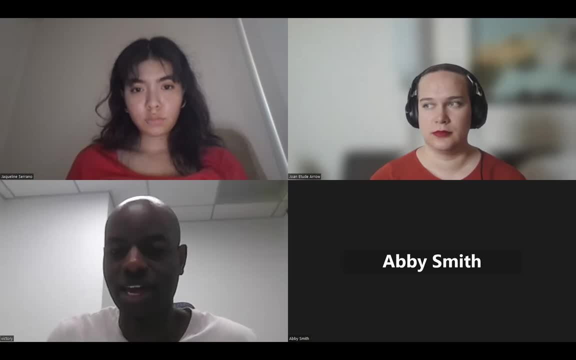 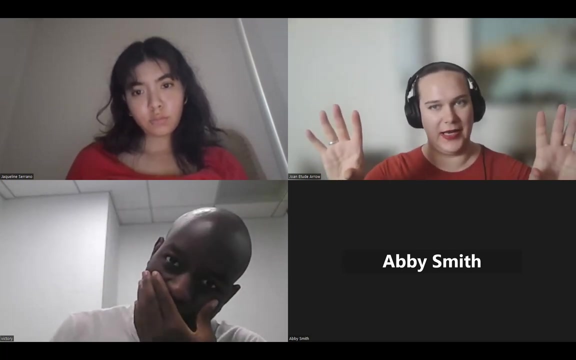 get an operation on that logical bit that corrects for that uh bit flipper. it's a pretty, it's. it's not a terribly hard concept. it's like, um, if you you've got a walkie talkie, you, you say a sentence, but let's say there was static in the middle of the sentence and but the message was clear on either. 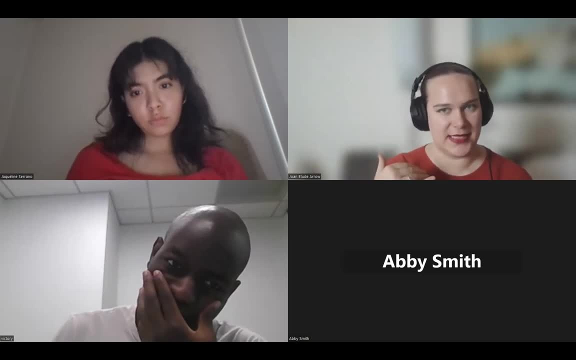 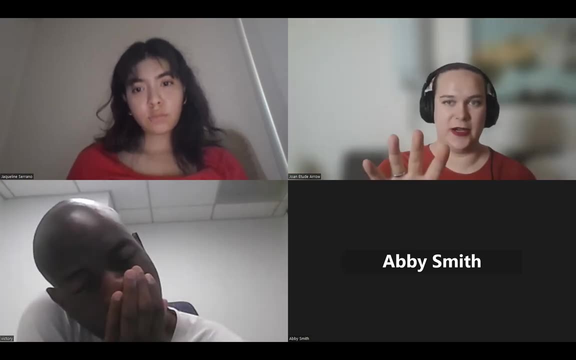 end. so the person is going to say: i didn't get the middle part, repeat. and then you say the exact same message again. maybe there's static at the beginning, but they already heard the beginning. and then there's it's clear in the middle: uh, maybe it's static at the end, but they already heard the end. so they can kind of put those two things. 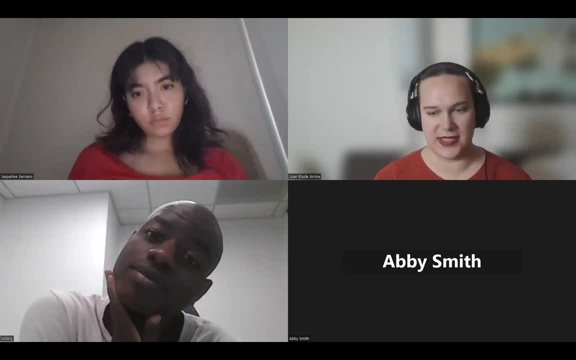 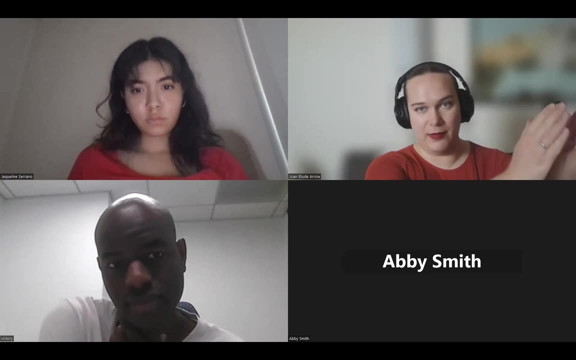 together and the idea of a repetition code is just, you know, the message might be: uh, zero one, zero one. so if you want a repetition code of five, you take every bit and repeat it five times, so you say zero, zero, zero, zero, zero, zero and send that, and then, even if one of those comes in wrong, 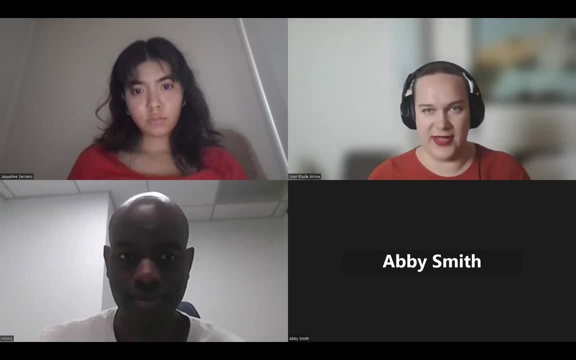 you, as victory said you take a majority vote. you're like: oh, four out of five of these are a zero, so i'm going to assume they were trying to tell me zero, exactly. also, victory, i enabled, uh screen sharing, so if you've got slides or anything, 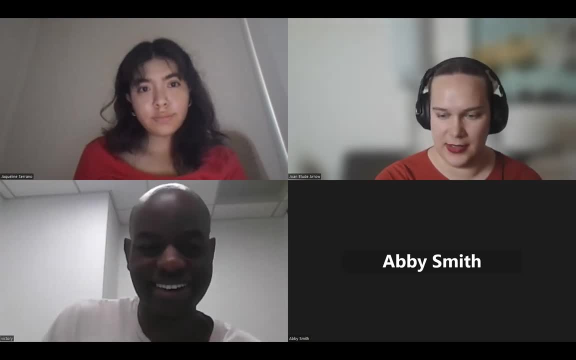 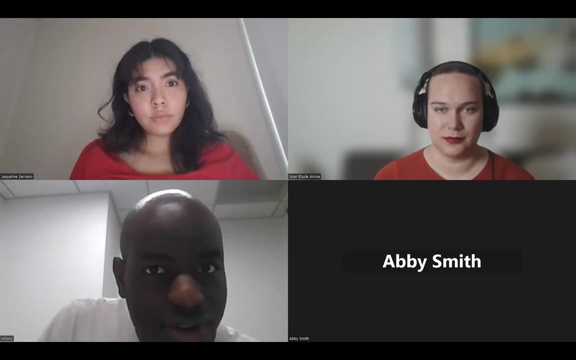 feel free to share those. and also, abby just joined us. hi, abby, hey, abby, we want to introduce yourself. hi, how are you so? uh, let's see, let's see here, um, can y'all, i can share my entire screen? okay, yeah, i can do that. okay, uh, let's see. okay, can you? can you see? 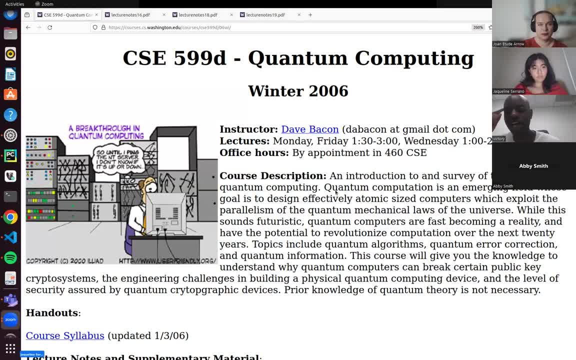 this i can. okay, so basically i i tried making slides and then i realized i was basically copying this. uh, i can send the link to this to this reference. this is a quantum computing course. uh, that was given by dave bacon. he's a software engineer at google and this is when he used to. 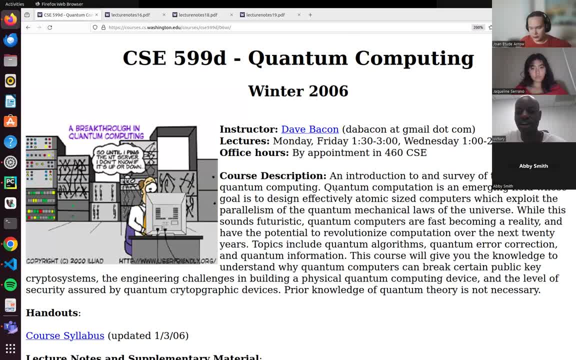 teach at um university of washington, but this is a quantum computing course basically. uh, i was basically the the general, uh, the general, like, um, uh, motivation for all the slides i was creating. i was like i might as well just share this and then walk through the lecture notes. 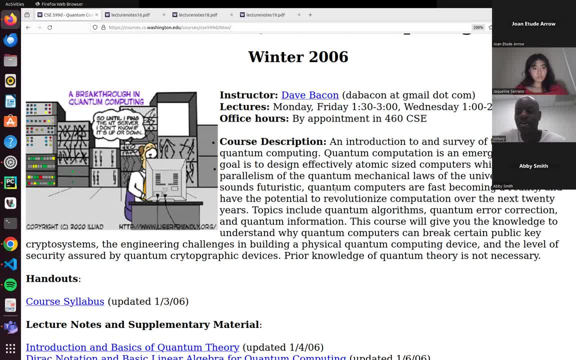 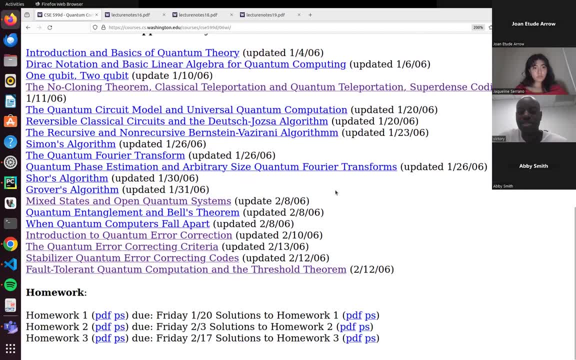 and that would just be basically uh give the same concept and also provide more context and um. i recommend that you uh read the sections if you do have the time, but the ones that i think are important for this hackathon is this: introduction to error correction, um. 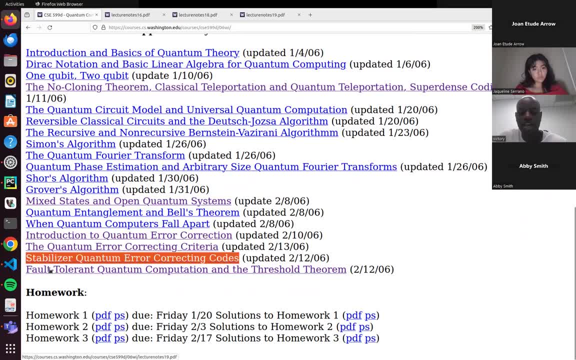 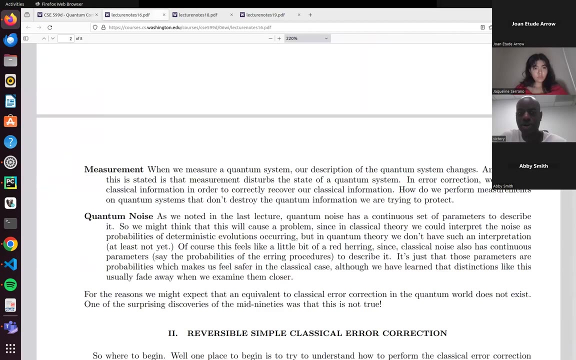 and this is what, uh, we were basically talking about when we're talking about um, you know, uh, you have, you have errors and, uh. this will just tell you a little bit more about what we're talking about, and this is what we were basically talking about when we're talking about um, you know, uh, you have. 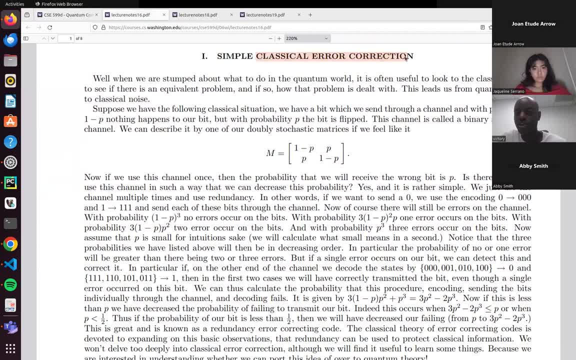 you have errors and, uh, this will just tell you a little bit more about what we're talking, about, what we just explained on how to do classical error correction, where you do a majority vote on the bits that have errors. um, so then, uh, the reason you can't, yeah, the reason you can't do, 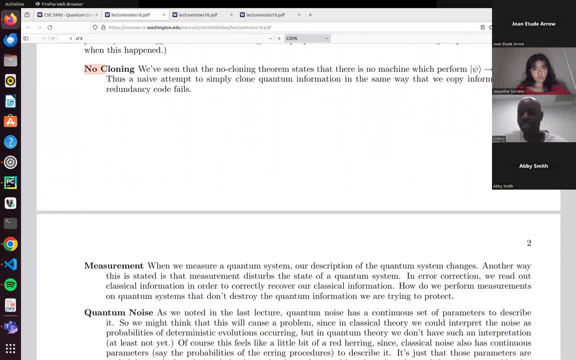 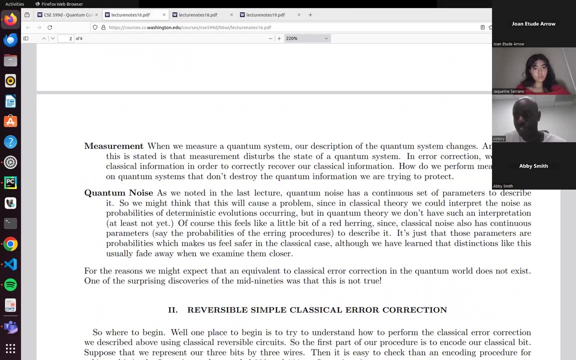 this quantumly is of the no cloning theorem, which you haven't heard of, but it's uh, basically there's a quantum mechanical uh law that says you can't copy these states. so then you can't just do whatever you do classically. you have to be more clever. um, uh, the noise. yeah, the noise disrupts. 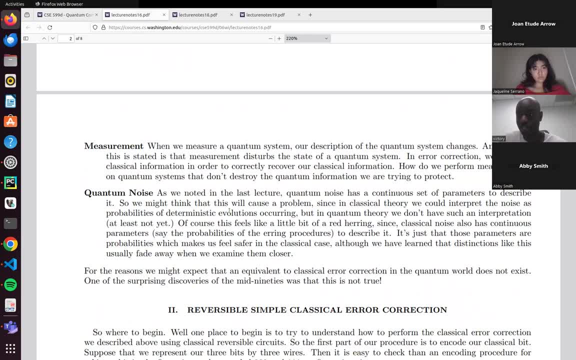 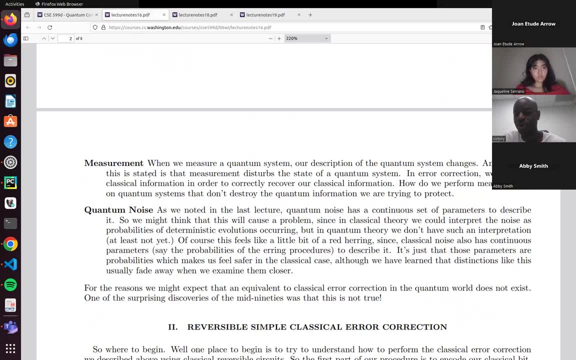 your state, uh, and quantum noise behaves, uh, the noise disrupts your state, uh, and quantum noise behaves differently than classical noise. and yeah, you also, you know when you we what we just talked about: when you measure a quantum system, that disrupts the quantum system, so you can't just measure, uh. 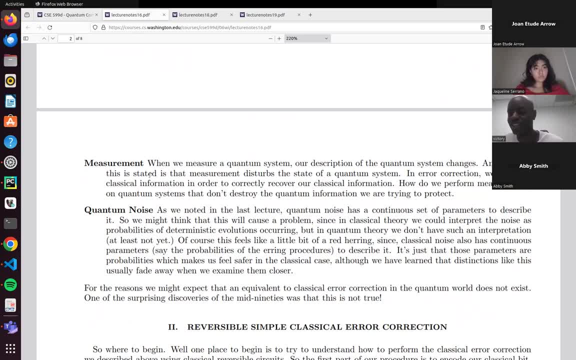 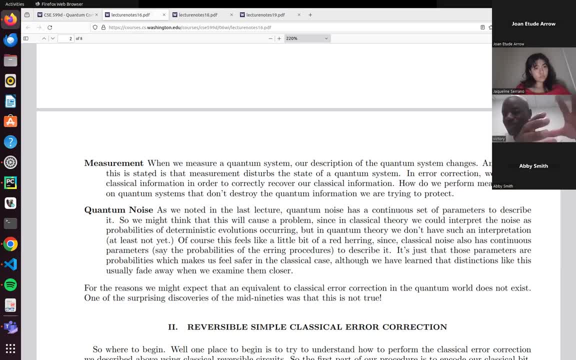 between states. so by measuring the parity- which is also another word, that that a technical term- you're basically measuring whether or not an error occurred. you're not finding out which error occurred, and by measuring disparity, it just gives you syndromes, which is symptoms of whether or not. 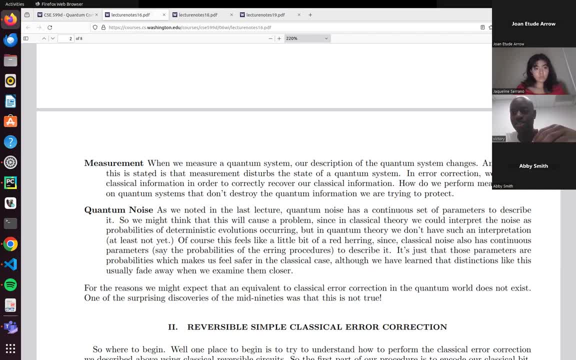 an error has happened when you state: um, okay, i'll stop, i'll pause there for your questions. so clarifications, uh, from joanne, yeah, just just, can you hear me okay? um, so the parity, parity measurement is just like, um, maybe define that a little bit. uh, my first thought is: like it's just 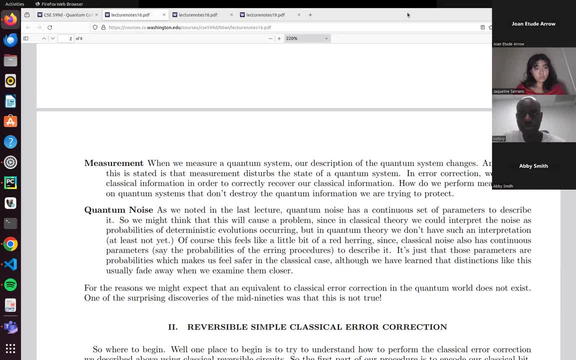 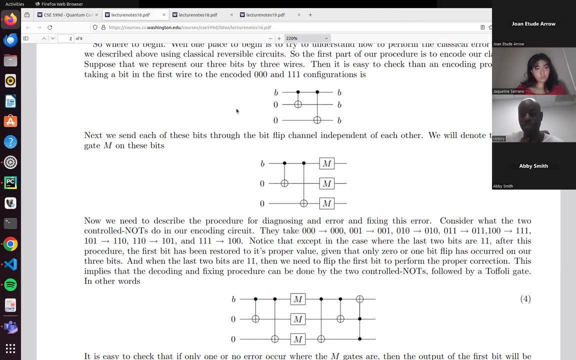 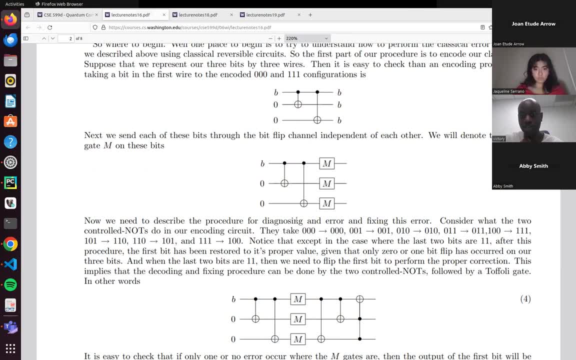 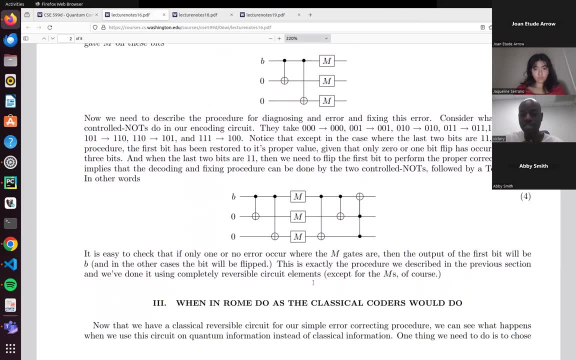 do is how to write the classical action action code on a on a on a classical computer. the m's stand for errors. so if m's, yeah, so um, just to, for we've. so we've seen, we've seen those um little gates that have the little circle plus through them. those are our x or entanglement. 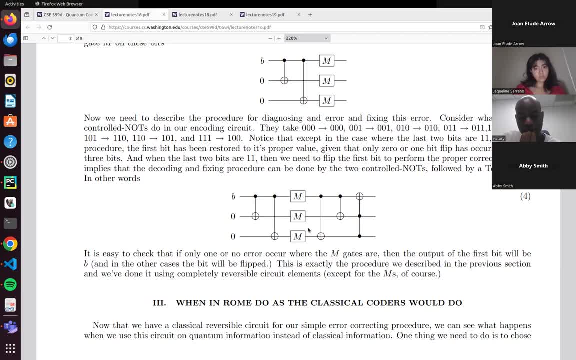 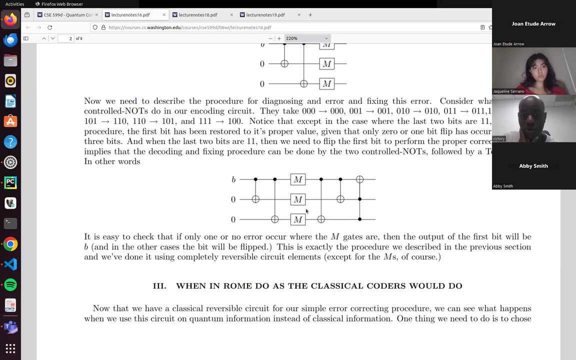 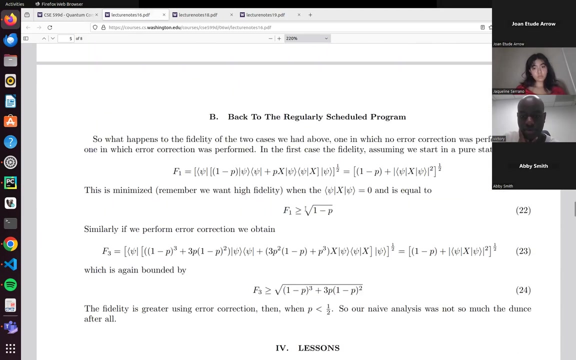 gates that we saw, um, so we have at least seen those, and so the the m boxes are just saying: um, something happened to the cubic, it right there, and i'm not sure what it is exactly. and, uh, basically, based based on what, what we measure, um, here you apply certain corrections. so, um, i will go way ahead, okay, so 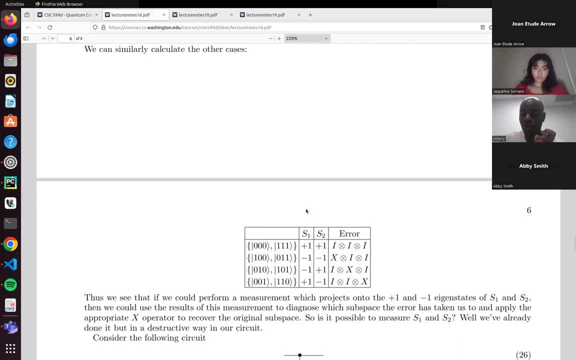 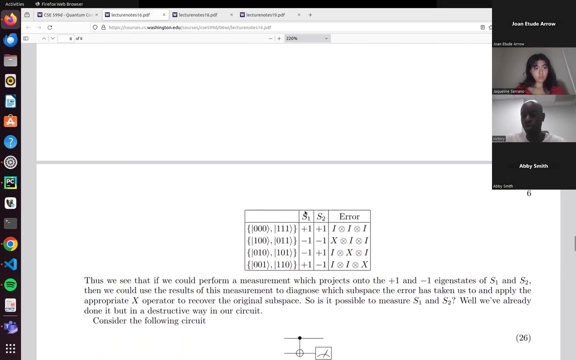 these, these are the simple measurements. so basically, uh, syndromes- again i said, are just uh. you're using certain qubits to detect whether or not an error happened on your state. so for the um, the repetition code which you're going through, you, you have two qubits. 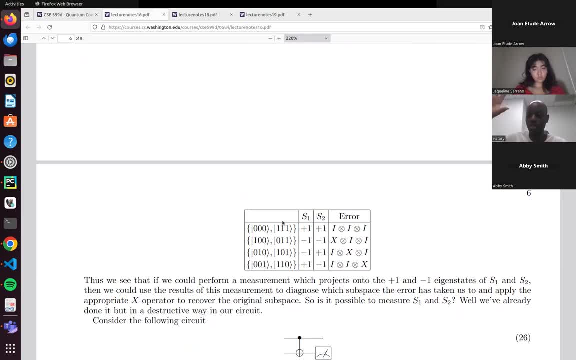 uh, that you are using to measure the syndromes of your three qubit, um, logical uh qubit, which which is what you're running the repetition code on. so if you get, if you measure those two qubits that you get um. so these are just eigenvalues, but you can say. you can say: 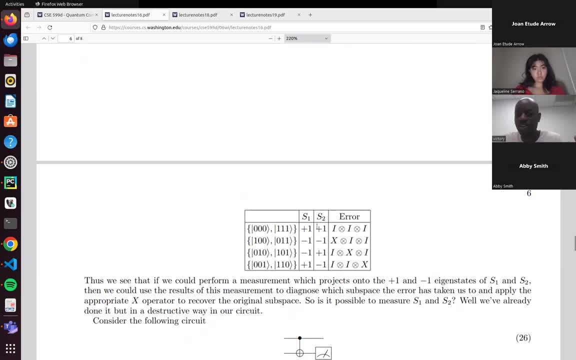 that plus one is a one and uh, minus one is a zero. so if you get a one one, then you know that no error happened on you, on your state. so then you, you don't do anything. if you get uh, um, uh one, sorry, also, this is one one. oh, sorry, uh, okay. uh, this is confusing. i'll say: plus one is uh, zero and minus. 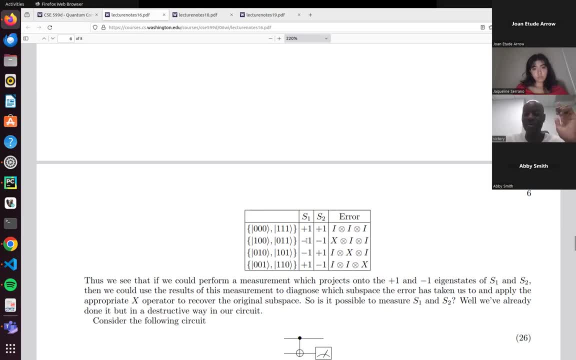 one is one, okay, so if you get uh one one, then you know that an x arrow happened on your first qubit, so that would be uh the x. that was what we just covered. jackie abby, you, you didn't see it. um, we talked about it in the very first part of the of the session, but the the x is um a pauli x uh gate. 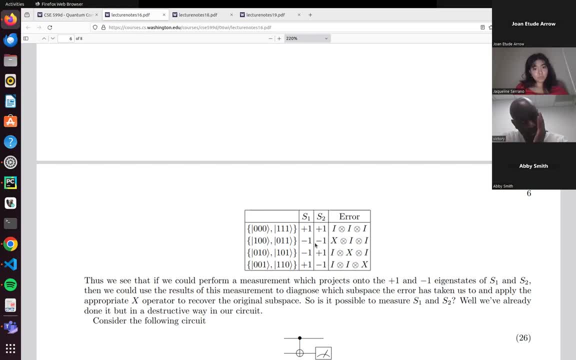 so what? what this is saying is that. so it's like um. the way i like to to give some intuition behind doing these syndrome measurements is it's like, um, you've built yourself a biometric scanning door. it scans someone's thumbprint and decides whether or not they are who you want, who you think they. 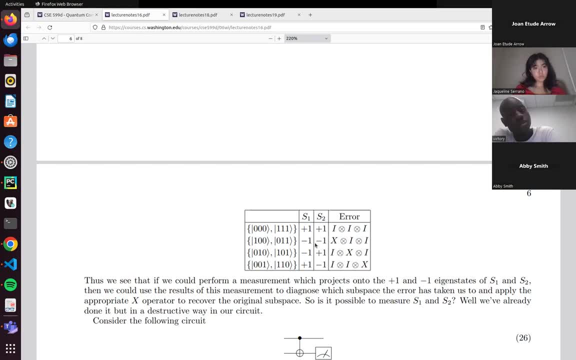 are. you don't want people to make it through who aren't, you know, part of your organization. so this analogy here is: uh, you only want the door to open if, uh, the, the person scans as being part of your organization. so you want some way to detect: is this person or is this quantum state, the state? 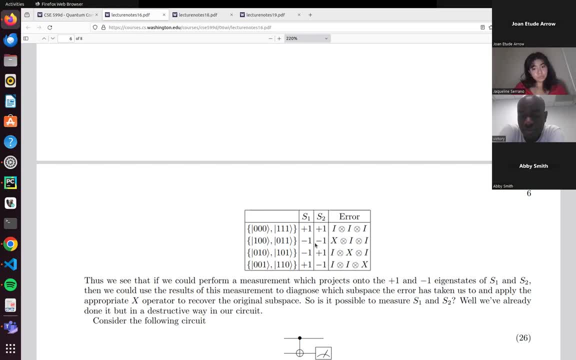 that i think it is. so. these, that's what these syndrome measurements are doing. they're a way to detect if an error has occurred, uh, and if so, ideally where it occurred, so you can fix it. so that that way it's like you: you do this whole quantum calculation, at the very end you get your. 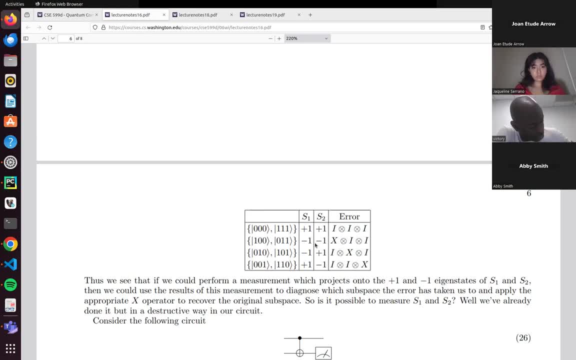 quantum state, but you don't know whether that state is the state you meant to prepare. so what these are doing is they're giving you a way of saying zero or one yes or no. this is the state i meant to prepare and it also. it's also giving you a little bit more information. it's saying it's: 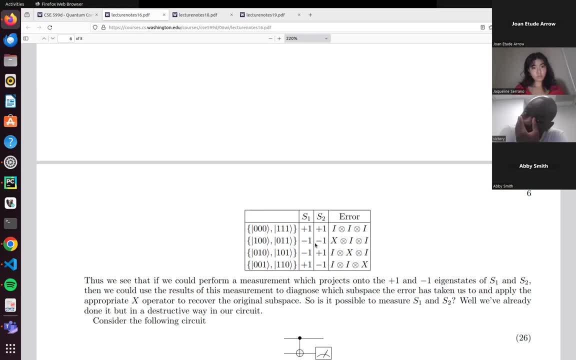 now two bits of information that also encodes: yes, there was an error and i can tell you where it is exactly. um, so the code helper right, say that again, abby. so it's like the code helper to be like: yeah, you have made a mistake. here you go exactly. that's all. that's what. it's entirely. what error. 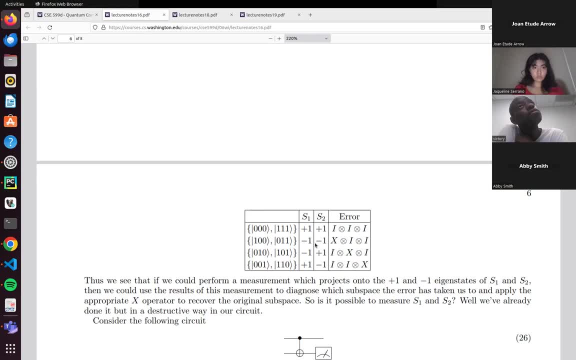 correction is about is is helping um, ensure that you're performing the computation you meant to perform. yep, okay, so, um, yeah, so, uh. so i'd like like a super mark circuit like this would be something that you could do when you're doing like a computational analysis on your computer. 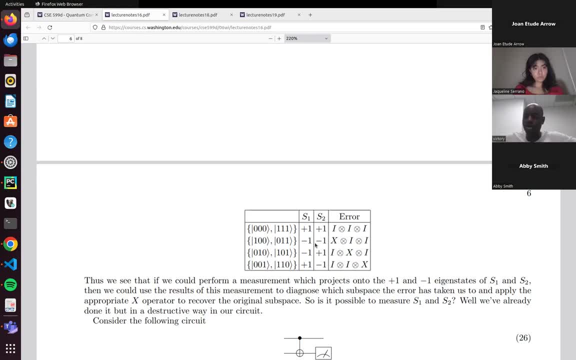 um. so i would like to tell you that, in order for you to perform a computational analysis, um you, this is all done classically. so you have your, you have your logic in your kind of computer, but usually the hour correction is done on a classical computer, in a sense of like you, the. 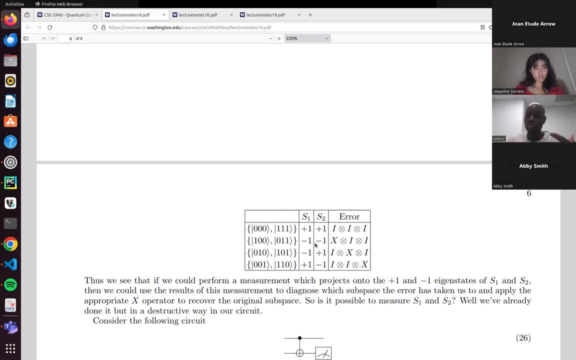 you measure, when you, when you do your measurements, you put your, your syndrome in in like a classical computer and then use a classical program to decide which error action operation to perform. so, for example, if i measured my syndromes and i got these one, uh one one, oh sorry, sorry, zero, zero, um, i would know that there's an x. 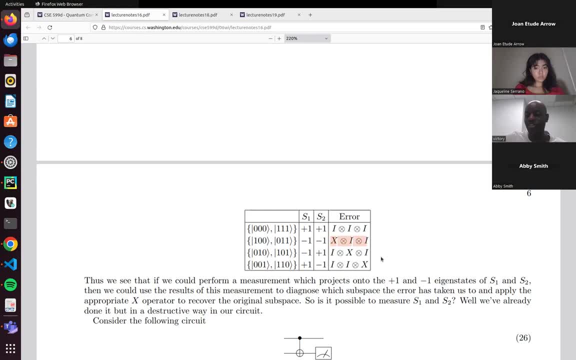 error on my top qubit. so then i would apply an x gate on the top qubit and then that would you know, x and x are an identity, so it'll the x will cancel out with it. the x error will cancel out with the x that i applied to get to cancel it out. that's what the error correction code is, because you'll. 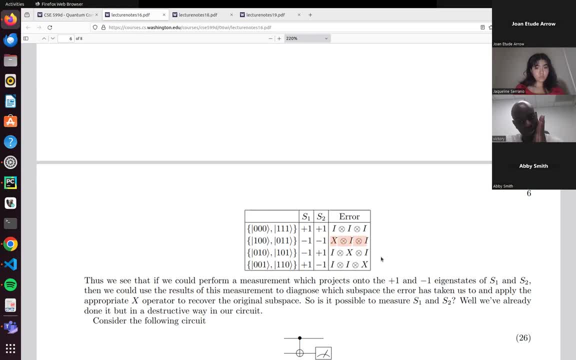 notice, uh, jackie and abby, that the x gate uh uses the identical notation to the bit flip gate, and that's not by accident. the pauli x is identical to a bit flip. it's just a bit flip being deployed in a quantum context. so, uh, that's why victory was just saying: if you find a bit flip, 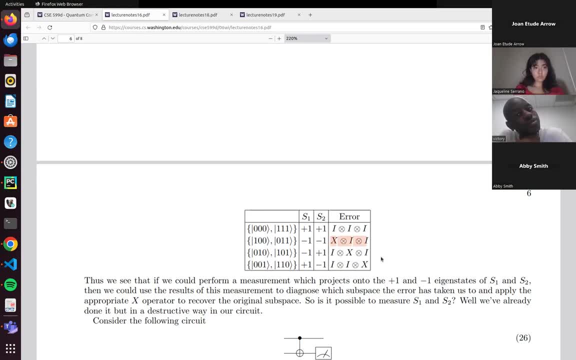 error somewhere, you can just you flip it back. you can apply just another bit flip gate on the correct qubit and that fixes the error that you found. yep, exactly, um, so, yeah, so, uh, that's, that's basically the whole error correction actually. uh, it's just, you have. 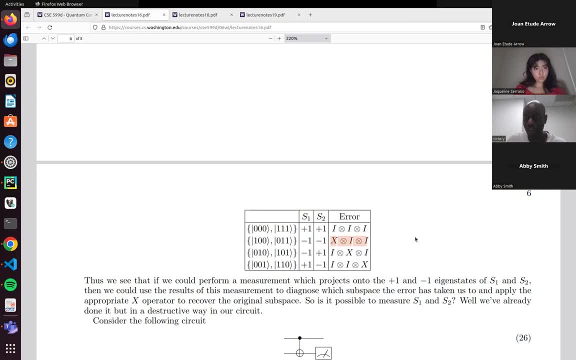 you have uh syndrome, uh qubits that call ancillas, and then you use those ancillas to measure the parity of your qubits and then, based on the measurements you get, you know that tells you which error, and then you can apply um the appropriate operation to cancel out that error and these, these, these codes are all figured out. so 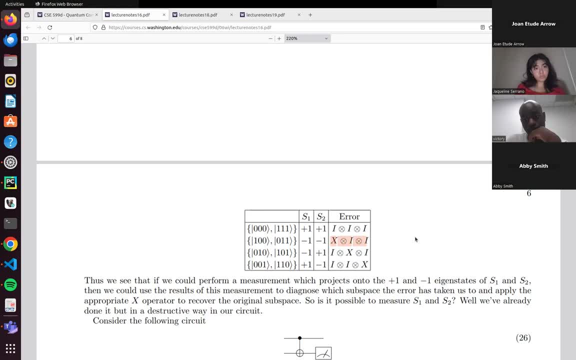 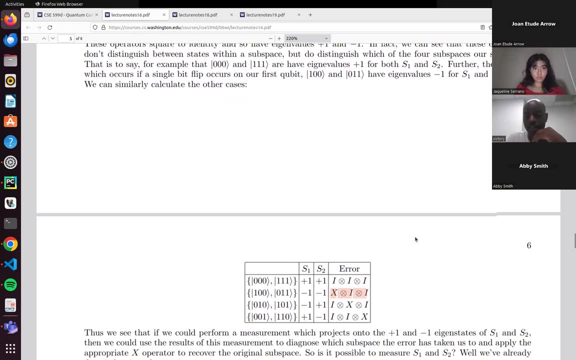 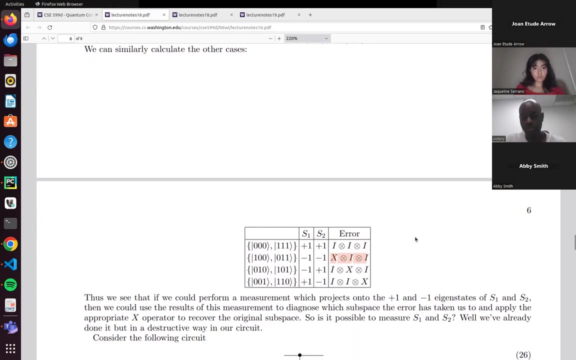 if you know what code, uh, you're using. so this, this is the this. what is the name of this code? victory? say again, are you asking if it's the bit flip code or are you asking if it's like a stabilizer code? yeah, is it just called bit flip code? yeah, yeah, so it detects bit flips. yeah, so if you know. 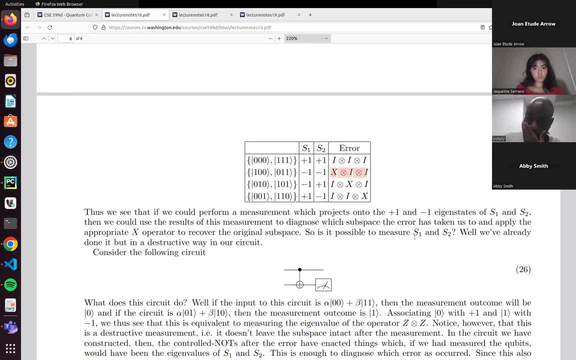 the code that you're using this table of of s1, s2, and you're just like: oh, i see a bit flip error. corresponding to which error? that'll just be in front of you. like you don't have to figure that out, all you have to do is set it up so that you. 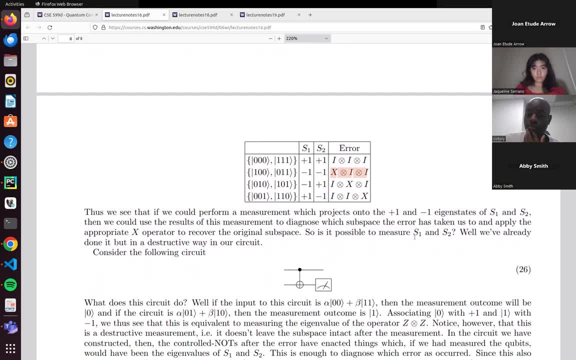 can detect. oh, i see a plus plus or a minus minus or a plus minus, and then you just compare that in your table. oh, that corresponds to a bit flip error on the third qubit, and then you can correct it. um, so really, the, the skills that you'll need, um, if you were working with a code like this, is just the. 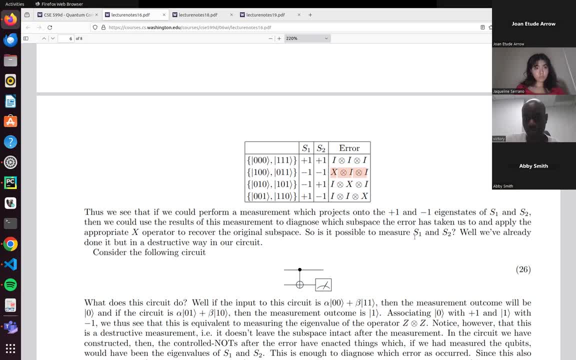 ability to rig up the. the circuit, you know, um, which is going to be core to basically all of the challenges, is just using uh. supermark uses google's quantum package, circ, which is a python based thing. they will have some syntax for how do you do uh um a poly x gate on which qubit, and then you'll just, you know, code it. 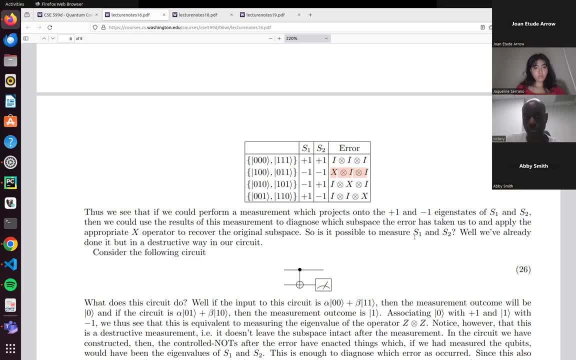 up in such a way that it detects the syndrome and then implements the correct uh gate in the correct spot to fix the error. am i on base there? victory is. that is that kind of what your your challenges are about. i was actually hoping you might like talk us through a couple of them. um, oh, um, oh, okay, yeah, sure, sure, i can, i can. 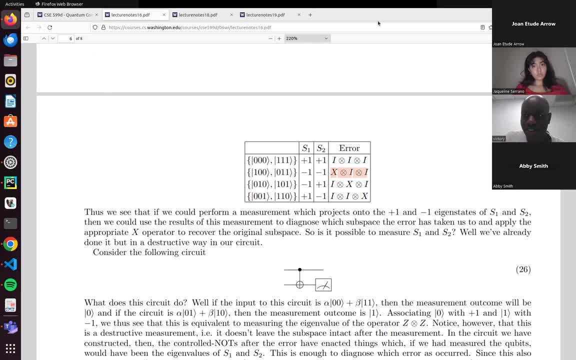 do that. um, if i can, did i ever like bookmark the? i can put the. i can put the link in, okay, please do. thanks also. uh, jackie abby, do you have questions at this juncture while we get the next step set up? no, i do not. okay, and and yeah, for both of you, this is, this is advanced stuff if it's like 99. 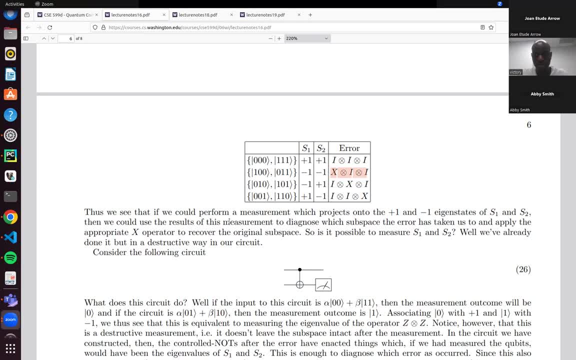 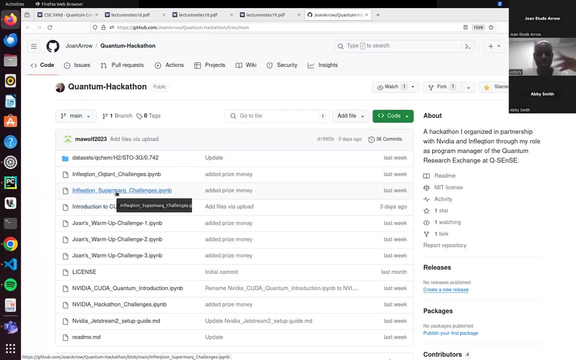 not making sense. don't feel like that's at all on y'all um, and i'll definitely make the um, the notebooks, more. i guess i'll add more meat to it. so it's like i'm over template, because right now it's very empty, so i'll fill it. i'll fill out um parts where- uh, that parts where you don't need. 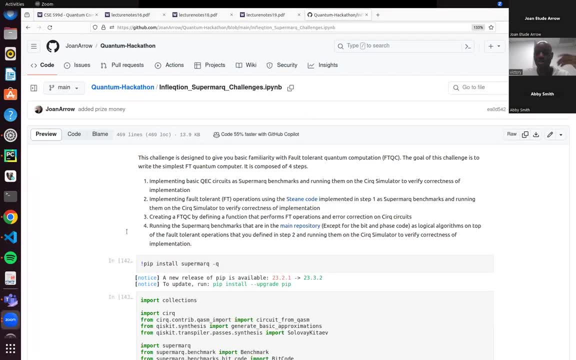 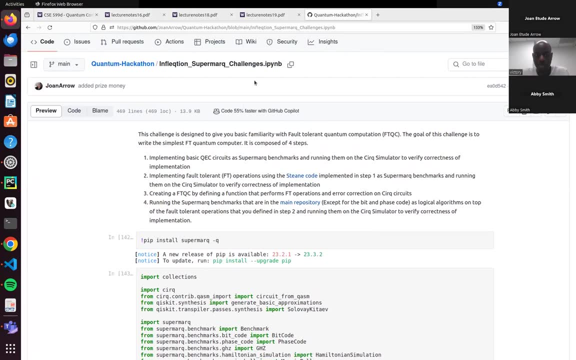 you don't really need to like um to get the general gist of our correction. nice, so this is the supermark challenges. uh, file, that's in the hackathon repo. yep, exactly so. uh, yeah, so the goal of the hackathon is actually to create, you know, a false, tolerant quantum computer, which is another term that we haven't defined yet. 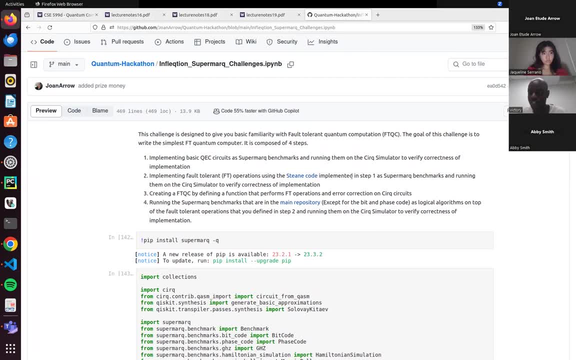 but it's basically just a quantum computer that runs error correction in a way where the errors don't spread out and like just kill your competition. so you can run these error correction protocols, but on quantum memory, so like on just uh, qubits that you're not doing computation on, but when you're actually like performing gates and doing measurements. 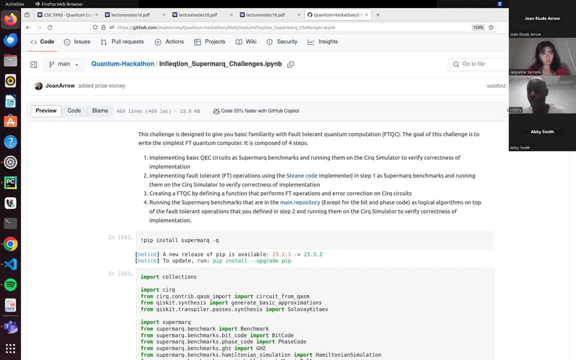 and preparing states, then you, you just running error correction is not enough. you actually need um to do it in a certain you need to run error correction a certain way where it's false, tolerant, and quantum computer is just the ultimate goal of error correction. you've realized a quantum. 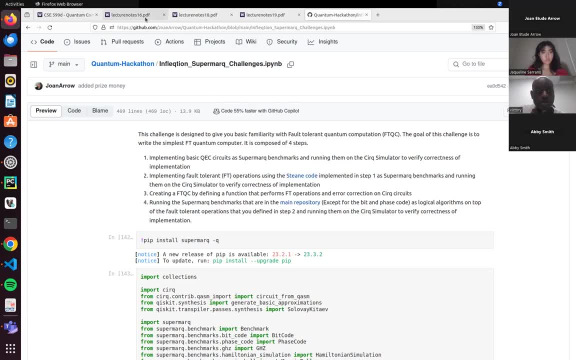 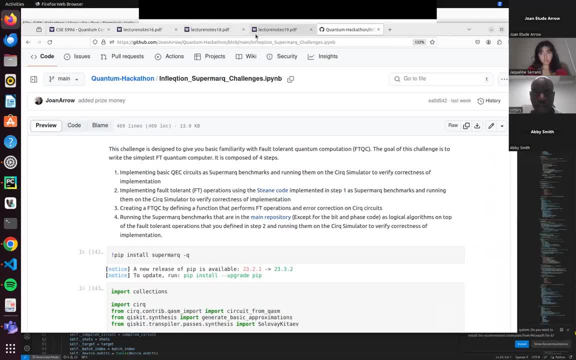 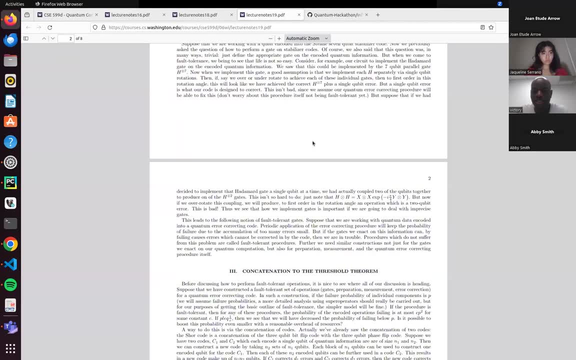 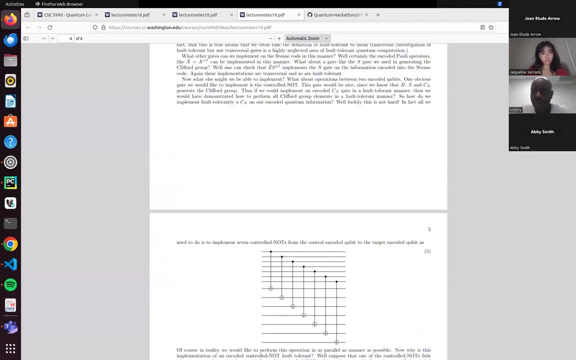 can you okay? uh, so this is actually a lecture. i'll just say that, um, i'm gonna send these as references, but this is just part of like the these last lectures. this is just talking to what a false tolerant competition is and why we care, and everything so, um, anyway, when i go back, uh, so it. 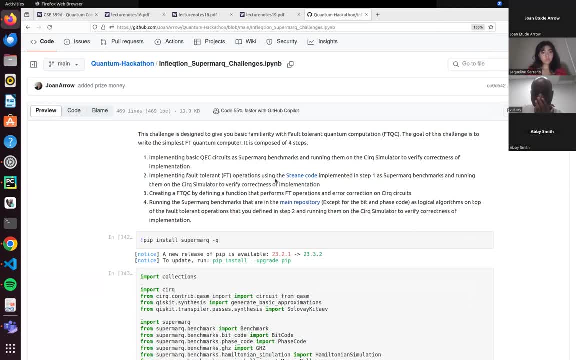 yeah, it'll walk you through. yeah, it'll walk you through. yeah, it'll walk you through. uh. implementing a steam code which is um a. uh implementing a steam code which is um a. uh. implementing a steam code which is um a certain type of error. correcting code. 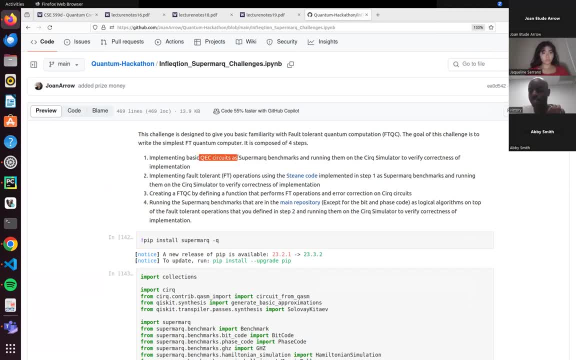 certain type of error correcting code, certain type of error correcting code. and after you, after you've implemented the, and after you, after you've implemented the, and after you, after you've implemented the basic qbc circuit, so um the basic ones. basic qbc circuit: so um the basic ones. 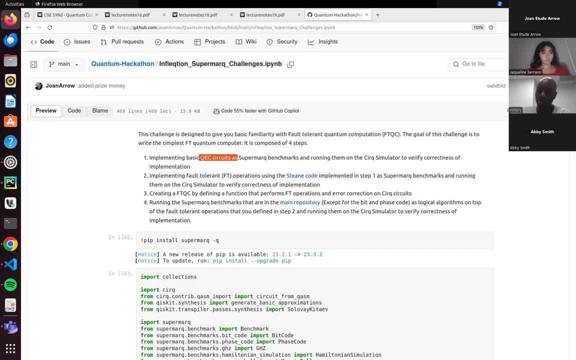 basic qbc circuit. so, um, the basic ones. uh, we just went through the bit flip code. uh, we just went through the bit flip code. uh, we just went through the bit flip code. there's the phase code. there's the phase code. there's the phase code and um, and after that you can just. and um, and after that you can just and um, and after that you can just implement this steam code: um you, i don't implement this steam code. um you, i don't implement this steam code. um you, i don't think i put the. i think i put the show's. think i put the. i think i put the show's. think i put the. i think i put the show's code here, but code here, but code here. but you don't need it. let me see, let me. you don't need it. let me see, let me. 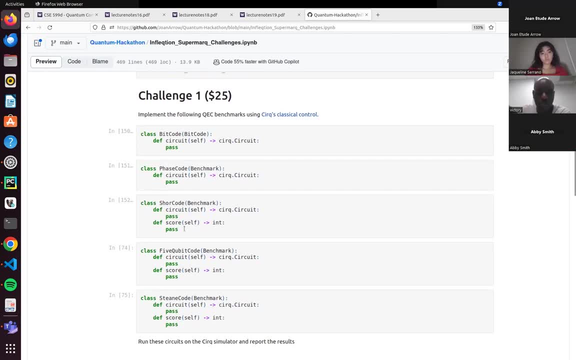 you don't need it. let me see. let me confirm that i put the show's code. confirm that i put the show's code. confirm that i put the show's code. so that, okay, so, um, i'm gonna delete this. so that, okay, so, um, i'm gonna delete this. 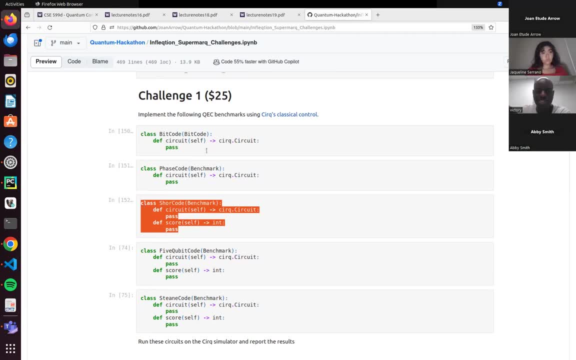 so that okay. so, um, i'm gonna delete this because you don't. you don't need this to, because you don't, you don't need this to, because you don't, you don't need this to get your thing done. these two are just get your thing done. these two are just 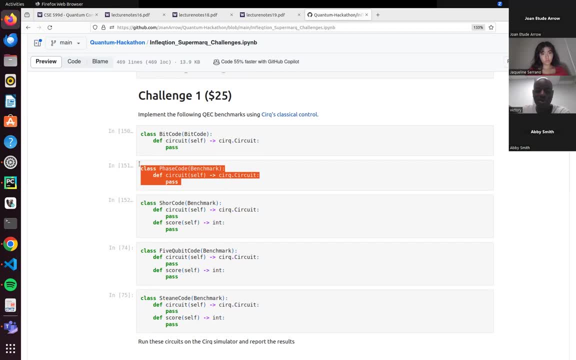 get your thing done. these two are just to like: get the general gist to like. get the general gist to like. get the general gist of what our question is, and then um of what our question is, and then um of what our question is, and then um, these are not needed for for the these are not needed for for the. these are not needed for for the challenge. so i'll delete both of these challenge. so i'll delete both of these challenge. so i'll delete both of these. so you can just implement the steam. so you can just implement the steam. 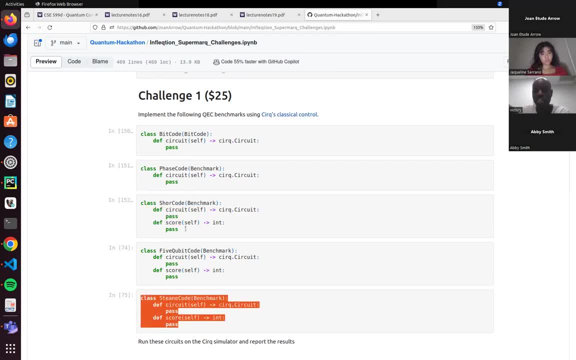 so you can just implement the steam code. but all these are just quantum code. but all these are just quantum code. but all these are just quantum correction codes. uh, shore's code was correction codes. uh, shore's code was correction codes. uh, shore's code was the first error correction code that um. 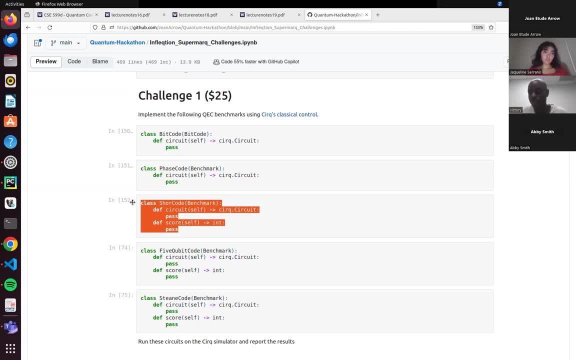 the first error correction code, that um. the first error correction code: that um was invented, so in the 90s, uh, after was invented, so in the 90s, uh, after was invented, so in the 90s, uh, after. shore's algorithm, uh, are you familiar? 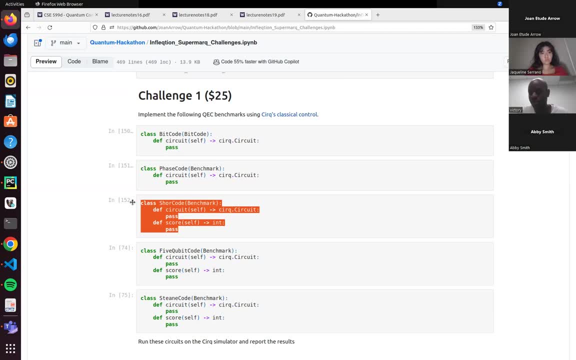 shore's algorithm. uh, are you familiar shore's algorithm? uh, are you familiar with shore's algorithm? we do not know with shore's algorithm, we do not know with shore's algorithm, we do not know what shore's algorithm is okay, so what shore's algorithm is okay, so. 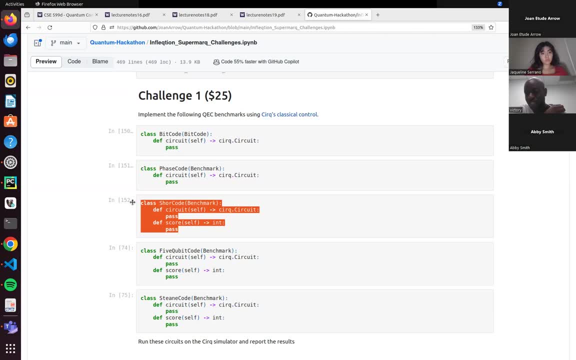 what shore's algorithm is okay. so shore's algorithm is why people are shore's algorithm, is why people are shore's algorithm, is why people are interested in quantum computing, in the interested in quantum computing, in the interested in quantum computing. in the first place, it's um a quantum algorithm. 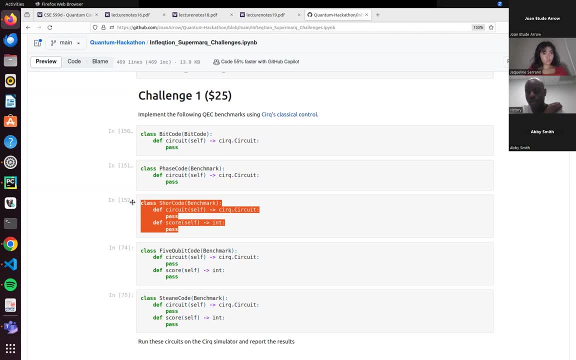 first place it's um a quantum algorithm. first place it's um a quantum algorithm that factors um, that factors um, that factors um. uh, gets the prime factors of numbers, uh, uh, way faster than um. like a way faster than um. like a way faster than um. like a classical computer would. 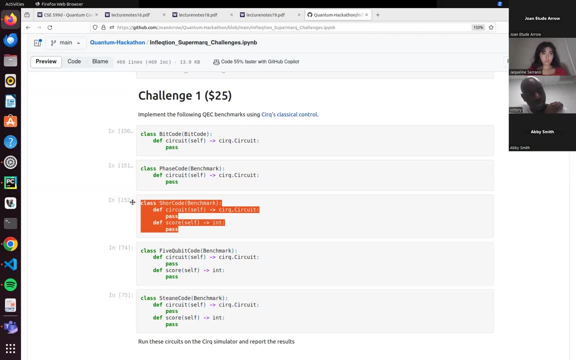 classical computer would. classical computer would it's. it's an algorithm whose only it's. it's an algorithm whose only it's. it's an algorithm whose only application is cyber terrorism. it's uh in in 1995, shore's algorithm. it's uh in in 1995, shore's algorithm. 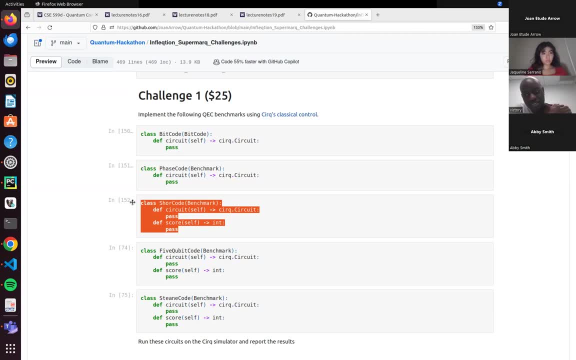 it's uh in. in 1995, shore's algorithm showed that all of the, the entire showed that all of the, the entire showed that all of the, the entire security infrastructure upon which the security infrastructure, upon which the security infrastructure upon which the internet is based, could be vulnerable if. 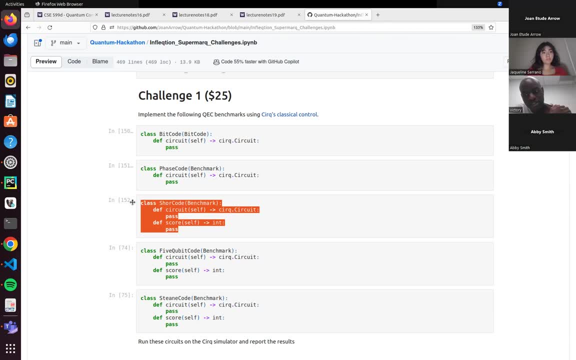 internet is based could be vulnerable. if internet is based could be vulnerable. if a large enough quantum computer were a large enough quantum computer were a large enough quantum computer were built, built, built um. which is why governments are putting um. which is why governments are putting um, which is why governments are putting money into quantum, because they won't. 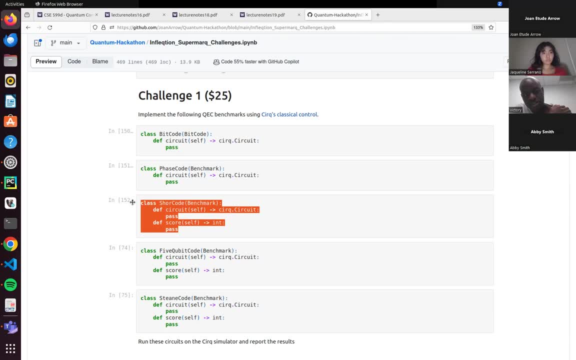 money into quantum because they won't money into quantum because they won't. they're either worried about someone else, they're either worried about someone else. they're either worried about someone else getting that capability, or they want getting that capability, or they want getting that capability, or they want that capability for themselves. it's. 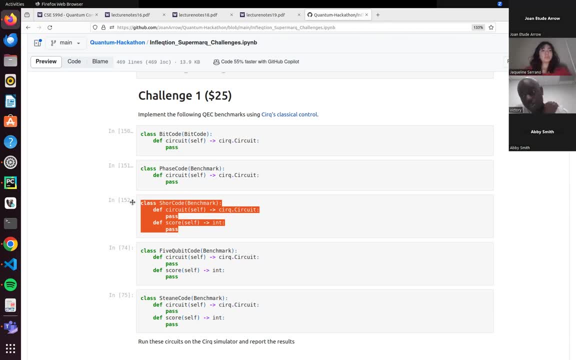 that capability for themselves, it's that capability for themselves, it's peter shore also then also came up with peter shore also then also came up with peter shore also. then also came up with the first example of an error. correcting the first example of an error. correcting the first example of an error. correcting code. 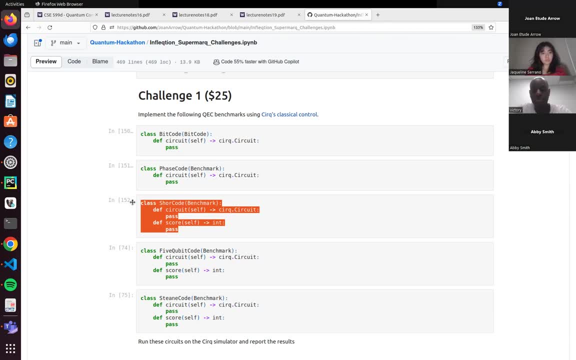 code code: um, um, um, exactly uh, and then so uh. the reason i exactly uh and then so uh, the reason i exactly uh and then so uh. the reason i added this was because um, it's added this, was because um, it's added this, was because, um, it's shore's code is basically a combination. 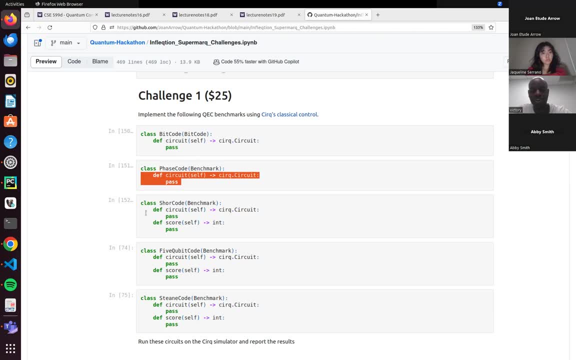 shore's code is basically a combination. shore's code is basically a combination of the bit flip and the phase code, but of the bit flip and the phase code, but of the bit flip and the phase code. but, as i said, it's it's not, it's not relevant. as i said, it's, it's not. it's not relevant. as i said it's it's not. it's not relevant to the challenge, so i'll remove this to the challenge. so i'll remove this to the challenge. so i'll remove this. and the reason i added this one is: 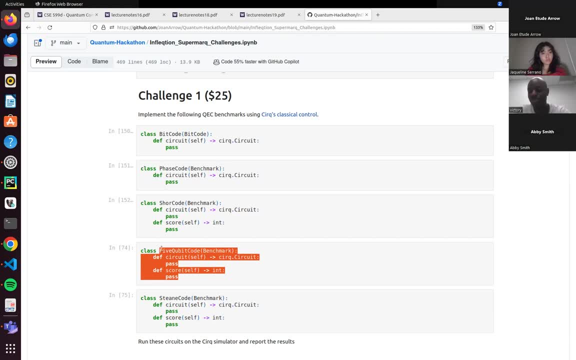 and the reason i added this one is: and the reason i added this one is because it's the smallest. because it's the smallest, because it's the smallest. uh like it's been proven that. if you uh like it's been proven that, if you uh like it's been proven that if you want to correct plus single, uh. like it's been proven that if you want to correct plus single uh. like it's been proven that if you want to correct plus single uh an error on a single uh logical uh. an error on a single uh logical uh. an error on a single uh logical qubit. 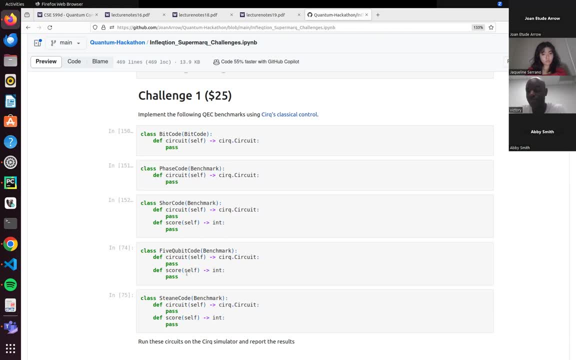 qubit, qubit. uh, the best you can do is is five, five. uh, the best you can do is is five, five. uh, the best you can do is is five, five, five physical qubits, five physical qubits, five physical qubits. um, but i just added these because um, but i just added these because, um, but i just added these because they'll be all they were in the lecture. they'll be all they were in the lecture. they'll be all they were in the lecture. notes and they're just but. notes and they're just but. 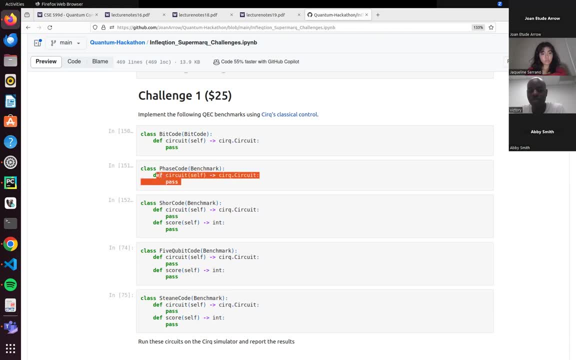 notes and they're just, but um, they're not needed for the challenge, um, they're not needed for the challenge, um, they're not needed for the challenge. so, uh, really the facebook, uh the face. so, uh, really the facebook, uh the face. so, uh, really the facebook, uh the face code and the bit code, if you implement. 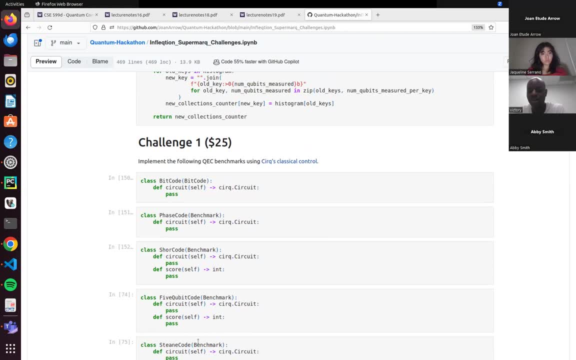 code and the bit code. if you implement code and the bit code, if you implement those, you can easily implement the this. those you can easily implement the this. those. you can easily implement the this team code, because, um um you'll you'll team code, because um, um you'll you'll. 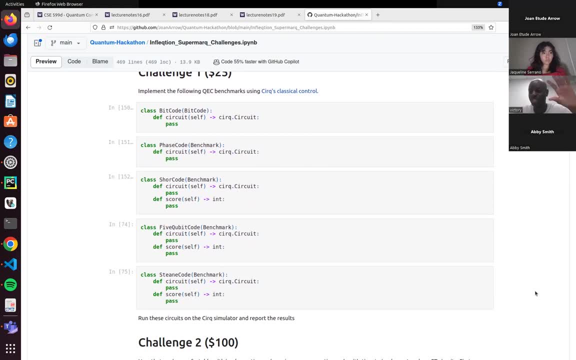 team code because, um, um, you'll, you'll understand, like the gist of how to, how understand, like the gist of how to, how understand, like the gist of how to how to measure stabilizers, which is to measure stabilizers, which is to measure stabilizers, which is basically how to measure. 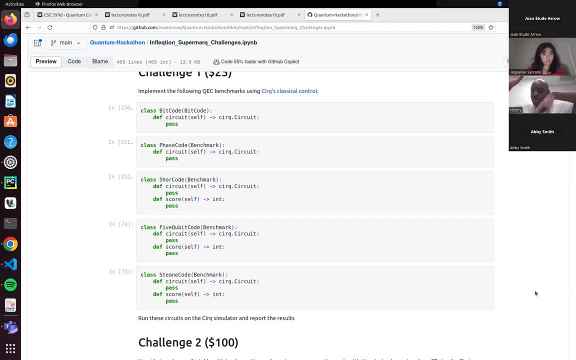 basically, how to measure. basically, how to measure, uh the how to use your ancillars to uh the how to use your ancillars to uh the how to use your ancillars to measure, um, the syndromes of your, of your measure, um, the syndromes of your, of your. 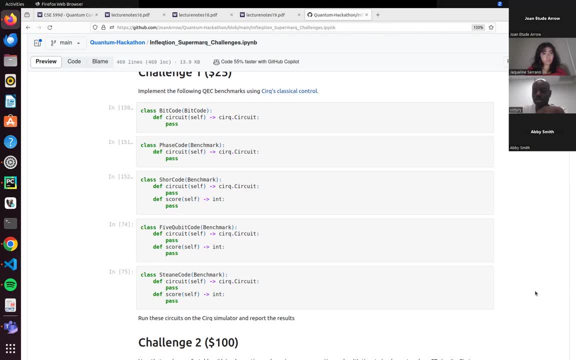 measure um the syndromes of your, of your logical cubit, logical cubit, logical cubit. so victory that the bit code in that box, so victory that the bit code in that box, so victory that the bit code in that box is the same as what we just saw in the. 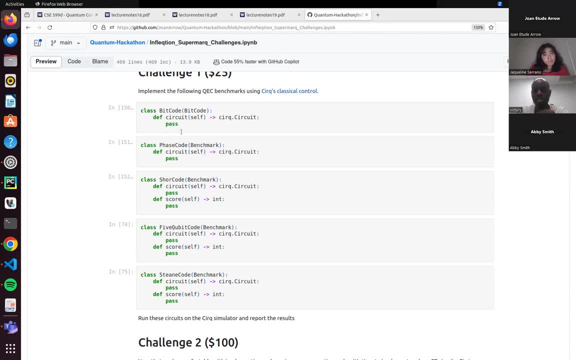 is the same as what we just saw in the is the same as what we just saw in the example. you were sure: yeah, yeah, yeah example. you were sure: yeah, yeah, yeah example. you were sure, yeah, yeah, yeah, exactly so the bit code is detecting if. exactly so, the bit code is detecting if. 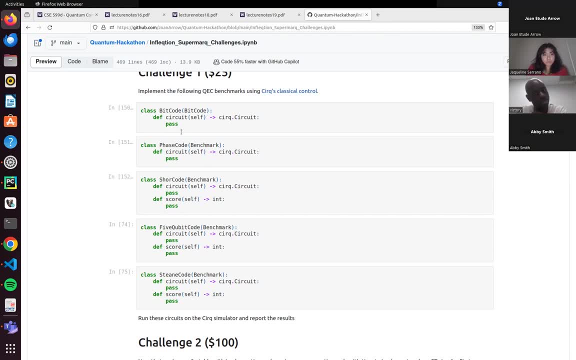 exactly so. the bit code is detecting if a bit flip happened, a bit flip happened, a bit flip happened, and then phase code- we haven't talked, and then phase code, we haven't talked, and then phase code. we haven't talked about it too much, but the so the bit bit. 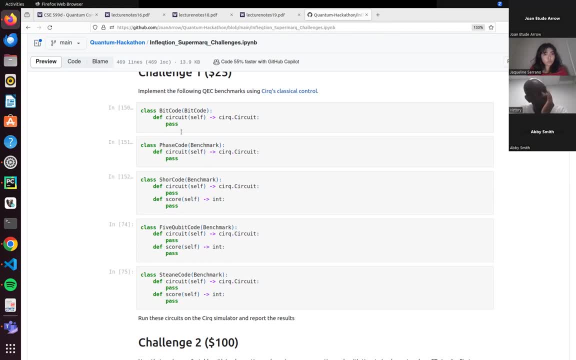 about it too much, but the so the bit bit about it too much, but the so the bit bit. flip code is about detecting. if an flip code is about detecting, if an flip code is about detecting, if an unexpected pauli x, unexpected pauli x, unexpected pauli x- occurred, and the phase code, i'm guessing. 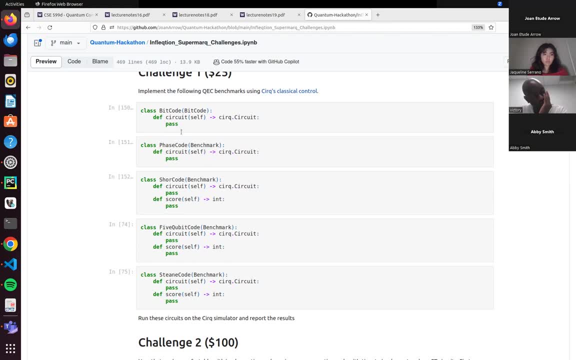 occurred and the phase code i'm guessing occurred and the phase code i'm guessing is detecting if an unexpected pauli z is detecting, if an unexpected pauli z is detecting, if an unexpected pauli z occurred exactly, occurred exactly, occurred exactly um. and then all three of these, all 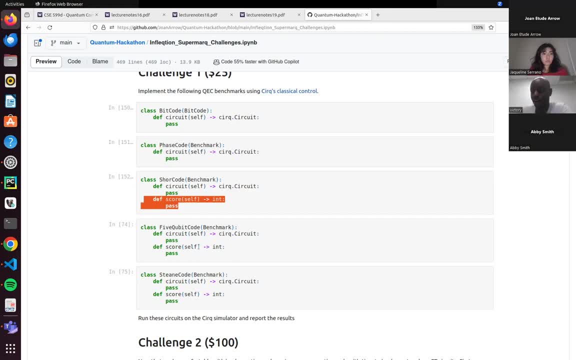 um and then all three of these. all um and then all three of these. all three of these detect if either a three of these detect, if either a three of these detect, if either a bit uh error occurred or a phase error, bit uh error occurred or a phase error. 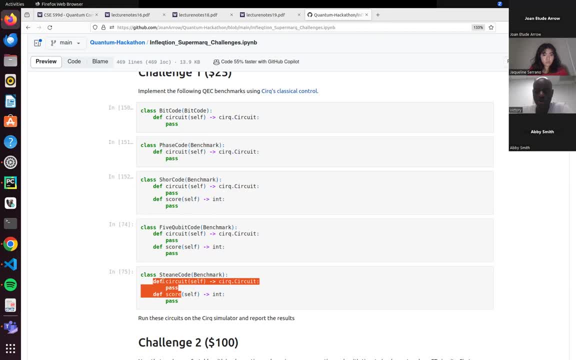 bit uh error occurred or a phase error? uh yeah, all these three like shows code. uh yeah, all these three like shows code. uh yeah, all these three like shows code. five. cubic code and steam code are both five. cubic code and steam code are both five. cubic code and steam code are both all three. detect both of them, right it? 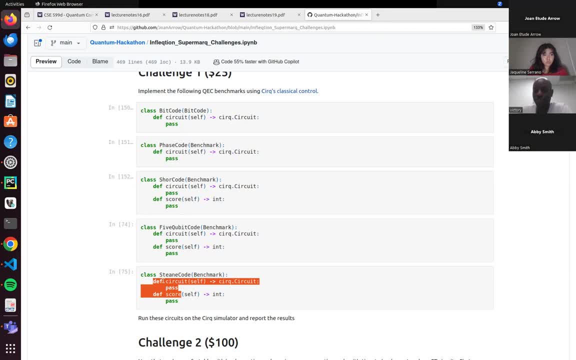 all three. detect both of them. right it. all three detect both of them right. it. detects whether or not a bit flip occurred. detects whether or not a bit flip occurred. detects whether or not a bit flip occurred or a phase code and it corrects for both. or a phase code and it corrects for both. 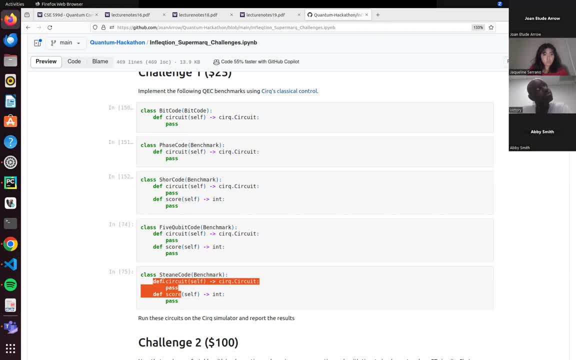 or a phase code, and it corrects for both of them, of them, of them. so then the. the challenge is um, the. so then the. the challenge is um, the. so then the. the challenge is um the. students need to write, students need to write. students need to write a program that implements the bit flip. 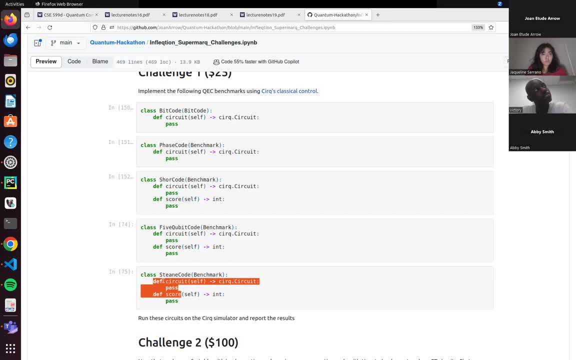 a program that implements the bit flip, a program that implements the bit flip and the phase code and the phase code and the phase code and then use those as a subroutine to, and then use those as a subroutine to, and then use those as a subroutine to construct the. 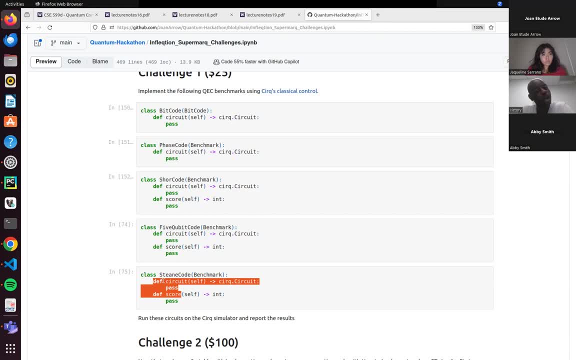 construct the construct, the five qubit and the steam code. or just five qubit and the steam code, or just five qubit and the steam code, or just the steam code, the steam code, the steam code. uh, so, uh, uh, so, uh, uh, so uh. you're cutting the shore code, right? yeah? 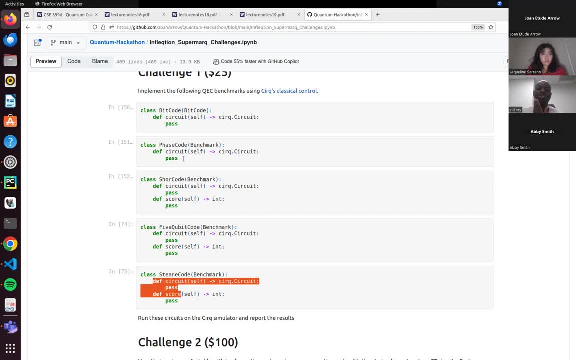 you're cutting the shore code right. yeah, you're cutting the shore code right. yeah, yeah, they, they, they, yeah, they, they, they, yeah, they, they they. what i was thinking was: uh, they would use what i was thinking was: uh, they would use what i was thinking was: uh, they would use the phase code and the bit code to. 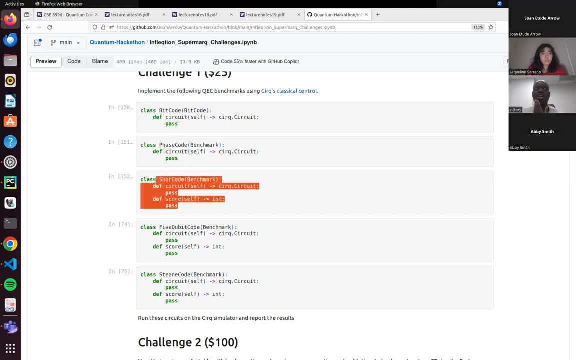 the phase code and the bit code to the phase code and the bit code to construct the shows, because that's how construct the shows, because that's how construct the shows, because that's how it's done. okay, but that's um, it's done okay, but that's um. 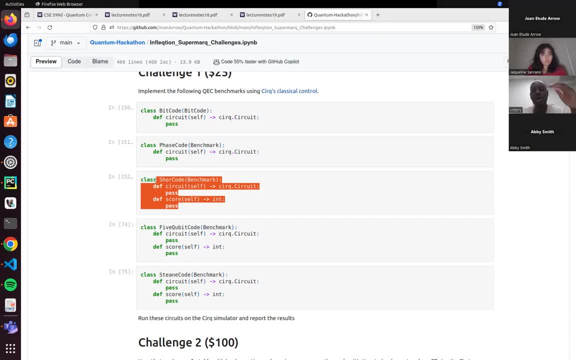 it's done, okay, but that's um, but uh, i uh, but uh, i uh, but uh, i uh. now that i think about it, i think i might, now that i think about it, i think i might, now that i think about it, i think i might just like do a whole. i put out like a: 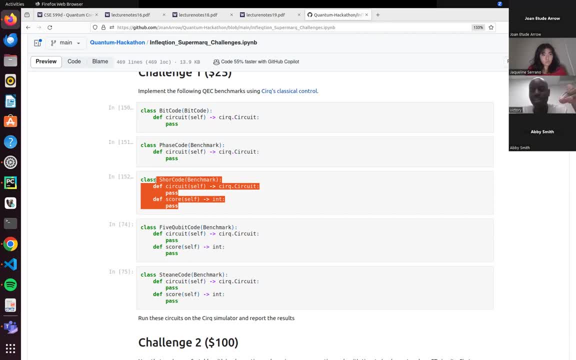 just like: do a whole, i put out like a. just like do a whole, i put out like a really quick summary on like just um really quick summary on like just um really quick summary on like just um: stabilize, like, just just say like oh. stabilize, like, just just say like oh. 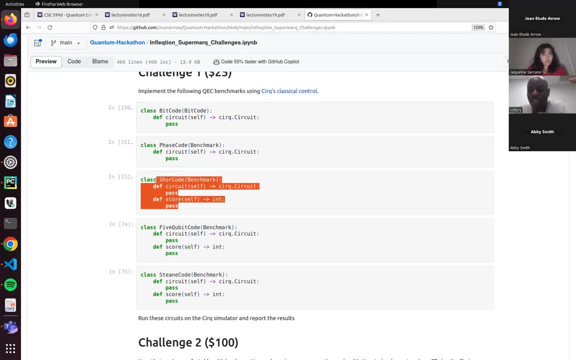 stabilize, like just just say like: oh, these are the stabilizers of the steam, these are the stabilizers of the steam, these are the stabilizers of the steam code, and then it would just be easy to code, and then it would just be easy to code, and then it would just be easy to implement once. 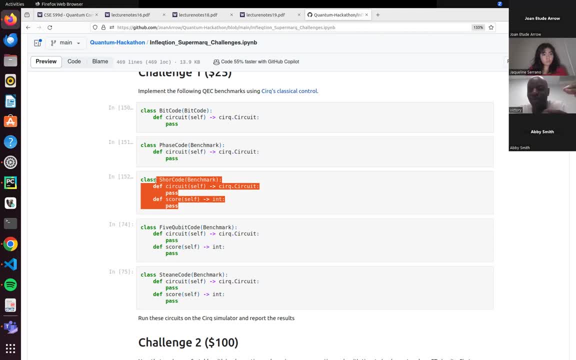 implement once, implement once. uh, i give a quick summary of what uh. i give a quick summary of what uh. i give a quick summary of what stabilizer error correction is. because i stabilizer error correction is because i stabilizer error correction is because i think once, once, i just explain like oh, think once, once i just explain like: oh, think once once. i just explain like: oh, yeah, you're measuring these stabilizers. yeah, you're measuring these stabilizers. yeah, you're measuring these stabilizers. then you don't, you don't really need, then you don't, you don't really need. 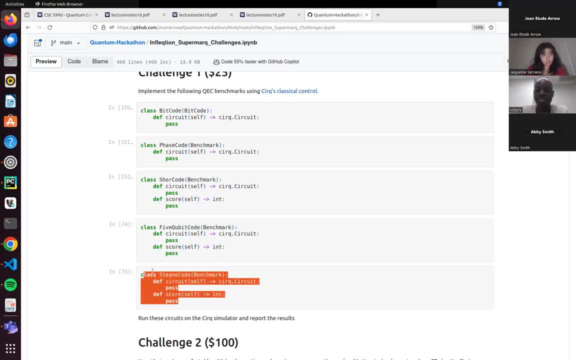 then you don't, you don't really need these two to like to like implement this, these two to like to like implement this, these two to like implement this steam code, steam code, steam code, great, great, great, uh. and so now you, now that you have an uh, and so now you, now that you have an, 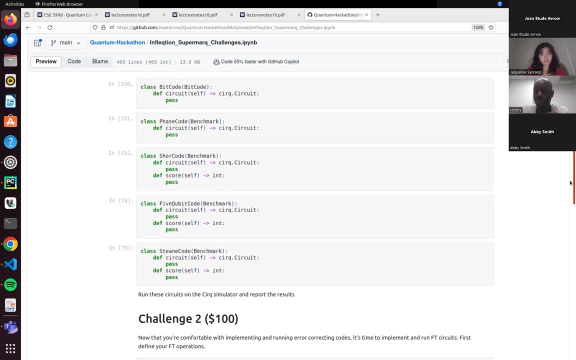 uh, and so now you, now that you have an error correcting code that collect, error correcting code that collect error correcting code that collect corrects, both corrects, both corrects, both face whip and um and bed flips using face whip and um and bed flips using face whip and um and bed flips using the steam code. 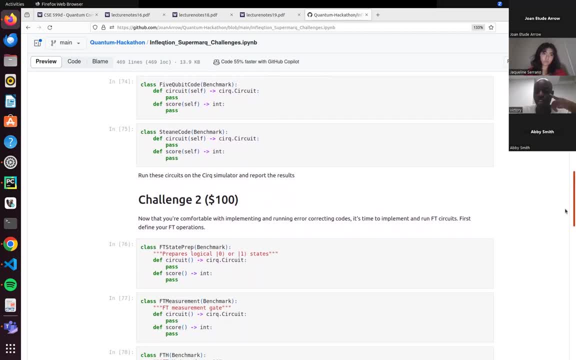 the steam code, the steam code, then you can um make your uh your. then you can um make your uh your. then you can um make your uh your computer fault tolerant, so to make your computer fault tolerant, so to make your computer fault tolerant. so to make your computer fault tolerant, you need: 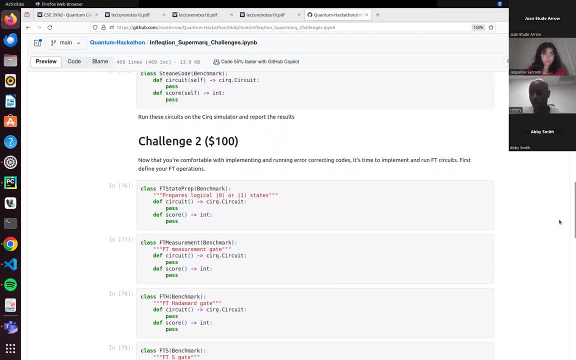 computer fault tolerant. you need computer fault tolerant, you need to basically. so uh are we talking about to basically. so uh are we talking about to basically. so uh are we talking about. we know about gates, right, we know about gates right, we know about gates right. yeah, we've talked to the. i mean, i haven't. 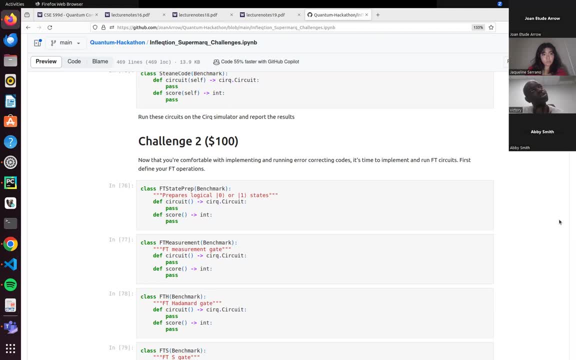 yeah, we've talked to the. i mean i haven't. yeah, we've talked to the. i mean i haven't talked about universality, but we talked about universality, but we talked about universality, but we, we've already established a set of gates. we've already established a set of gates. 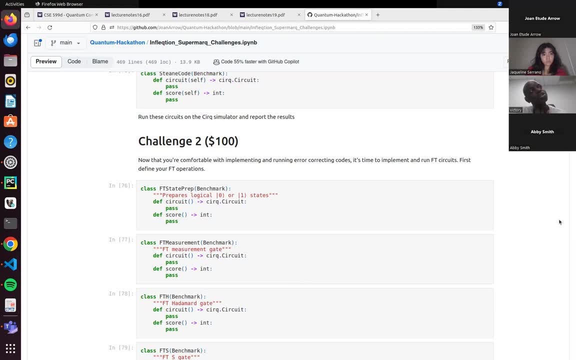 we've already established a set of gates that gets you there. that gets you there. that gets you there. so we talked about x, y and z rotations. so we talked about x, y and z rotations. so we talked about x, y and z rotations by arbitrary angles and the control, not 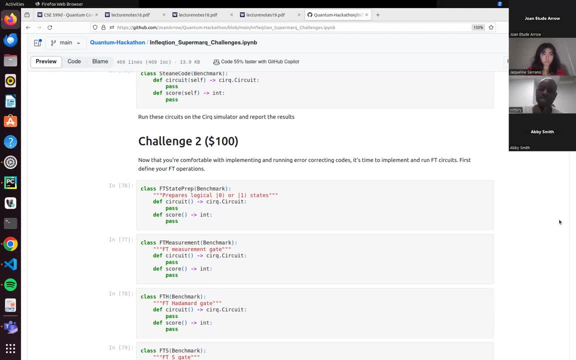 by arbitrary angles, and the control not by arbitrary angles, and the control not gate, gate, gate. and i get that gets you there. oh, and i get that gets you there. oh, and i get that gets you there. oh, perfect, so, perfect, so, perfect. so, jackie and abby, when we're talking about 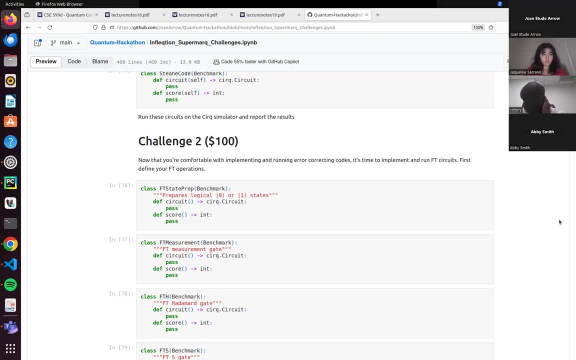 jackie and abby. when we're talking about jackie and abby, when we're talking about a universal quantum computer, we're just a universal quantum computer, we're just a universal quantum computer. we're just basically saying, basically saying, basically saying: what is the minimum set of basic? 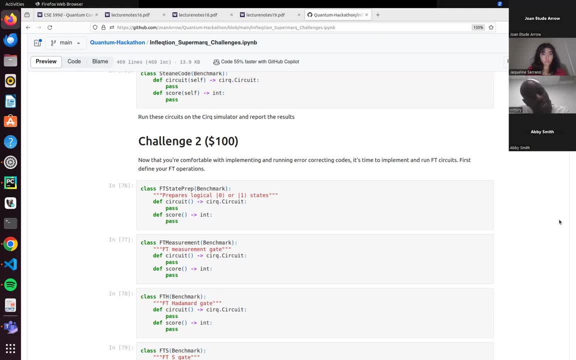 what is the minimum set of basic? what is the minimum set of basic operations? i need to build every operations. i need to build every operations. i need to build every possible possible possible quantum circuit, just in the same way we quantum circuit, just in the same way we. 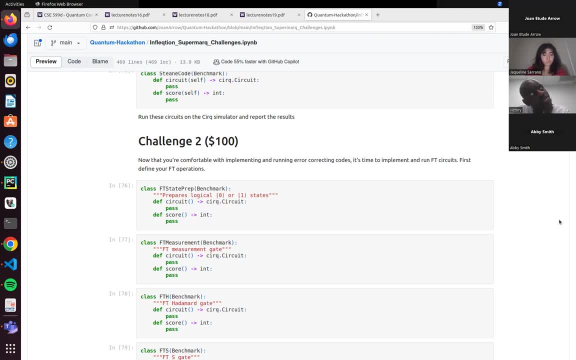 quantum circuit, just in the same way we talked about how, talked about how talked about how uh the uh control, not uh the uh control, not uh the uh control, not um the x or and the and gate were the um, the and gate were the um, the and gate were the basic logic gates that you need for. 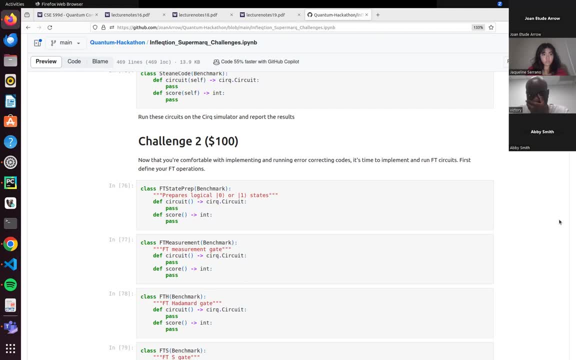 basic logic gates that you need for basic logic gates, that you need for classical computation, classical computation, classical computation. the set of quantum gates you need for the set of quantum gates you need for the set of quantum gates you need for universal quantum computation, are universal quantum computation. are. 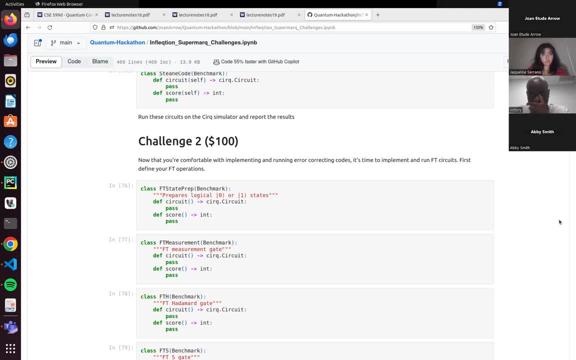 universal quantum computation are there you could. there's a bunch of there you could. there's a bunch of there you could. there's a bunch of different ways you could set them up, but different ways you could set them up. but different ways you could set them up, but the way we've set them up is. 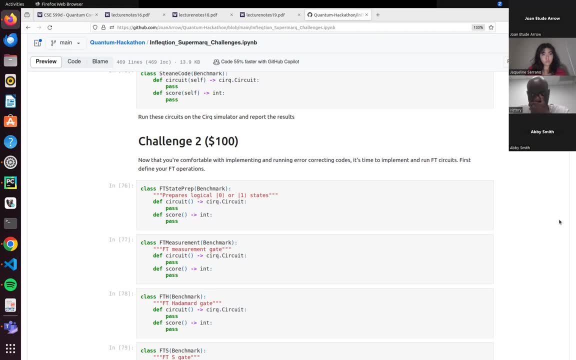 the way we've set them up is the way we've set them up is: you need your three uh block sphere. you need your three uh block sphere. you need your three uh block sphere. rotations x, y and z rotations by any. rotations x, y and z rotations by any. 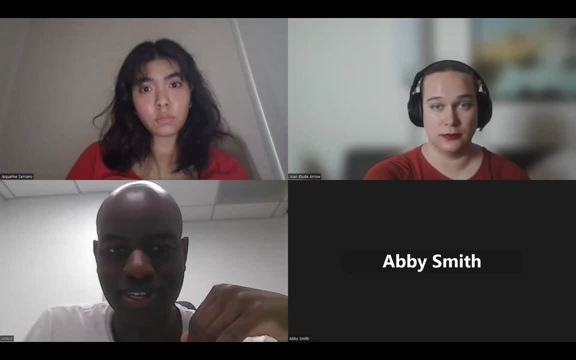 rotations x, y and z rotations by any of this call. like this call again, just of this call. like this call again, just of this call. like this call again, just to like talk to people through this uh. to like talk to people through this, uh. to like talk to people through this uh. so if there's any way we can organize, 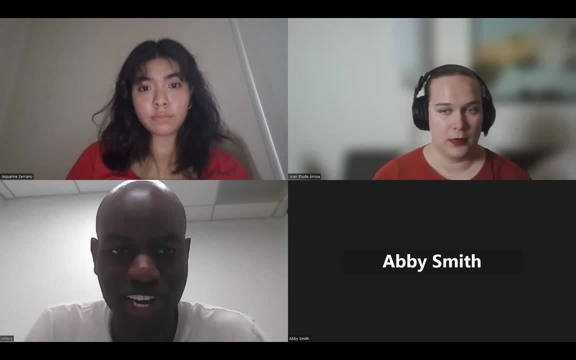 so if there's any way we can organize, so if there's any way we can organize another, another, another call similar to this, where i just like call similar to this, where i just like call similar to this, where i just like walk people through this challenge and 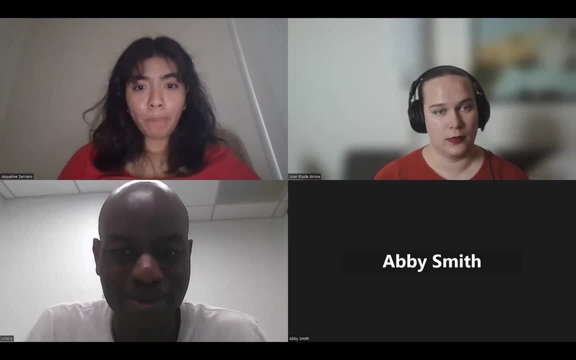 walk people through this challenge and walk people through this challenge and um anytime we run into something, we um. anytime we run into something, we um. anytime we run into something we haven't defined, we can give a quick haven't defined. we can give a quick haven't defined. we can give a quick summary of it and everything. 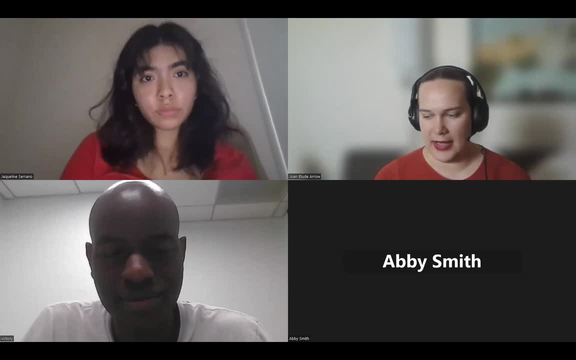 summary of it and everything. summary of it and everything. yeah, i think this is, i think this is good. yeah, i think this is. i think this is good. yeah, i think this is. i think this is good, um, um, um, i, i actually think, like in the larger 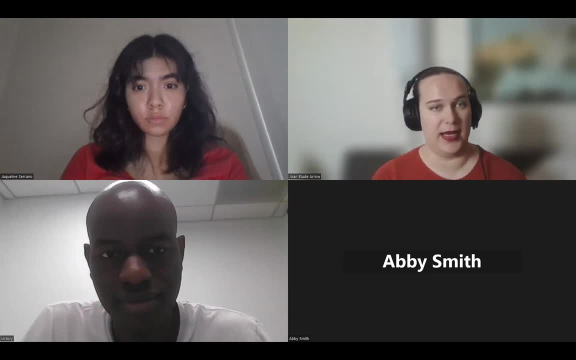 i, i actually think, like in the larger i, i actually think like in the larger scale of things, um, scale of things, um scale of things, um, it'll be better to set up more regular. it'll be better to set up more regular, it'll be better to set up more regular meetings for everybody, because, just you, 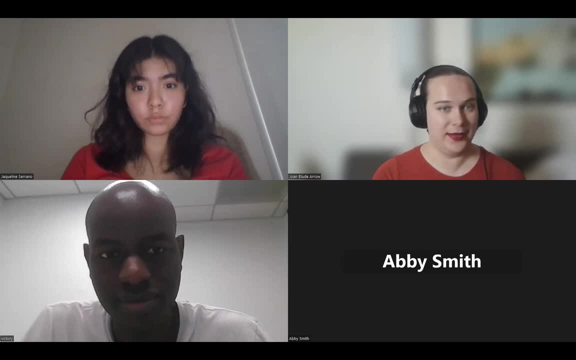 meetings for everybody because just you. meetings for everybody, because just you know the this, know the, this know the this hackathon was two weeks long and this is hackathon was two weeks long and this is hackathon was two weeks long and this is week one like. 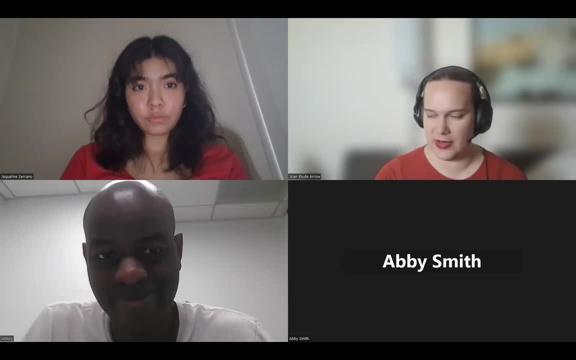 week one like week one, like time where time is rather short. i wish time where time is rather short. i wish time where time is rather short. i wish i wish there had been a little bit more. i wish there had been a little bit more. i wish there had been a little bit more time. but the 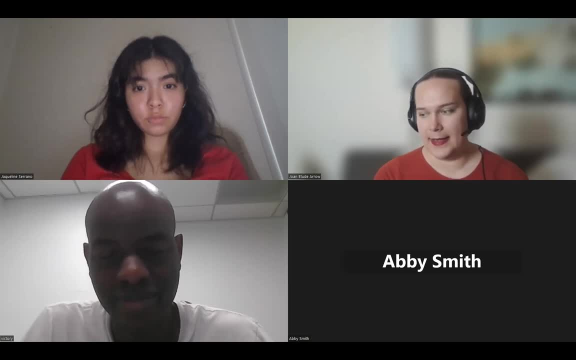 time, but the time, but the the calendar of the qrx is quite full. but the calendar of the qrx is quite full. but the calendar of the qrx is quite full. but, um, the way i've been kind of hoping, um, the way i've been kind of hoping. 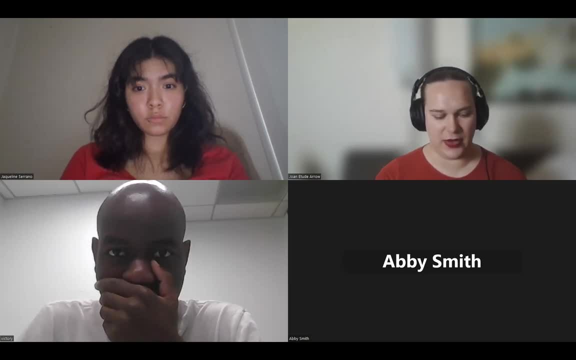 um, the way i've been kind of hoping to have this set up, victory is to have this set up. victory is to have this set up. victory is uh to have you connected with everybody. uh to have you connected with everybody. uh to have you connected with everybody. uh like give, i'm gonna give them your. 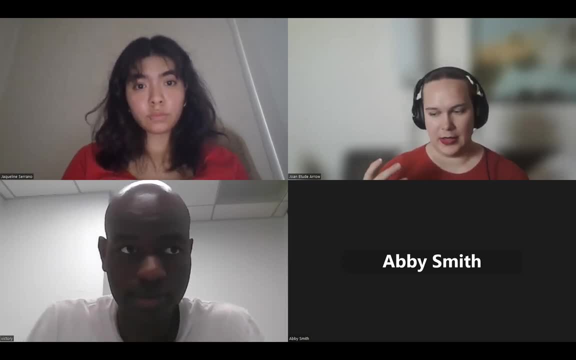 uh like give, i'm gonna give them your. uh like give, i'm gonna give them your email. basically, email basically, email basically, and then um, i'm having, and then um, i'm having and then um, i'm having, uh, the hackathon team members pick, uh, the hackathon team members pick. 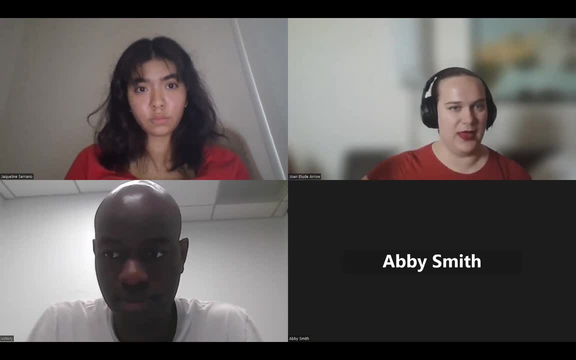 uh, the hackathon team members pick challenges that they want to work on, challenges that they want to work on, challenges that they want to work on, and then they have a point person who, and then they have a point person who, and then they have a point person who they can talk to, who can help them with. 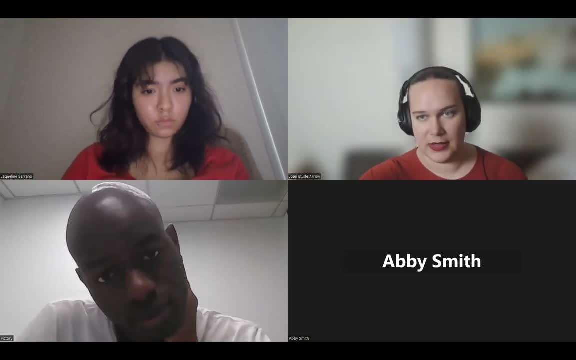 they can talk to, who can help them with. they can talk to who can help them with those specific challenges, those specific challenges, those specific challenges: um, um, um, um, um, um. so what, what i think i'll do at the follow-up? what, what i think i'll do at the follow-up? 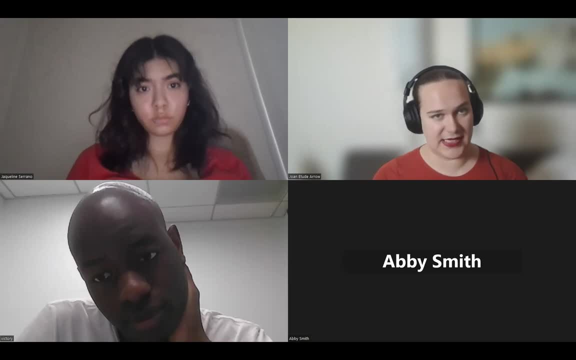 what? what i think i'll do at the follow-up for this meeting is i'll send that email for this meeting. is i'll send that email for this meeting is? i'll send that email. all of you will have victory's email. all of you will have victory's email. 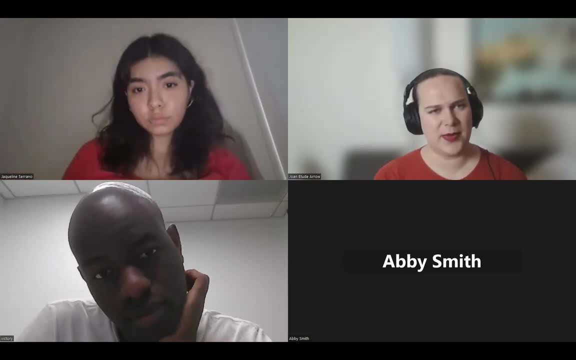 all of you will have victory's email. you'll have the emails of. you'll have the emails of. you'll have the emails of of uh. is isaac still participating of? uh? is isaac still participating of? uh? is isaac still participating? jackie and abby: 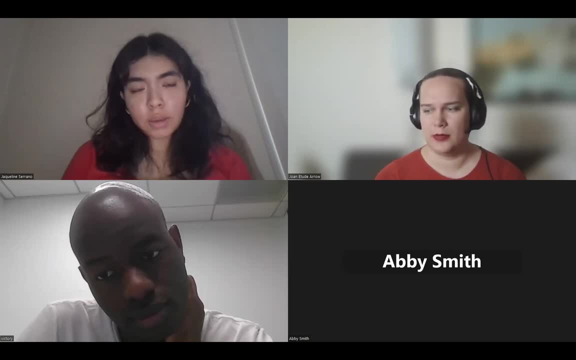 i think so, um, he's been asking me to. i think so, um, he's been asking me to. i think so, um he's been asking me to like, like, like, meet up so that we can kind of work on. meet up so that we can kind of work on. 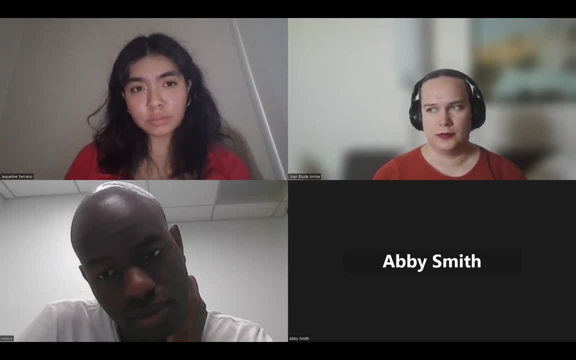 meet up so that we can kind of work on it together, it together, it together. but i'm not sure which challenge he's. but i'm not sure which challenge he's, but i'm not sure which challenge he's gonna, gonna, gonna do. i'll cc him um, but so i'll include. 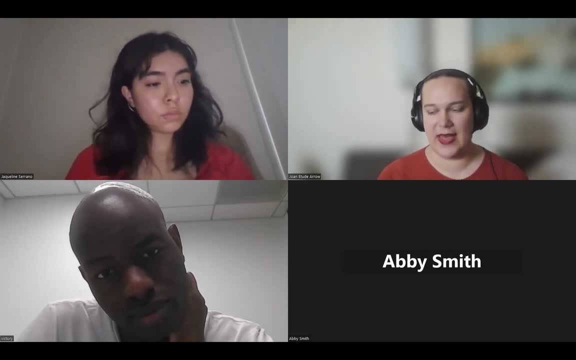 do i'll cc him um, but so i'll include. do i'll cc him um, but so i'll include the students who are still participating, the students who are still participating, the students who are still participating, and then um in that email we can set up, and then um in that email we can set up. 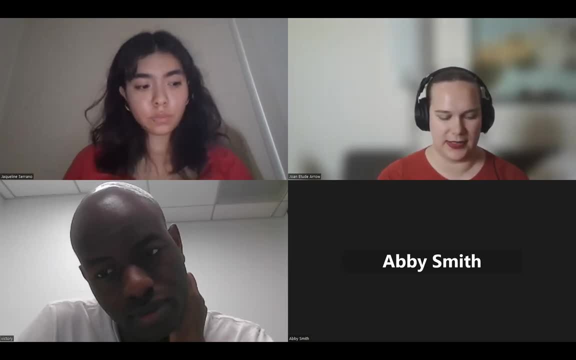 and then um in that email. we can set up a time a time a time. students need to. if students are trying, students need to. if students are trying, students need to. if students are trying to tackle the, to tackle the, to tackle the, the supermark challenges, we can set up. 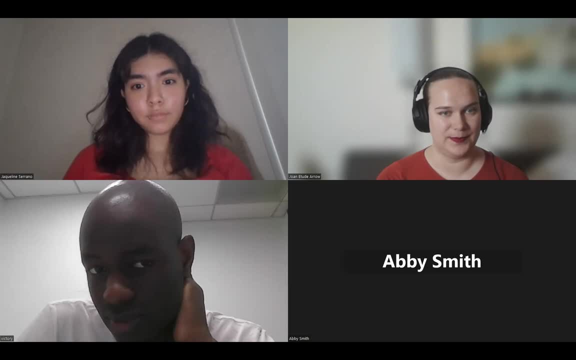 the supermark challenges. we can set up the supermark challenges. we can set up another time early next week, to another time early next week, to another time early next week to to have another meeting like this. okay, to have another meeting like this. okay, to have another meeting like this. okay, perfect, yeah, this is definitely a. 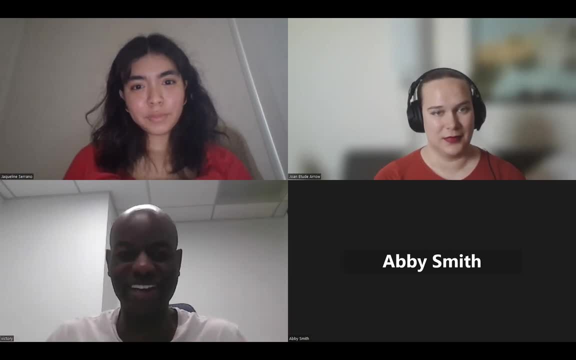 perfect. yeah, this is definitely a perfect. yeah, this is definitely a depend depend type type thing, so, but if depend depend type type thing, so, but if depend depend type type thing, so, but if you get this, you'll get, you'll get this. you get this, you'll get, you'll get this. 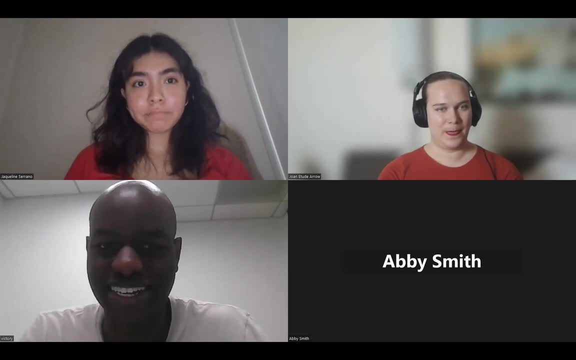 you get this, you'll get, you'll get this is basically all is basically, all is basically all the whole thing. yeah, this is basically what the whole thing. yeah, this is basically what the whole thing. yeah, this is basically what our question is. our question is, our question is yeah, and and again, i, and i've told the 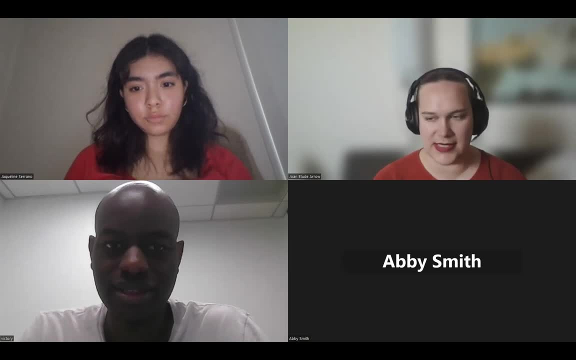 yeah and and again. i and i've told the yeah and and again. i and i've told the students this like the students, this like the students, this like the. my only hope for this project program is my only hope for this project program is my only hope for this project program is even is. i don't care if a student even is. i don't care if a student even is. i don't care if a student solves any of the chat. if none of the solves any of the chat, if none of the solves any of the chat, if none of the challenges get solved, challenges get solved. 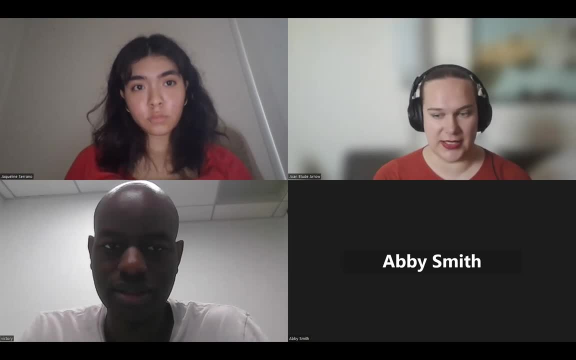 challenges get solved. i won't be um disappointed the main. i won't be um disappointed the main. i won't be um disappointed. the main goal is just to like give students the goal is just to like give students the goal is just to like give students the chance to interact with people like you. 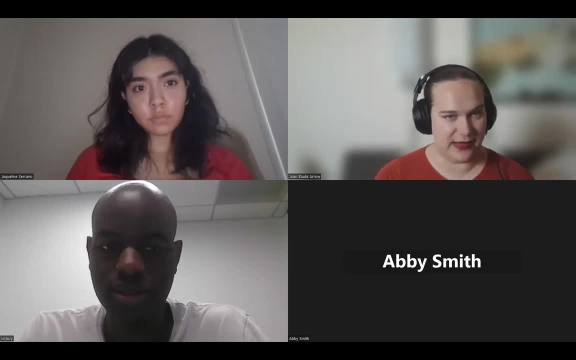 chance to interact with people like you. chance to interact with people like you who are working at quantum companies, who are working at quantum companies, who are working at quantum companies, giving them the chance to challenge, giving them the chance to challenge, giving them the chance to challenge themselves with some interesting 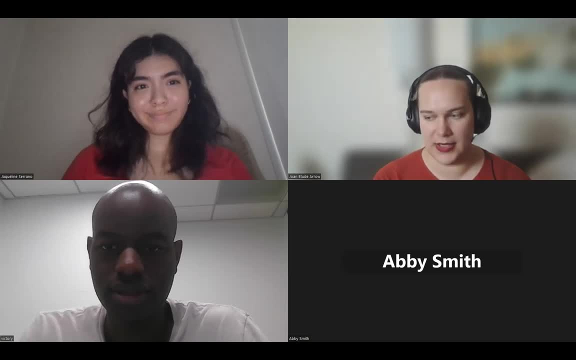 themselves with some interesting themselves, with some interesting problems, and you know who knows um problems and you know who knows um problems and you know who knows um. trying to get students connected to trying to get students connected to trying to get students connected to internships at quantum companies is the. 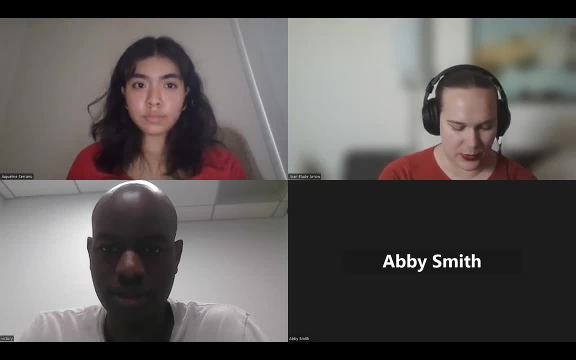 internships at quantum companies is the internships at quantum companies is the overarching objective of my program. so, overarching objective of my program, so overarching objective of my program, so um having these connections and working um having these connections and working um having these connections and working on projects like these, i think are 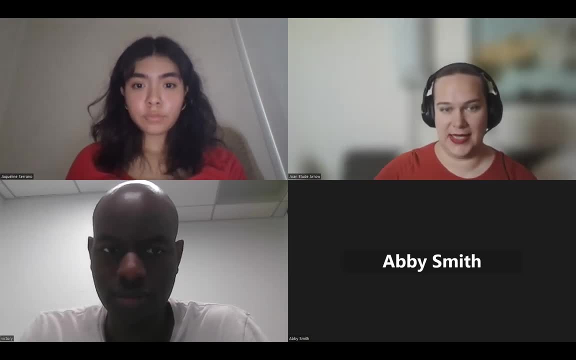 on projects like these, i think are. on projects like these, i think are is really valuable, even if a solution is really valuable, even if a solution is really valuable, even if a solution isn't found in the time limit we've set. so both of you talk to and reach out.